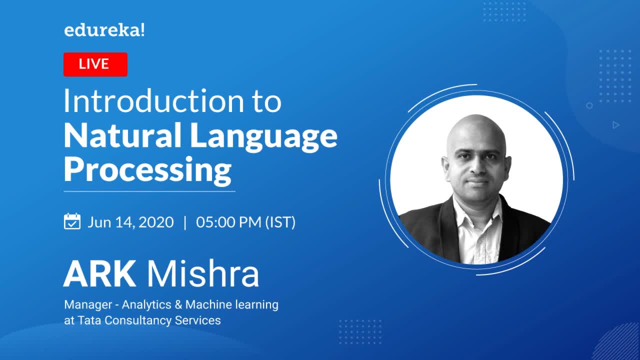 with new Sigma, then Microsoft And then Excel City, American Express, PCS. I mean these organizations and clients I have worked with, and right now I'm working as a project manager with ECS and I basically lead a team of people where we deliver projects related to NLP, artificial intelligence, deep. 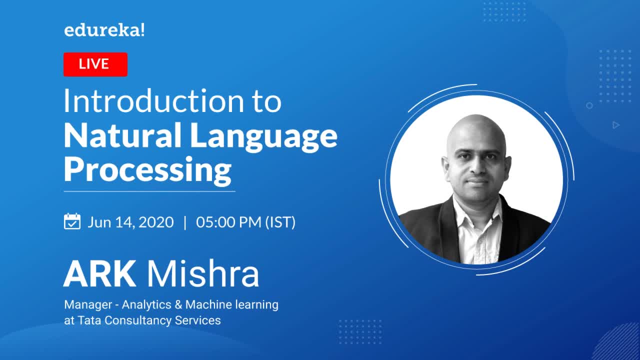 learning, machine learning and all so and mainly the tools and technique which we use is python, tensorflow, tensor, RT and R And Different statistical machine learning algorithms tool. So this was all about my corporate experience, but apparently I'm also involved in into lot of training and teaching activities. 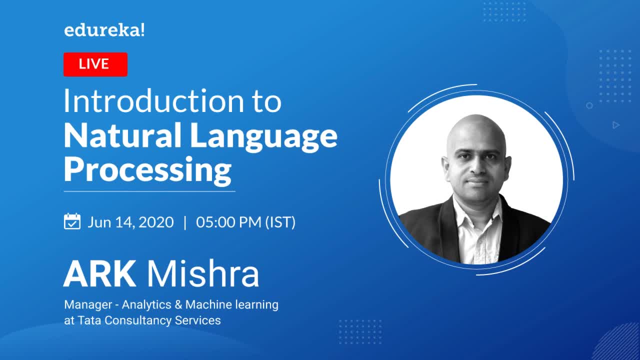 So, if I talk about my parallel teaching and training activities, I have almost 10 to 12 years of experience. So, and also the one of the best thing which I really like to do is I am the faculty of a statistics at bits Pilani. 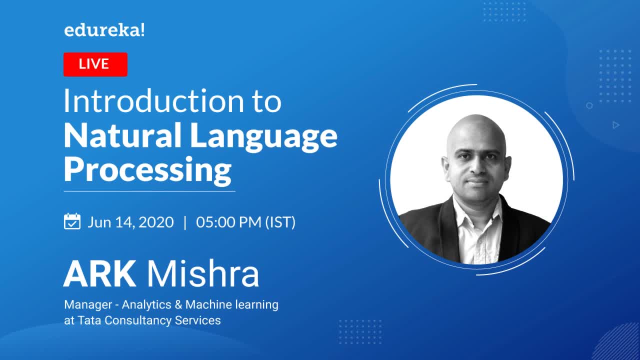 So which Pilani, is again one of the most reputed institutes in India for technical learning, For technical technology and science studies. so not only teaching, but I am the course content designer and then not starting the course content, then designing the content, finalizing the content to teaching examinations and then evaluation everything. 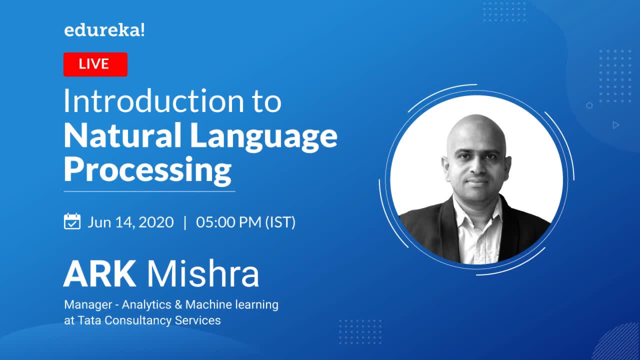 So I'm involved there and I teach one subject that is called statistics. So that is basically one program which happens on weekends, So I take that. So So that's about me guys, about my corporate experience, about my teaching experience, So let's not spend much time here. topic today is a natural language processing introduction. 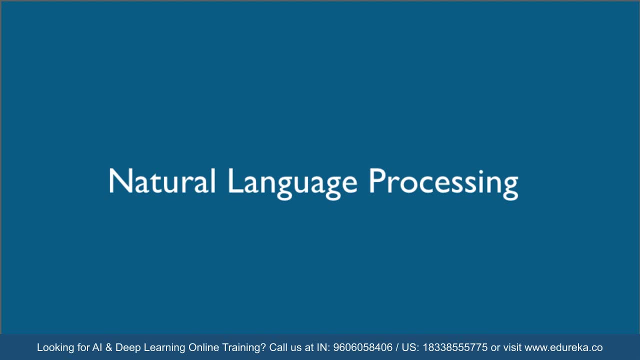 What is natural language processing? that comes to our mind and basically natural language processing is made of mainly two words, which is first is called natural language and second is called processing. So natural language is any language which is communicated between, mainly to human beings. It 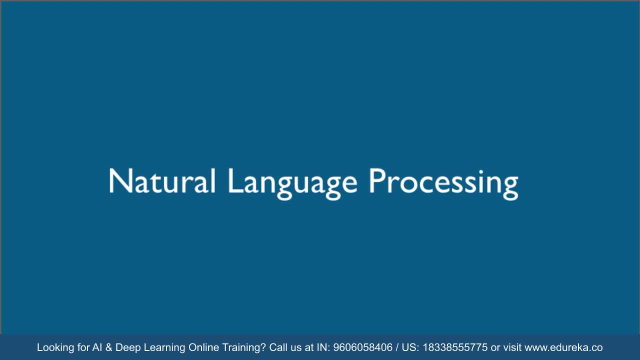 It may be method of voice or medium, maybe a voice or a speech. It may be a written chat. It may be on WhatsApp. It may be on Facebook. Maybe it may be a tweet. It may be a written document. It may be a letter. 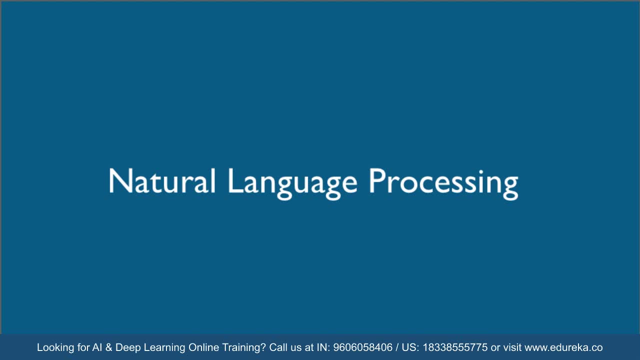 It may be a PDF file, It may be any notes which I make on a piece of paper and pen, so it can be anything. So any natural way of communicating is basically natural language, right? So if I'm talking to you here, so I'm using an English language to communicate. 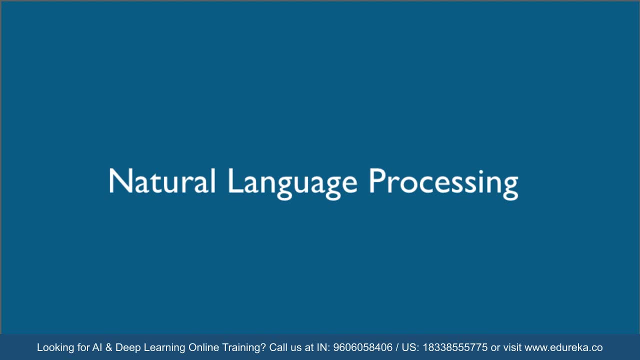 To you now what I am speaking. you are clearly able to understand it. why? because there is a dictionary. So I am basically following all the words, I'm taking all the words from the English dictionary and I'm using the semantics, the grammar of English dictionary. and that has been and the same thing. you have been trend. 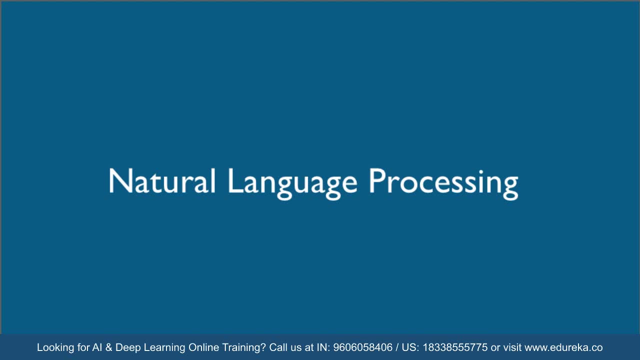 for you know English, you know the dictionary words, you know the grammar of English. So when I speak, your brain receives it and analyzes it and then understands, interpretates That what I'm speaking and what. the exact same meaning, or almost the exact same meaning. 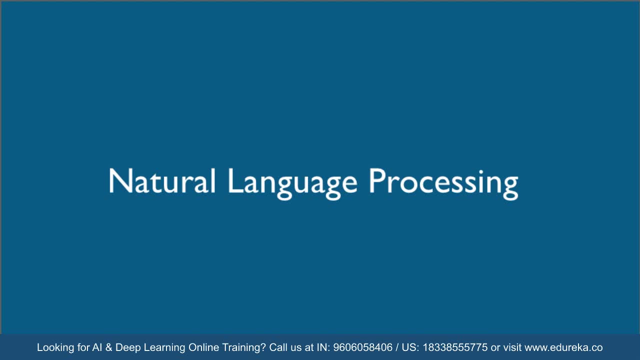 you are able to listen and then analyze and then interpret. So that is natural language. any form of medium you can say, or language which is naturally generated, like speech, like text in which to human beings generally talk, is called natural language. So there are two types of languages, guys. 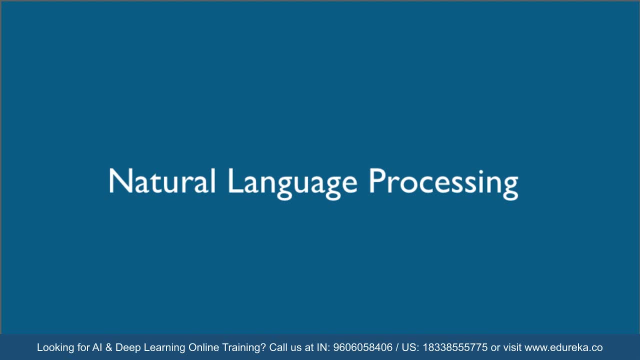 You already know, is money machine language. So machine language is the language where to compute, Computers talk to each other. So, for example, you have a computer, you have a laptop and you are chatting to somebody sitting at some other country, right? So if you write, how are you? so does the computer send exactly the same message to the next. 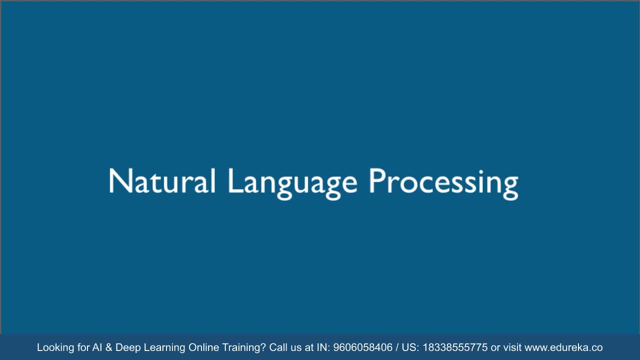 computer- maybe to your friend who is sitting in us know- it basically converts it into bits and bytes 0 and 1, and then it, the same message, is sent to your friend and then it is decoded. So that is not natural language, That is a machine language. 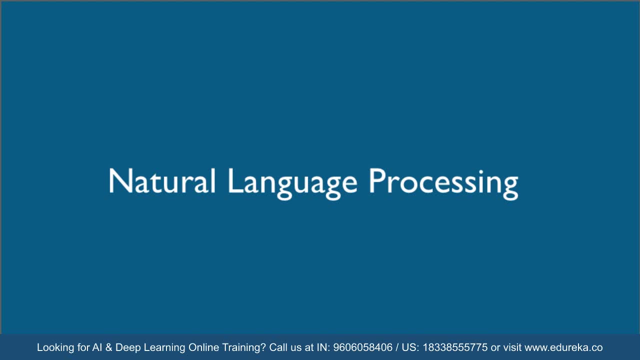 So when a machine talks to a machine, that is called machine language, and then when a human being talks to a human being, that is called a natural language. and natural language processing is basically one of the signs or one of the technique to understand and interpret the natural language by a machine. 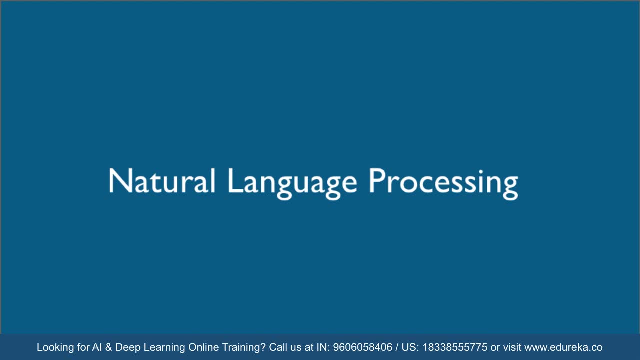 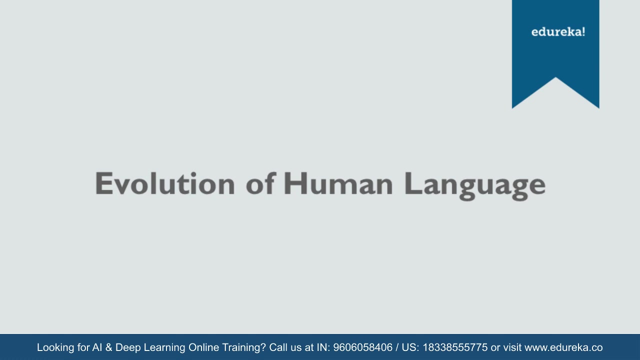 So when a machine, a computer, is able to understand and interpret and analyze and regenerate the language What you are talking to, then that process is called natural language processing. So everything as I talked about, everything is basically related to human language. Now, evolution of human language, guys. 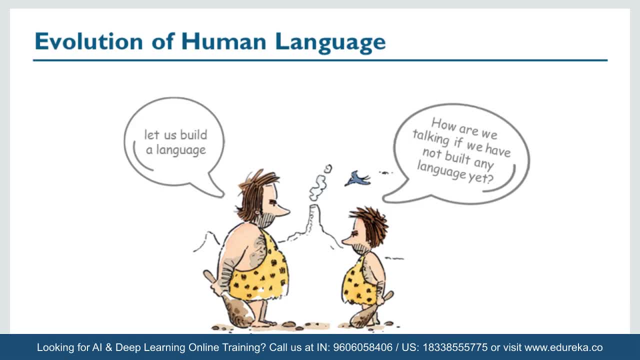 This has a big history. So initially, if we talk about, like thousands of years ago, how people used to communicate to each other, Maybe it was some symbolic movement of their hand, maybe symbolic movement of their body, Maybe some facial expressions, or maybe a combination of spatial expressions and some. 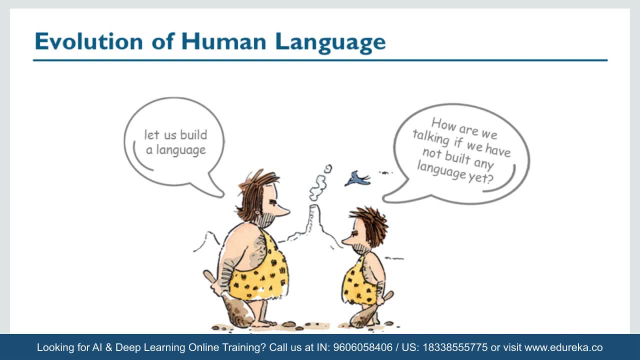 movement of their hand or maybe bodily movement. So that was the process with which people used to communicate to each other. Now it changed with time and people thought that there should be some way of communicating so that it's better, we can do it in a better manner. 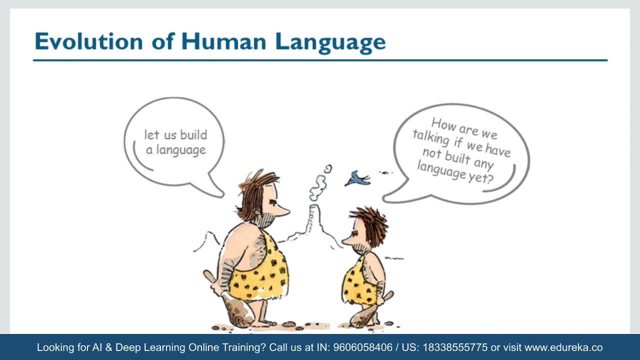 Basically languages were developed And then languages was so, for example, you give some symbol to a fruit- apple- and that apple, that symbol, is maintained homogeneously over a country or a state or maybe a group of people. then that becomes a standard language. And if you give a particular symbolic voice to a fruit, for example apple, the name of apple. 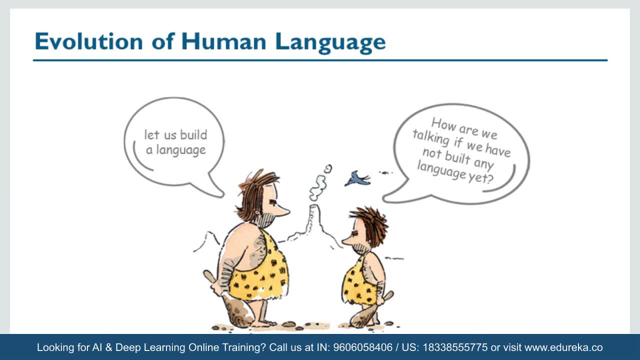 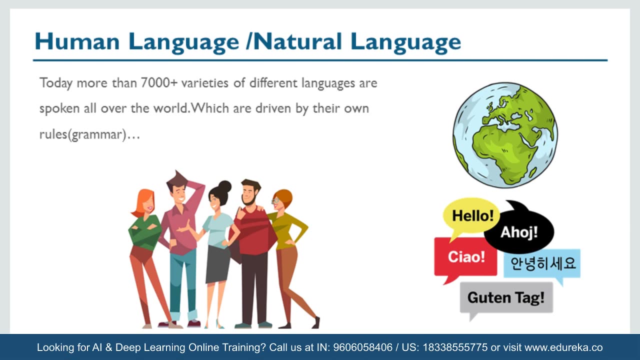 is apple. basically it becomes basic unit of a language. So this is how The language was generated and then human basically started communicating to each other with the language, Initially when there was no language. and then again you can understand that gesture and posture was a method of human language. but right now, when we have developed different 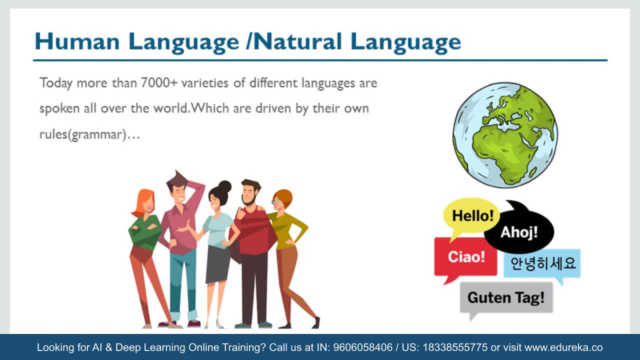 languages which we can speak, and which we can write and which we can convey, then the natural language basically does not contain that gesture. So now, guys, If I talk about the overall number of languages which are being talked or spoken over the globe, So we have even more than 7000 different languages which is spoken all over the world. 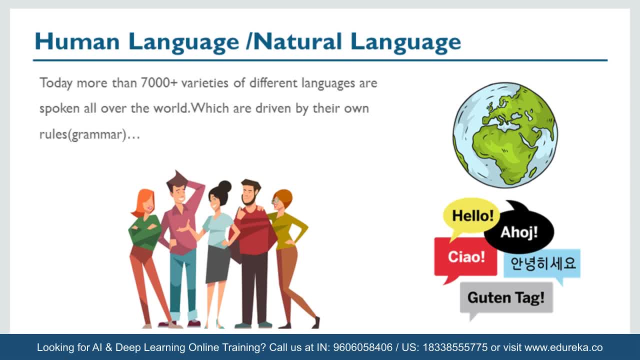 Now this is a big variety of languages you have, guys, but again, that is one of the challenges. Now, why it is a challenge? because a machine, because you want to analyze the human language by a computer. you want to make it automated When a computer 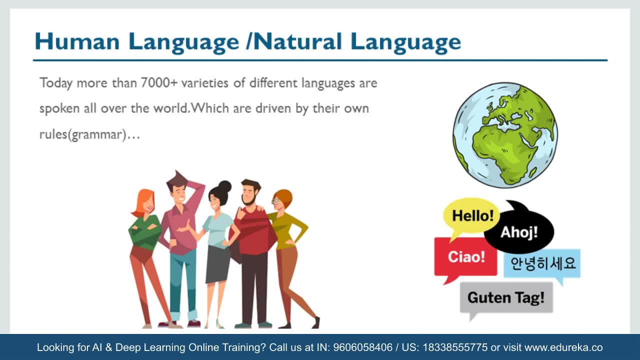 Or a laptop or a program or a model, just takes the data which you have written on Facebook, maybe all the historical posts which you have kept on Twitter. or maybe it wants to take all the posts or tweets from Bill Gates done on Twitter and then it wants to analyze whether 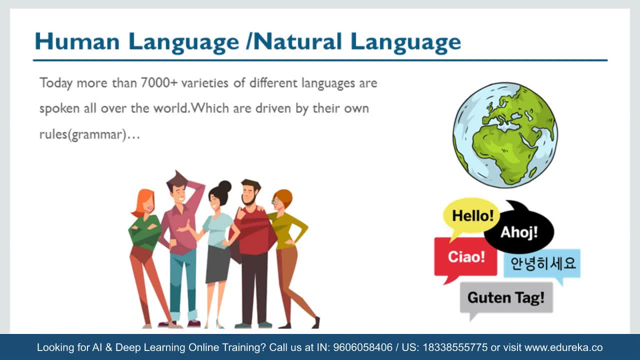 Bill Gates is a good person, which is basically contributing towards the community development, or not? Maybe you want to take all the tweets. may be done by Mr Narendra Modi, And then you can take all the tweets and then you can analyze whether he is contributing. 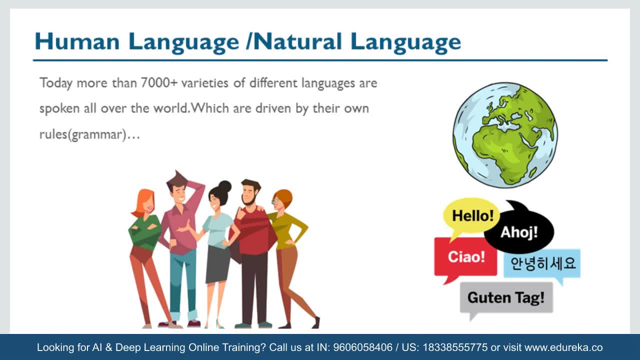 towards the positive growth of society or not. So this kind of analysis if you want to do manually, it will take a lot of energy, a lot of time and it will be hard for a human being to analyze almost, if I say, 1 million tweets. 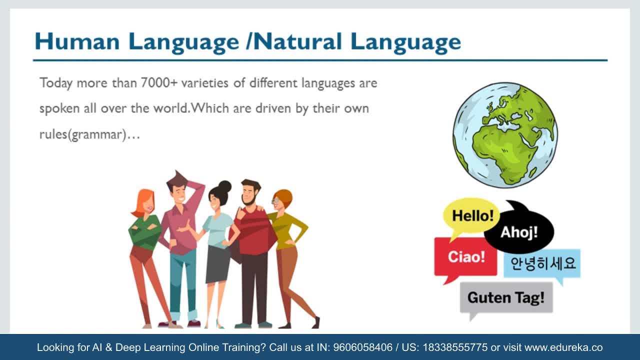 So that will be difficult. That's why you want a computer or a program or a lab or basically a model to understand and analyze all the tweets. But when the tweets are in 7,000 different languages, when the data comes to you in 7,000, 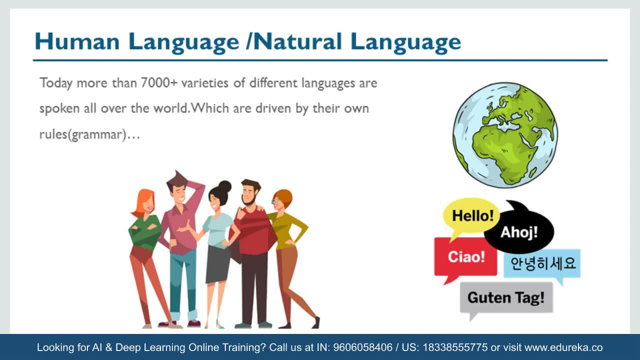 different languages, that becomes really a challenge. So, guys, this is again. the variety of languages is present on over the globe is again one of the benefits. I mean this is kind of variety we have, but again, for natural language processing This is a kind of challenge as well. 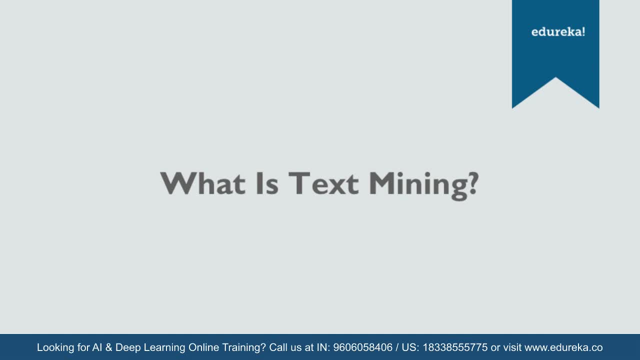 What is text mining, natural language processing, guys, if I tell you in one nutshell, Nutshell definition, It is basically writing a program, developing a model, developing a deep learning model or developing artificial intelligence logic which takes input, which takes your natural language- It may be text- and then analyze it, interpret it and then give you insights. 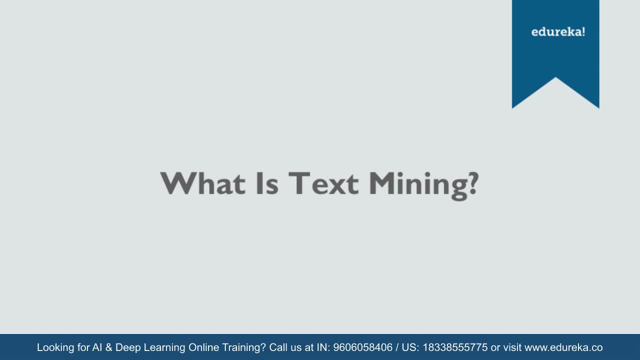 So that is called natural language processing. So process your natural language and specially if I talk about the data, kind of data which we are receiving nowadays is the text data. the voice data is not that much the video data, I mean it's not that much- but the biggest type of data which is being generated nowadays. 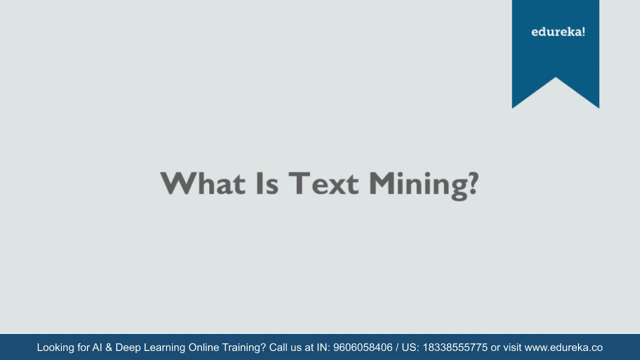 is the text data, For example, if I talk about WhatsApp, so you are basically almost everybody is spending at least one hour on WhatsApp, Maybe giving some information, chatting to your friend, talking something professionally, or maybe on Twitter, You type a tweet Or maybe best example. 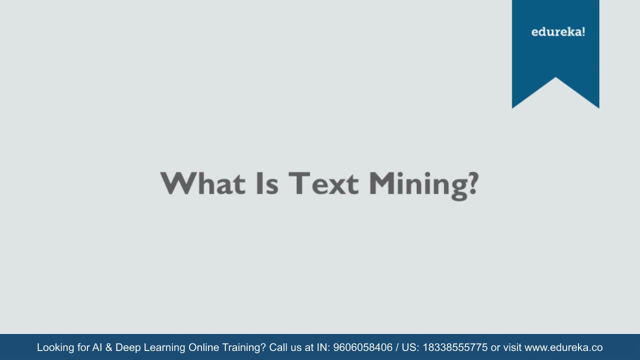 I would say that you are writing emails. So when you write emails to your friend, to your boss, to your colleague, to your organization, you are generating some text data, and so this is the highest quantity of data which is being produced over the globe. that is a text data, and that is the reason, guys, we need to understand. 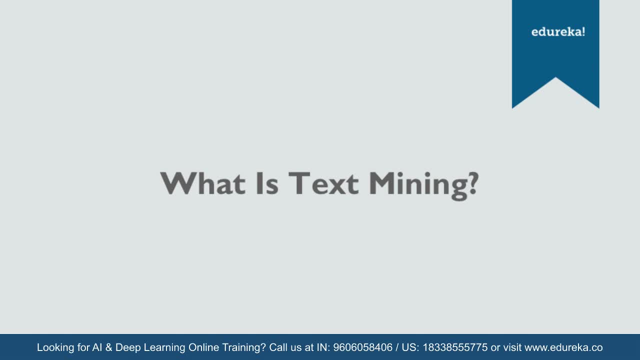 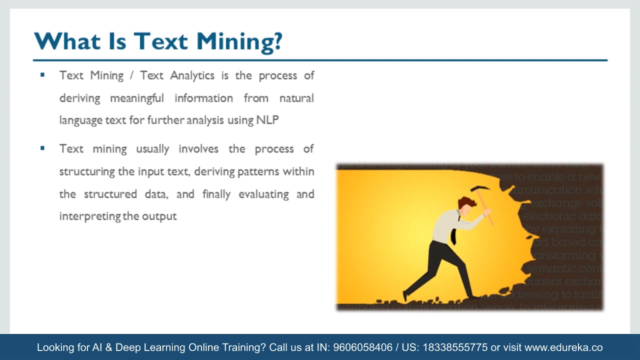 and we need to study, and we need to develop this text mining or NLP process, where we can take text data as input and we can draw a lot of beautiful insights from it. So if I want to explain you what is text analytics, guys? so it is nothing but similar to data. 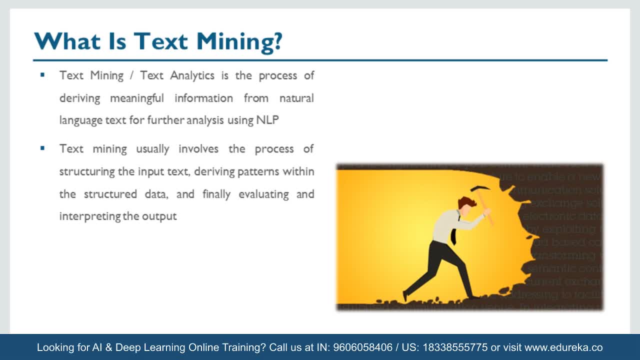 analysis where you take the- I mean a structured data. you take a structured data, you make some analysis like, for example, you do the missing value treatment, you do the treatment. then you basically see the basic statistics like the mean median mode, standard deviation on maybe variance. 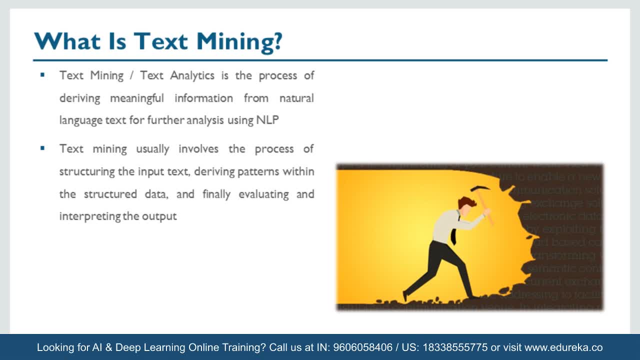 Then you do some hypothesis testing, then you do some regression thing, then you do some time series forecasting or you some do some linear regression or logistic regression, a lot of different analysis you do, and then you come up with some prediction or maybe you come with come up with some good insights about the data. in the same way, guys, if you 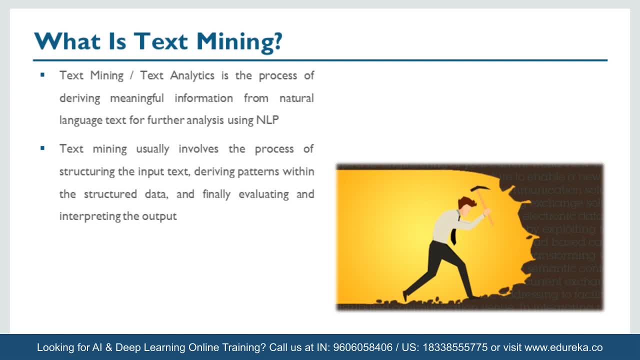 are working on some text data rather than a structured data, So that thing is called text mining. So what you do in text mining is basically you take text data- or you can say On a structured data- as an input and you process it to basically derive patterns and 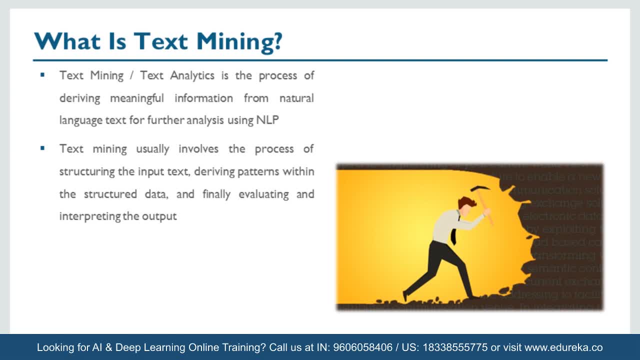 to derive beautiful insights, to do some forecasting, to do some clustering, to do some classification and a lot of things you can do now. generally, there is a confusion here between people say what is structured data and what is unstructured data. why are you calling text data as an unstructured? 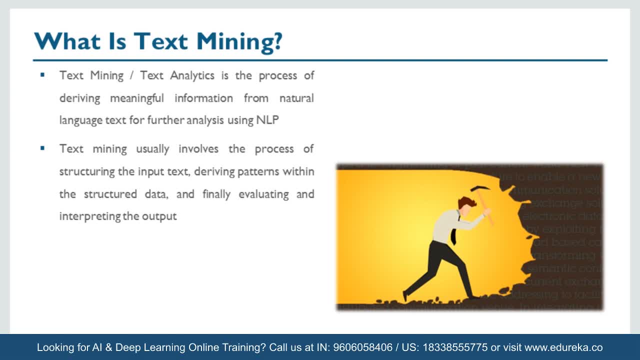 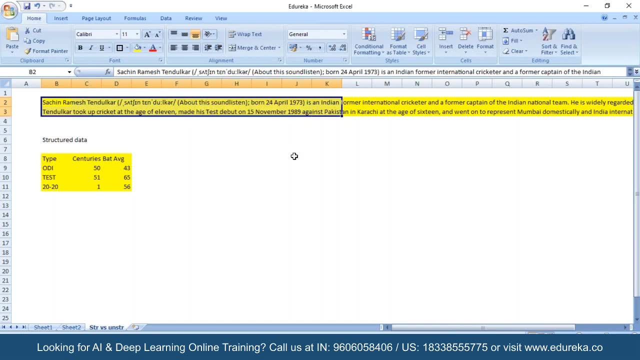 data. So, guys, I would give you an example of a structured and unstructured data, For example, if you see this data here. this is some couple of lines which have been taken from the Wikipedia page of Mr Sachin Tendulkar. 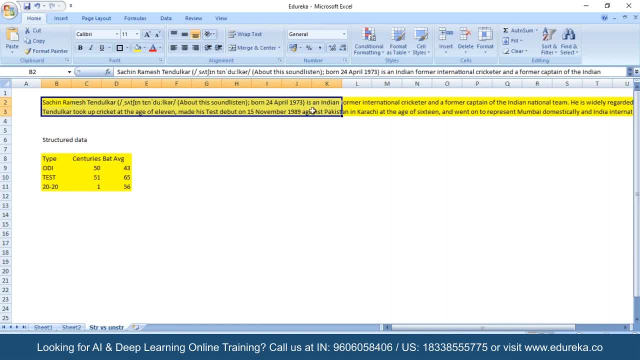 So this is a unstructured data, guys, This is the kind of text which has been written here, right, but how does that structure data look like about Sachin Tendulkar? So when I make it a structured data, when I process it, and when I make it a structured 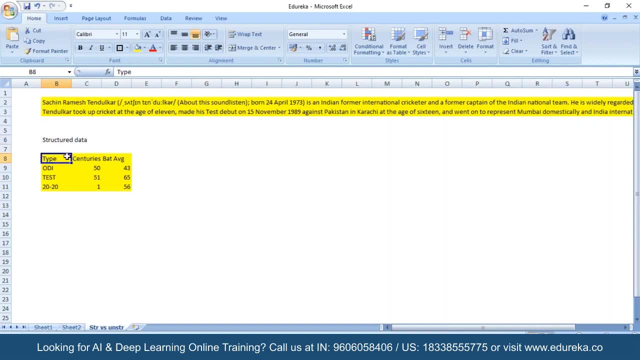 data. it will be like three columns where first column is the type, second column is the century, is number of centuries, and third column is the batting average. Now, if you see, the type is ODI, test and 2020 format, or the type of games which he has played. 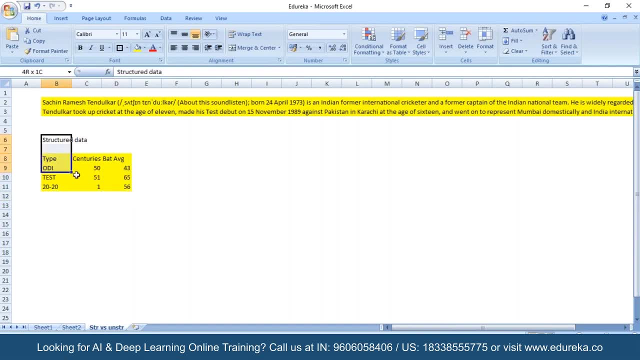 then number of centuries and then the batting average. So, guys, this is structured data, right, and this is on a structured data. Now, the irony is that structured data is easy to interpret, is easy to understand, is easy to summarize, is easy to analyze, but on a structured data, on the contrary, is not that easy. 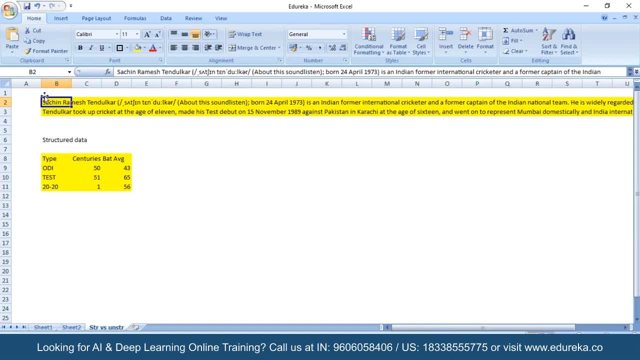 So, basically, the text data or the unstructured data needs some kind of processing, and to make it readable, to make it more structured, to make it in a format where you can apply some machine learning or deep learning or artificial algorithms on that, you need to process it and that is the reason, guys, we call it natural language processing, making. 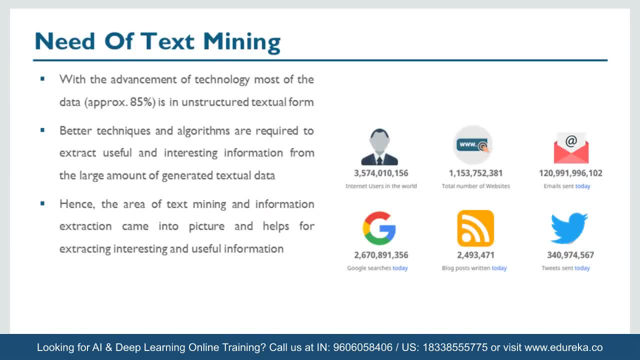 unstructured data into a structured format, and again talking about the amount of data, especially the text data, which is getting produced over the globe. So if I say that, almost, and guys, there is one very good, interesting thing which I wanted to talk about. So, basically, have you seen that this data analysis and machine learning, deep learning, 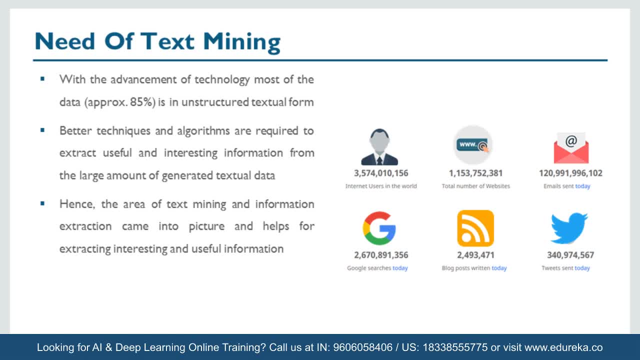 artificial intelligence have taken growth in last eight to ten years. Now, what is the factor which has changed all these things Now, why you are here listening to this session and why I'm here Delivering this session, why any data is formed, why there are other institutes of which are? 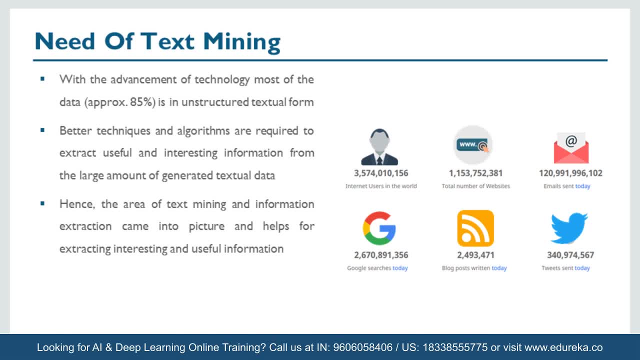 teaching analytics and data science and why machine learning is is on so high. and then why artificial intelligence is so popular, why deep learning so popular, by data analytics or so? Eight to ten years ago there was no discussion but most hype into data science and what had. 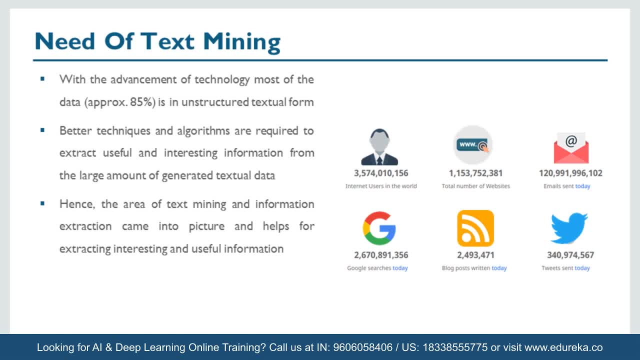 changed the complete scene. the scene which has completely changed is the factor is basically the amount of data getting generated. So, if you remember, like eight, ten years ago, there was very limited number of phones. There was no smart TV, no smart houses. your washing machine was a very normal washing. 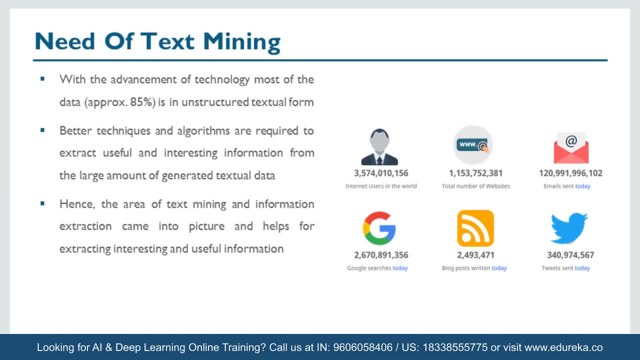 machine and after eight to ten years, when communication revolution came into the picture, when Internet came into the picture then, and when Internet of Things came into the picture- but smartphones came into the picture and a smart TVs came into the picture- lot of data started, They generated. Orkut came, then Facebook, then WhatsApp and a lot of different platforms. 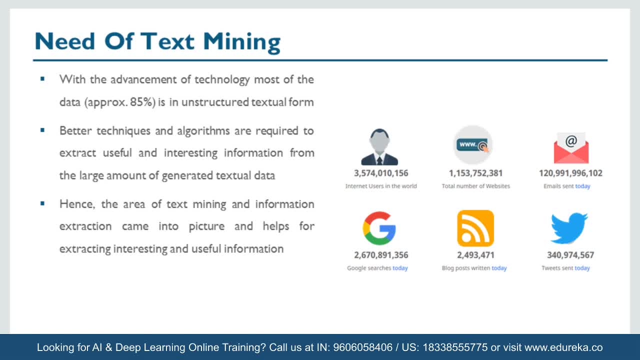 are there now. your TV is smart TV disconnected to Internet. your washing machine is a smart washing machine. It is connected to the Internet. your phone is connected to the Internet. your laptop is connected to the Internet. You are connected to the Internet. everything your house is connected to the Internet, right? 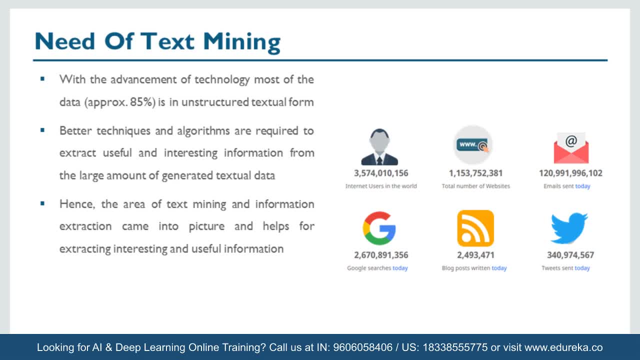 So, whatever you are doing, you are producing data, and now, when you are producing such a huge kind of data, huge amount of data, now, data contains information, Right? So data is basically raw form of information. You do some analysis, You apply some algorithm and then you get machine learning. you apply some machine learning. 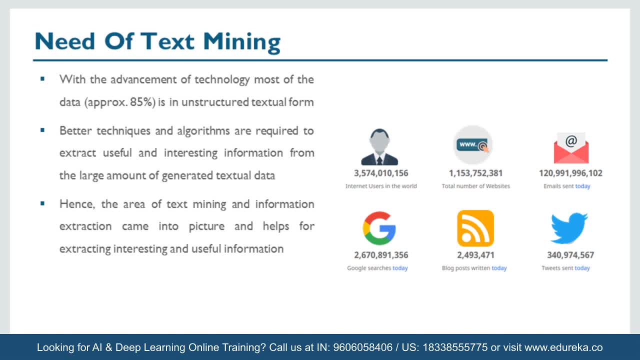 or maybe some simple algorithm and you get some insights. you can see what is going to happen in future with the help of the historical data. So that is the reason guys Hype into machine learning, deep learning and artificial intelligence game just because the amount of data is being generated in since last eight, ten years and 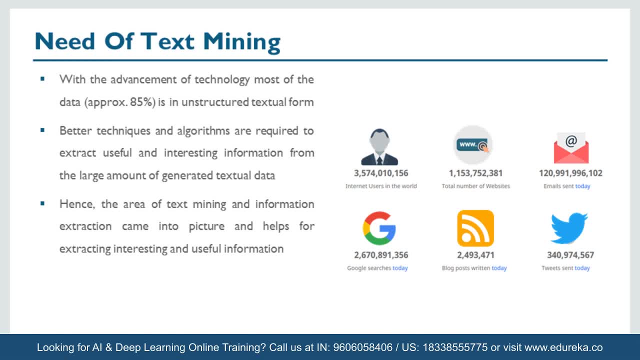 this is the reason and let me tell you that the, the amount, the whole amount of data which I talked about, Is it the structured data or is it on a structured data? Is it the voice data? Is it the video data? Is it the text data? 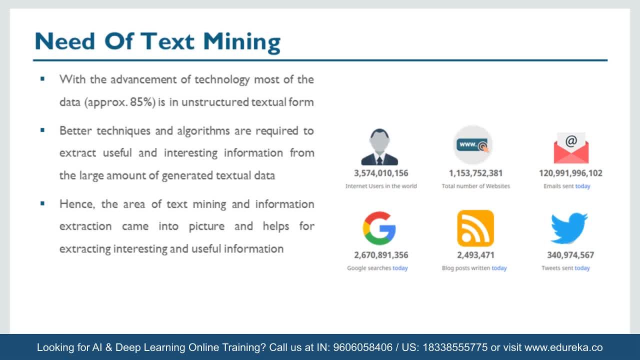 So, guys, let me tell you that almost 85% of the data which is getting generated day by day in the modern world is basically unstructured textual form, where you are either writing some blog, or you are writing a tweet, or you are writing some Google search. 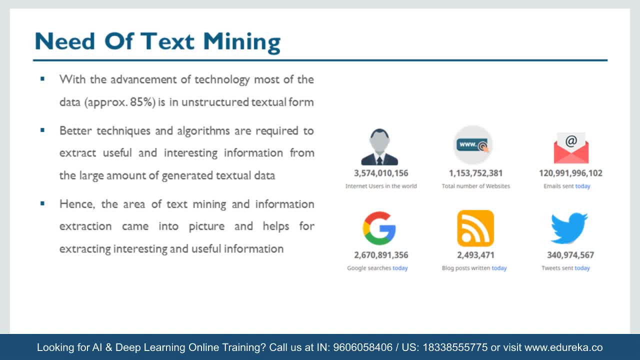 You are doing some Google search, you are writing some emails, You are you are browsing some website. So these are the very interesting figure, guys, where 300 crore internet users are there, 100 crore websites are there, 200 crores emails are being written on daily basis. 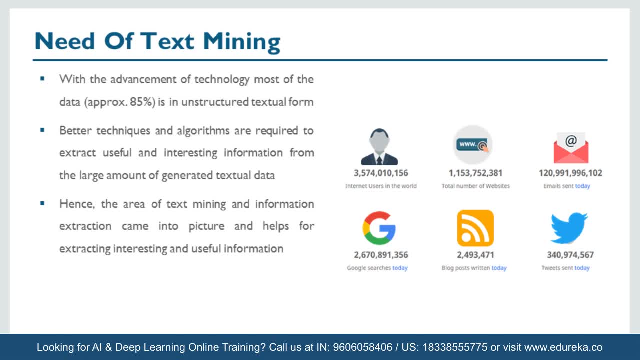 200 crores of Google search. basically people are doing on daily basis. 20 lakhs blog posts are written daily and in the same way, there are a lot of tweets. They are being written on daily basis. Now can you imagine the amount of data. 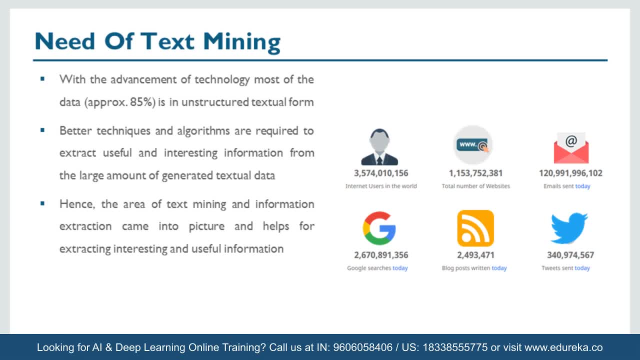 which is being produced in textual format. now, guys, let me tell you again a very interesting case: that generally what happens is when election comes in India- or maybe election comes in any country, Let's talk about India- when election comes very near, people become very active on Twitter, people become very active. 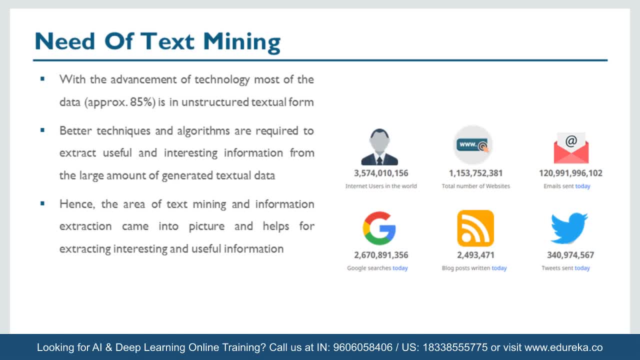 on social media. our politicians become very active and Twitter and Facebook. this becomes a very hot Medium to spread maybe some rumors, maybe information and lot of things. Now, if you are not talking to your friends, if you are spending more time on Twitter rather than talking to a community, 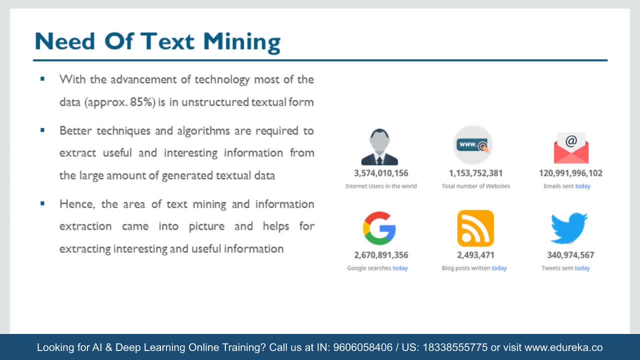 rather than talking to your friends and you are expressing your sentiments on Twitter. can dive take all the Twitter tweets of maybe 1 million people or 2 million people and then analyzing the tweets, or see that what is the frequent word people are using. So, guys, this is just an example. 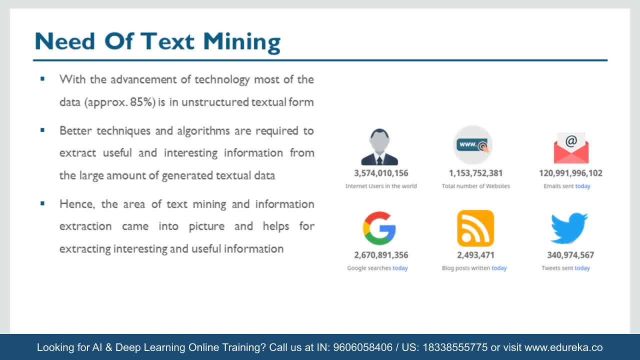 And this example is called sentiment analysis. Let me give you another example. Everybody knows here IMDB, internet movie databases. So at IMDB, basically, if you can see that lot of users are there, even who watch a movie, then write a review, So lot of reviews are positive. now suppose there is a movie. 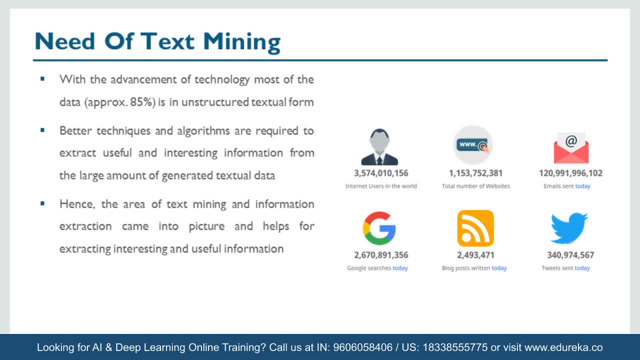 which is called sauce and Redemption or maybe the latest movie. So maybe I would like that movie and maybe some person here may not like that movie. So that depends on choice to choice, person-to-person. now, overall movie reviews are positive or not, So that we can analyze by taking all the reviews individually. 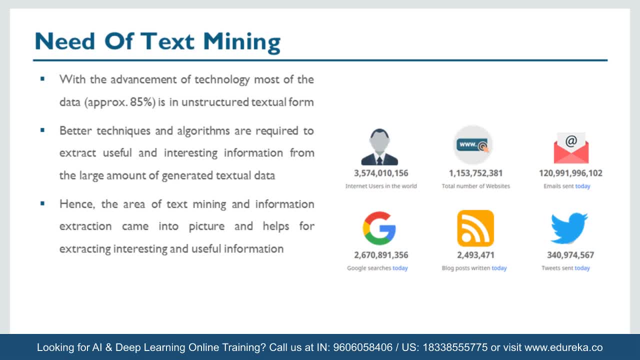 and seeing at the world like which word they are using: awesome, Great word, good acting, This is historical, This is awesome or maybe waste of time, money wasted. So these kind of reviews are there So you can go through the reviews, You can fetch the reviews. 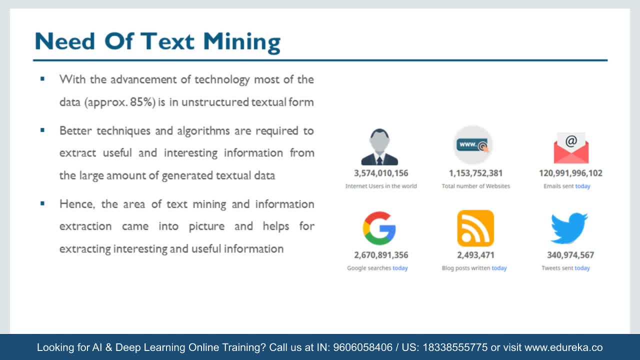 You can analyze the words and then you can analyze the sentiment of the user and then you can see whether this movie is going to do business, good business or not. Is this movie is going to be a flop movie on box office or is this movie is doing good on box office? 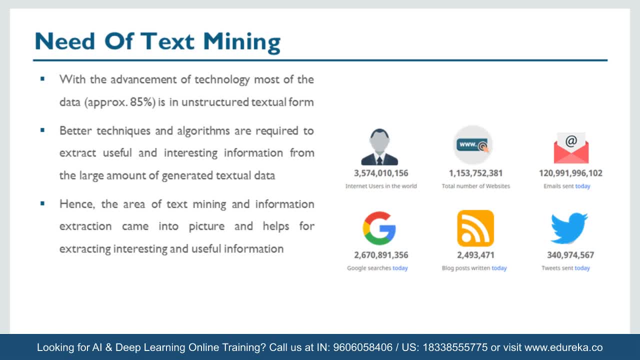 So everything you can predict is the customer sentiment going upwards or is the customer sentiment going down downwards day by day. So there are a lot of different examples on NLP which I can give you. So and that is due to the amount of data which is being produced. 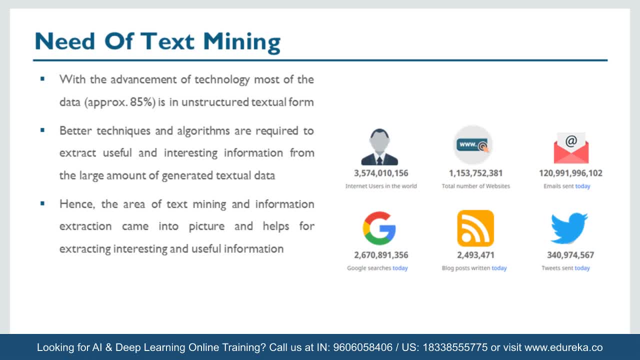 and if you think that the amount of data is the huge amount of data, text data which is getting produced, are we able to capture everyone, all the data, most of the data? Yes. are we able to analyze and interpret all the data? Absolutely. 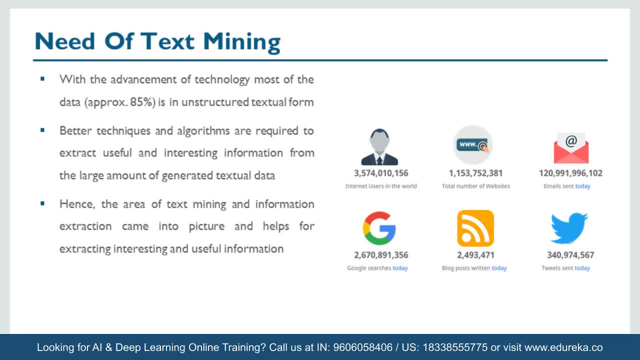 No, are we able to use those data into any machine learning algorithm to get insights? know, or have you set up a process where we can use, Use all the data which is being produced and using any deep learning or artificial intelligence so that we can get some good insights or making? 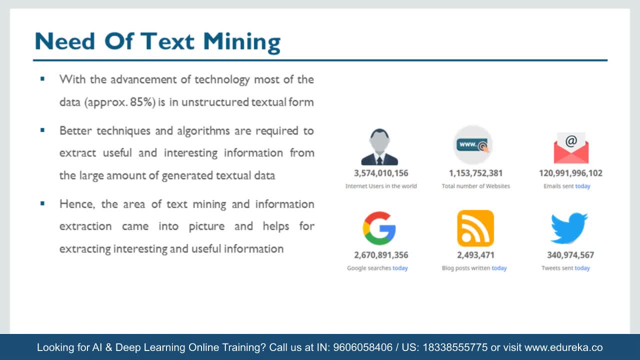 maybe we can do some predictions. Absolutely No. Now, what is the reason? the reason is two things. first, text data is hard to process. second thing: lack of expert people or lack of people into this expertise domain. third thing: heavy chances. lot of chances are there for improvement of existing 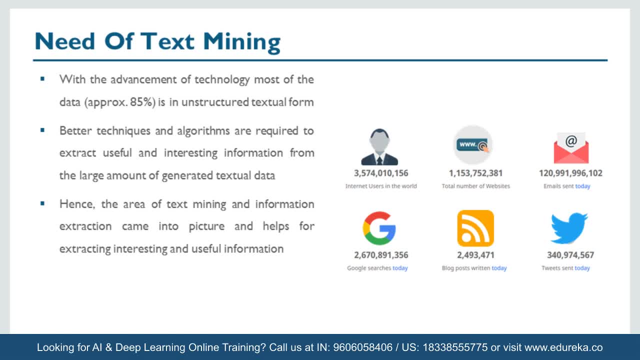 algorithms. the existing algorithm, the deep learning artificial intelligence algorithms, are doing quite good, but there's a great chance of improvement of research into natural language processing or maybe text mining. So, guys, this is the reason there is a huge demand and huge scope of research to huge scope of work and huge scope of skilled people. 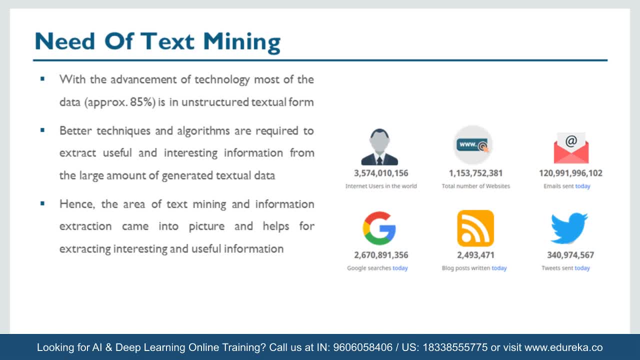 into Natural language processing. So, because you can see that the amount of data which is being produced is huge, but we are not able to use it, We are not able to make a useful derivation out of it. Now, what is NLP? 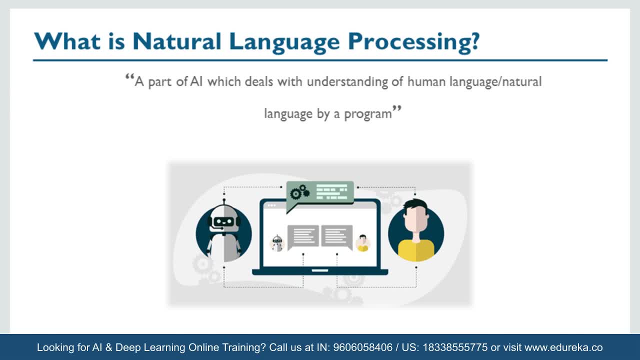 NLP is a process where you take natural language- It may be speech, It may be textual data- and you basically try to analyze or interpret or generate or understand that natural language With the help of a program, a computer, a model, a mathematical equation. 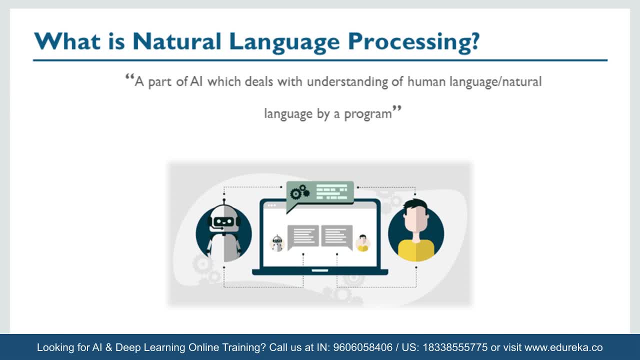 So this is a part of AI, is basically artificial intelligence. Basically, you deal with human language. It may be a voice language, It may be a text language, and then you make it interact with a program, you make it interact with a model, and then you get a good 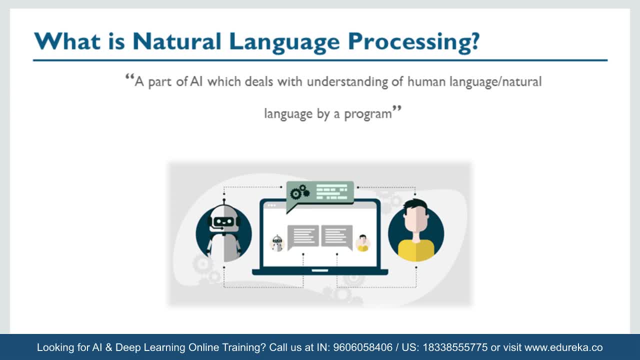 insight. Let me give you an example again. The IRCTC website has Launched a chat bot whose name is Disha. Now, at the end of the chat bot, when you write a query, do you think that there is a? there is a girl whose name is Disha and she is. 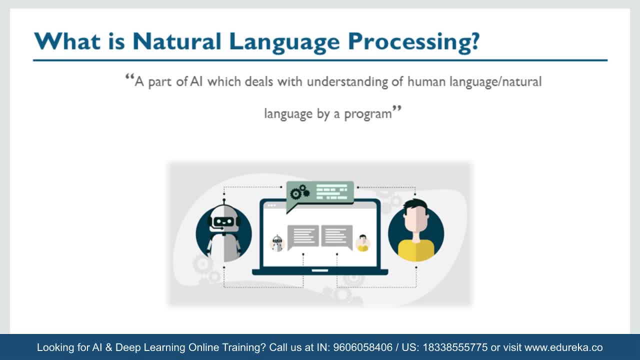 basically answering your questions? Not at all. This is nothing but a computer, a computer program who interacts with you when you write a question, a query: Can you tell me which train the number of trains from Delhi to Bombay? Now, this query Will be answered by a computer program or an artificial intelligence. 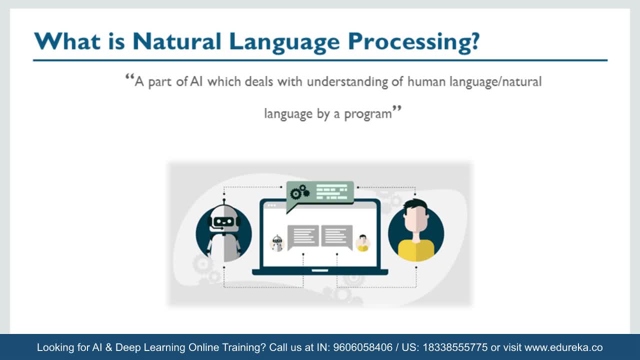 program. So, guys, this is how we define NLP, that this is a part of artificial intelligence where you deal with natural languages like voice or text data written by a human being and, on the basis of that data which you have received, you analyze, it interpreted and then maybe after that, 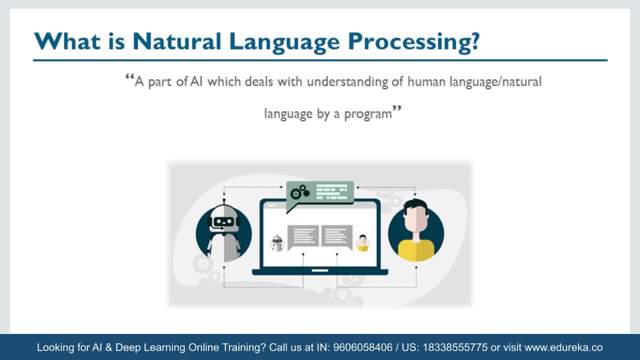 you take some action. Now what kind of action you can take? either you can Answer the question or you can do what he's saying. For example, Alexa Siri, Google assistant now in my house. If I go and ask Alexa- Alexa, please play a birthday song. 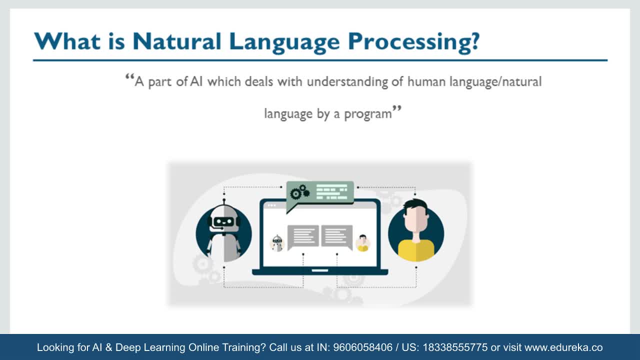 This is my daughter's birthday. Now how does this is being applied? Basically? you spoke some English words: Alexa, play a birthday song. First one is Alexa. second word is play a birthday song. Now this is listened by Alexa, So there is a microphone which receives your frequency audio. 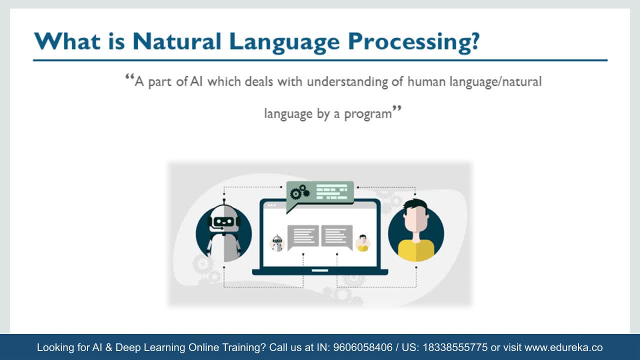 frequency. Then it is being converted to text data. Then, after converting to text data, Alexa takes it and understand what you want to do Now. Alexa will take the keywords birthday song. Maybe it will go to YouTube and it will write those keywords birthday. 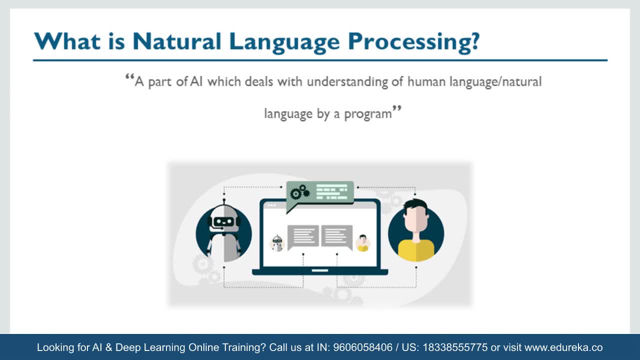 song and after that, the first link which comes to you, YouTube, it will play it. So this is how, guys, an artificial intelligence program basically works and basically analyzes the language which you are speaking, the language which you are writing, and then it in the response. 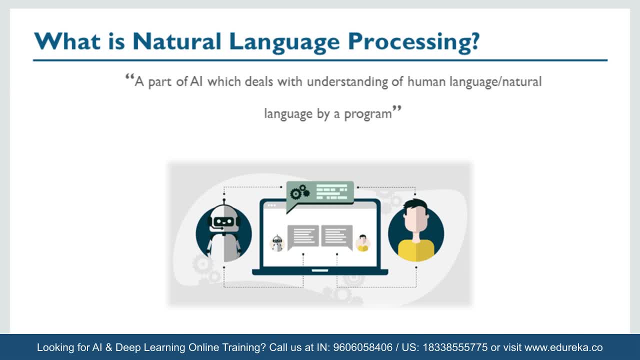 It may be an answer to your question. It may be the command which you have given that will be executed. So a lot of things are there which is being happening that is called NLP. Again, guys, if I talk about the historical Process or progress of NLP, 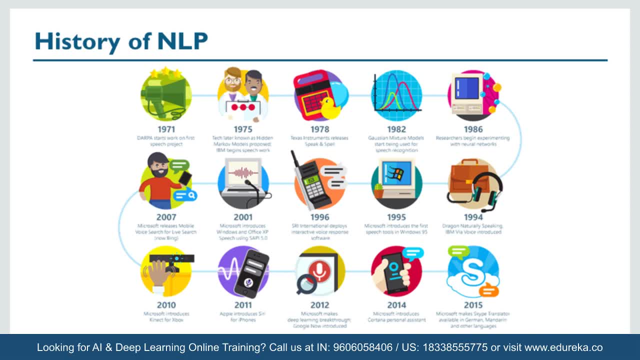 It has not taken just one day to reach this point where we have Alexa Siri and we have Google assistants in our houses, in our mobile phones, and we just ask them to do when they are doing everything. So if I ask Alistair to switch off my TV, it will do it. 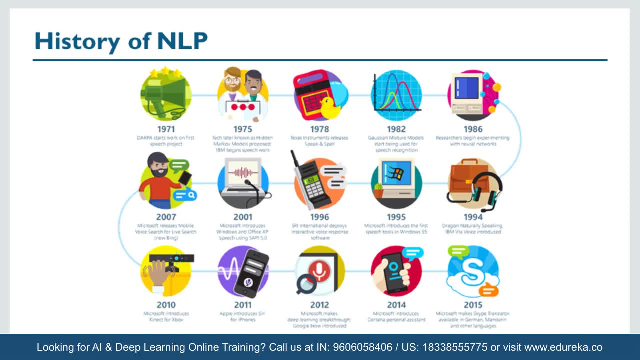 So this is not like we have done it in just one day. So if I talk about historically, it almost started into 97. One where Darpa Industries basically started on speech product. So after that basically some Marco models statistics were proposed by IBM, then Texas instruments again came up with a release of. 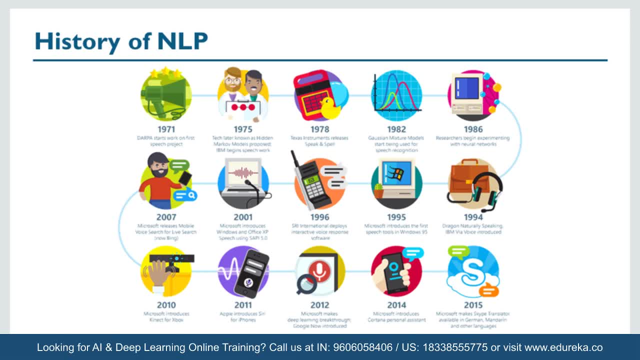 speak and spell. So basically, speak and spell was right. like you press or you write something, it will read it out then. So the growth has been taken like almost 30, 40 years to reach this point where we are today. So from touch and speak to speech, recognition to again speech to. 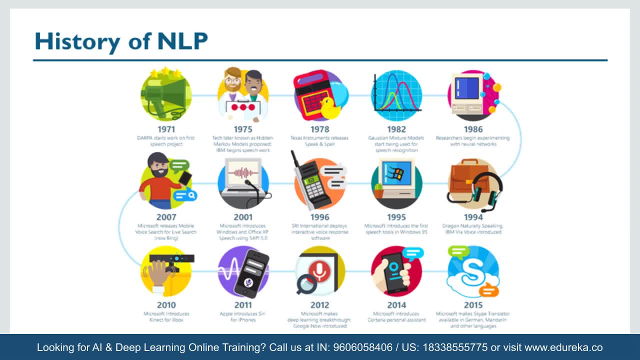 command, like Alexa, Siri, to IVRS and to Google assistant Alexa and Siri. It has taken almost 40 years to reach this point here. to be more specific, almost 50 years. So, guys, this is a progressive thing. So it is started with very basic research where people just wanted 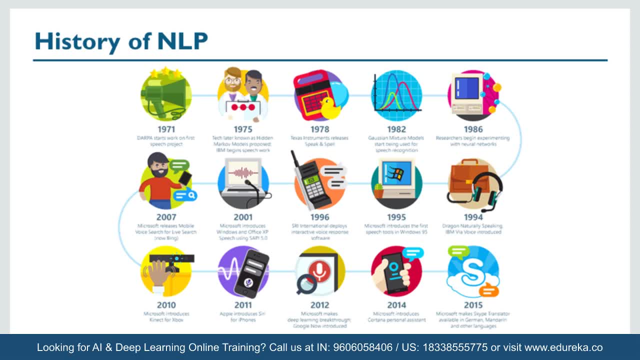 to see whether We can make a machine. we can just read out what is written in the text, and then it was done. then, after that, people start with that: Okay, can we create a program where it can listen to our voice and then it can respond to? that was again done. then again the approach. 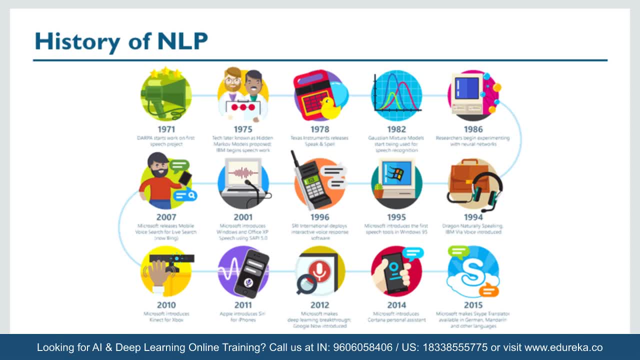 was. can we develop a program which can understand what I'm saying and which can also reply and can do some action regarding my query? For example, if I ask Alexa book a flight from Delhi to Bombay On 24th of June, So it will go to a particular website, type the query and see whether 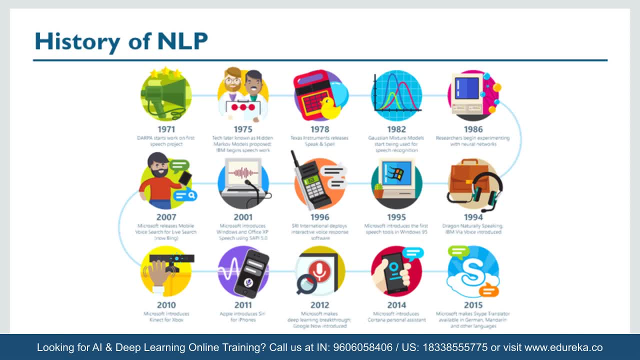 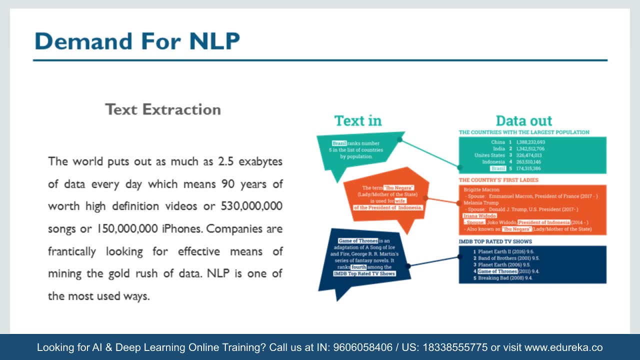 what? what are the prices available? So, guys, it has taken almost 40, 50 years to reach this point. what we are doing today, again, Why there is a demand for an LP in in terms of skilled people, and why there is a demand of NLP, if you talk about in organizations, why we 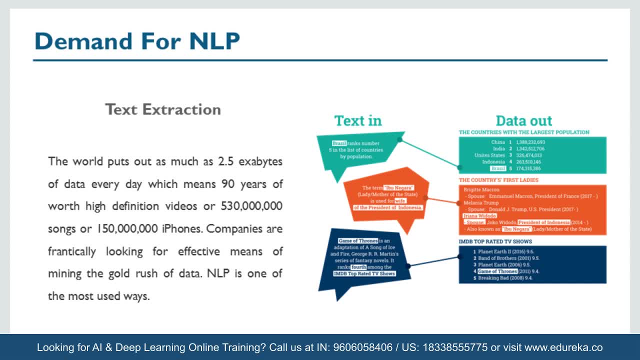 need an LP to do. that is most of the data which is coming. So, for example, each day we are basically having 2.5 exabytes of data. Now, what is the exabyte? exabyte is basically 1. exabyte is equal to. 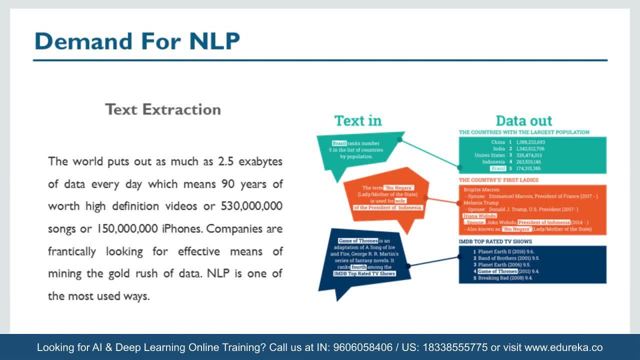 10 to the power, 10 GB of data. Let me repeat it: 10 to the power, 10 GB of the data. right, So this is exabyte. So it is almost equal to basically 90 years of worth high definition videos. 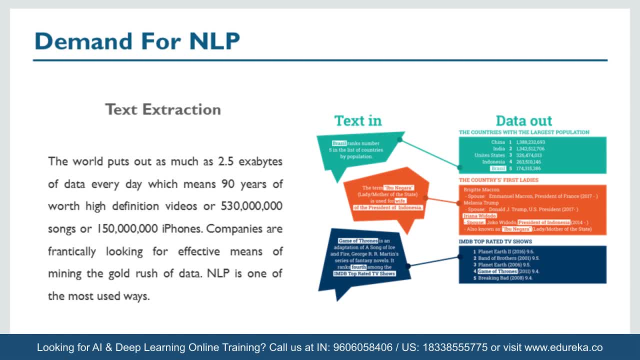 So if I take a video which is almost 90 years long, high definition video, That amount of memory we are consuming by producing text data on each day- Now you can just imagine that how much information is basically hidden besides, or the data which is being produced in a textual format. 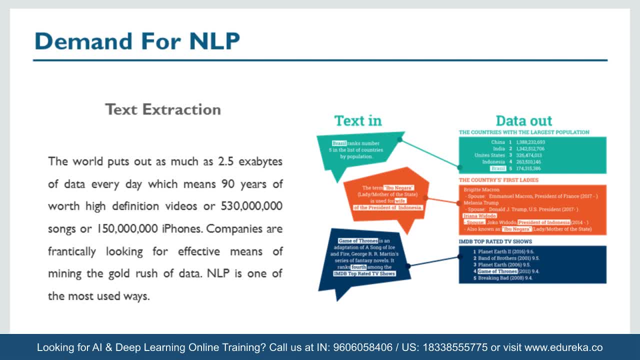 So the only thing which you need to do, as I told you, that text in is basically unstructured data, and you need to do some processing, because after that you need to make it without structured data. For example, if the text data says that Brazil ranks fifth in the list of countries, 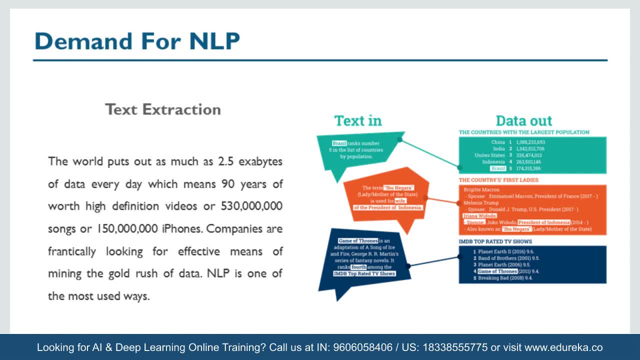 by population. maybe, with such kind of data, you want to create a list where the column a represents the name of the country and the column to represents the rank and the column 3 represents the population of the country. So this is how, basically, you need to process your data in order to make 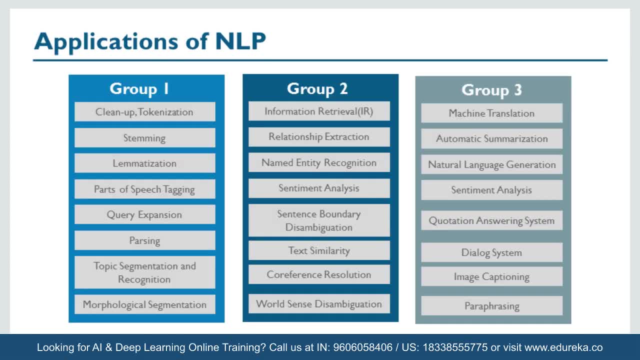 it more useful, make it more easy to analyze- now, if I talk about the main components of NLP or the main actions of NLP, what you do in NLP mainly, it is grouped into three groups on the basis of complexity of the task. So group 1 is easier to accomplish, are busy, very basic things then. 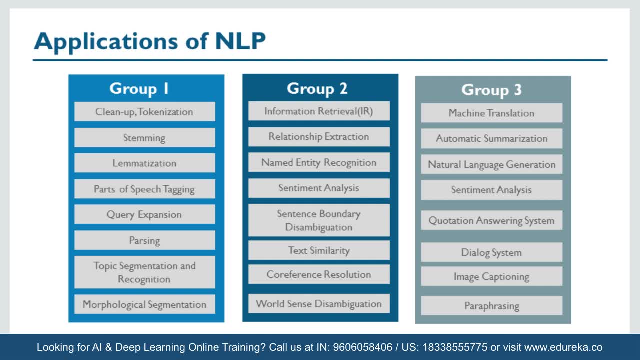 group 2 is basically little more complex as compared to group 1, and then group 3 is the most complex thing to do here. So, guys, now you will be wondering That, what are these things? so these are all the algorithms and these are all the processes which are present, with which you can do a lot of. 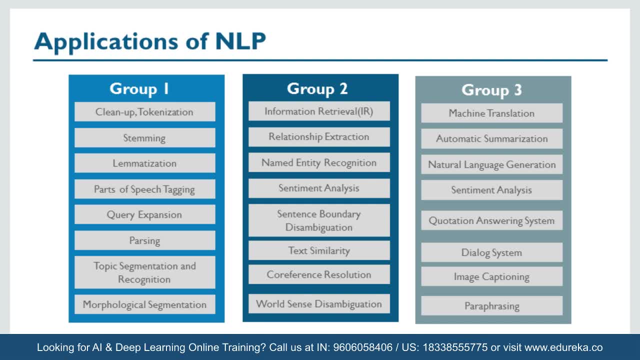 magic here. So, for example, let's talk about this first thing, which is clean up and tokenization. Now, what is clean up? clean up is basically removing the unwanted things from your data. For example, if you remember your whatsapp chat, you generally use a lot of smileys. 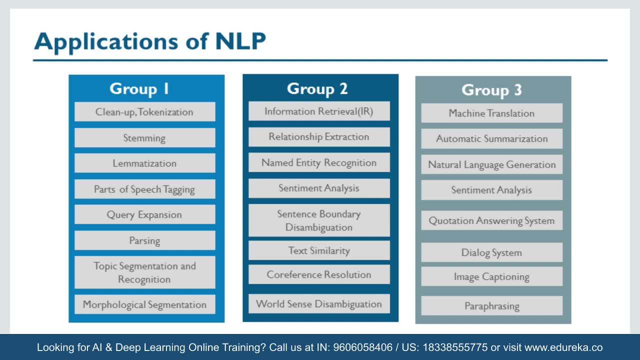 you generally use a lot of gifs or maybe smileys. So if I take your chat bot whatsapp data to analyze, I need to remove those smileys from there, right? or I need to remove some special characters which you are using. so that is called clean up. 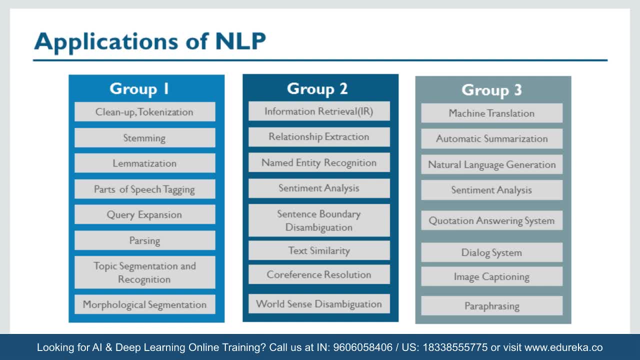 Now, what is tokenization? tokenization is nothing but taking your complete text data and breaking it into sentences or maybe breaking it into words. That is called clean up or tokenization. So again, let me give you an example here. So, for example, 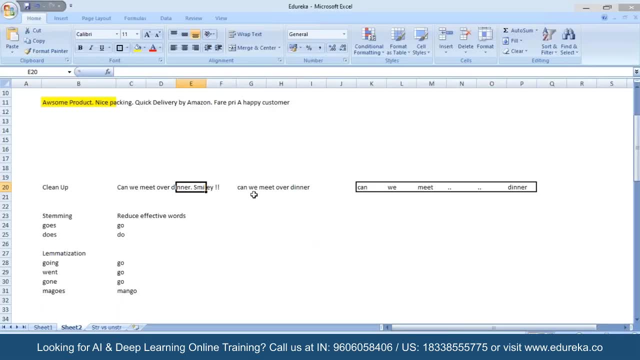 this is your chat, like: can we meet over dinner? and then smiley. So clean up means you need to remove that smiley and after cleaning up that smiley your sentence become: can we meet over dinner. Now what is tokenization? tokenization is basically breaking a sentence into. 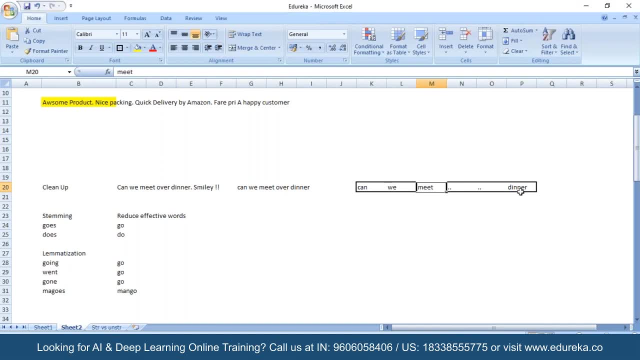 word like: can we meet over and dinner. So this is tokenization And why we are doing this, guys, because a text is made of sentences. a sentence is made of words and word and some special meanings. So what we want to do here is basically taking a text data. 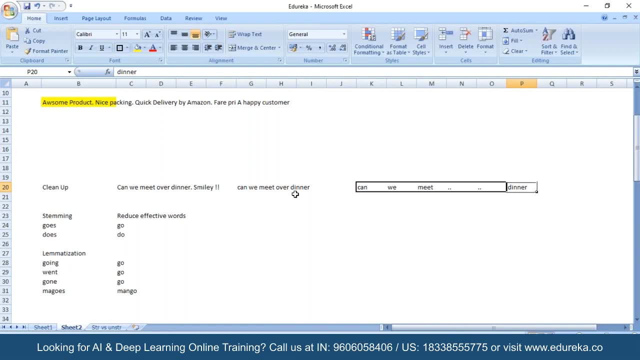 and breaking into words so that we can reach to the basic level of your text data and we can understand that. Okay, What is the frequency of meat word? What is the frequency of dinner word? What is the frequency of? we were so, after analyzing this, 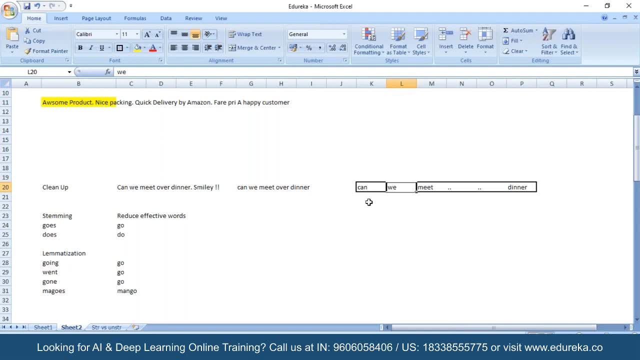 We can basically do a lot of different things. For example, we can find the summary of the whole text data again. Let me give you another example, For example, if I give you six season of Game of Thrones books written by Mr Martin. 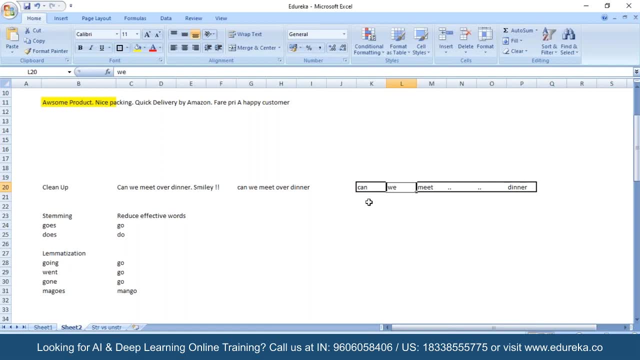 so Mr R Martin basically wrote Game of Thrones five, six seasons. Now I don't have time to go through all those six novels, So what I can do is I can use an LP model and I can input this PDF file of all those six novels and I will ask that okay. 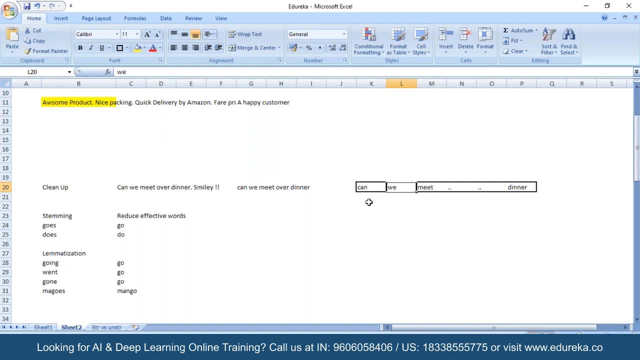 can you please tell me the summarized form of the overall overall novels, or maybe six season? So maybe it will give you the 40 or 50 lines summarized paragraph of all the story. basically, in 40 just simple sentences You can understand the overview of whole six seasons of Game of Thrones. 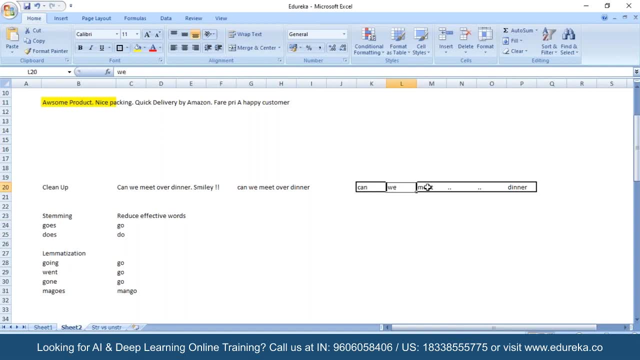 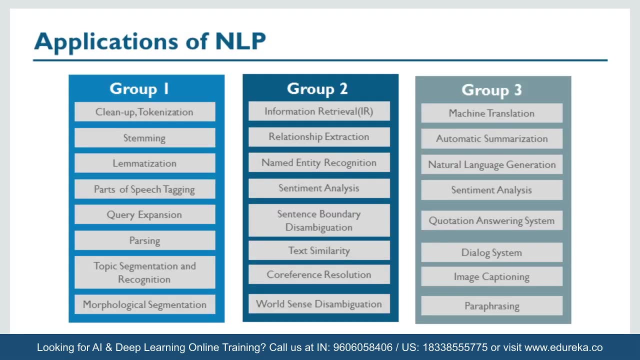 So that you can only do, if you can tokenize your sentence and you can go to the root word element of your text data, And that is the reason we always need to tokenize it Now, if I talk about stemming or lemmatization. so stemming is nothing, guys. 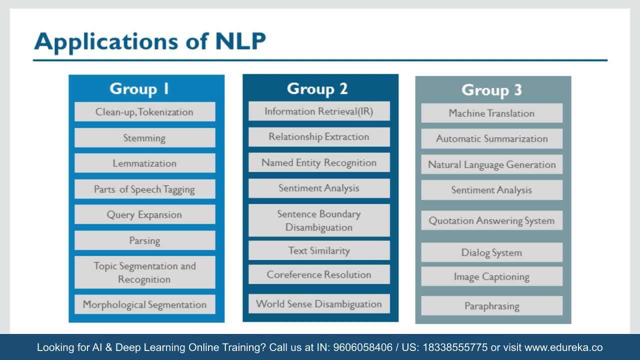 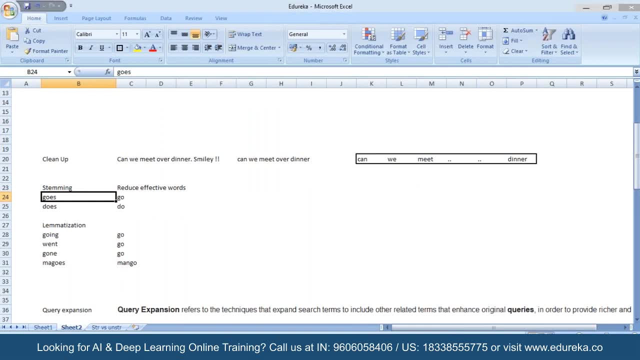 So again, let me give you an example: is stemming is nothing but going to the root word. For example, your data contains goes word. now going to the root word. The root word of goes is go. It may be went again, The root word is go. 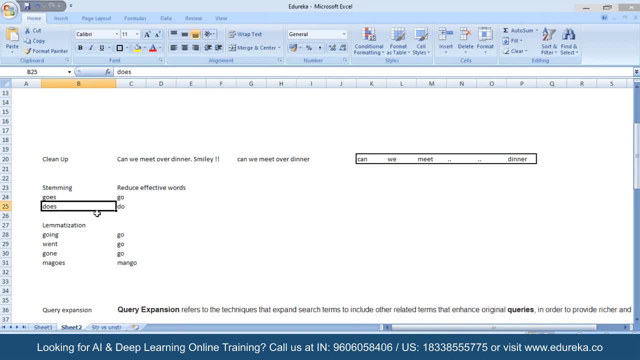 Suppose there is a word which is called us, but the root word of this word is do. So basically, what is stemming does is removing the suffixes and removing the prefixes of the word and taking it similar to or making it similar to the root of that word. 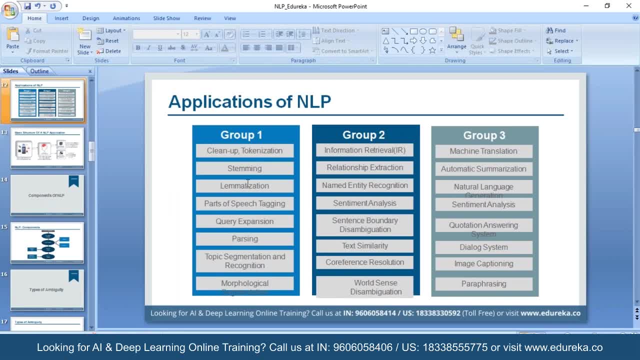 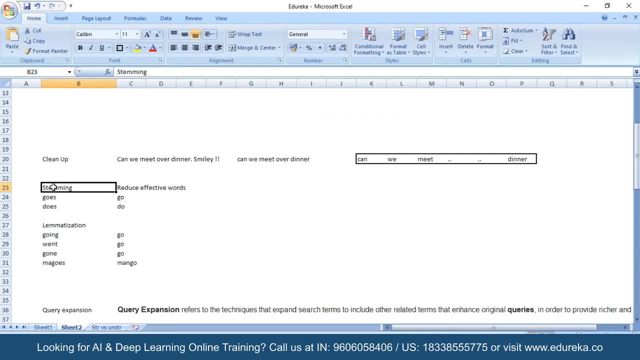 So that is called stemming. Now, another technique here which is mentioning is called lemmatization. Now, what is lemmatization? lemmatization is again very similar to stemming, where you are again searching for the root word of a particular given word. 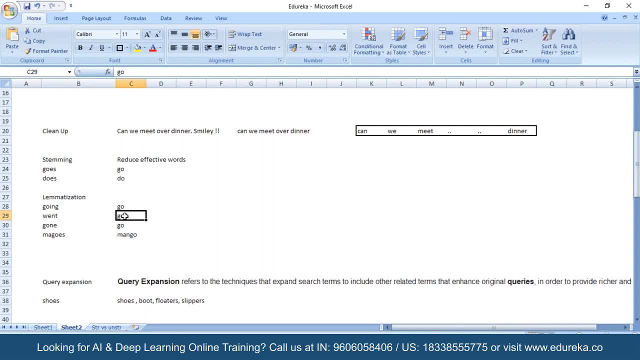 For example, going, the root word is go, went. again, The root word is go, also for gone, gone. It is cool. for mangoes It is mango. So basically, lemmatization and a stemming are very similar, It's just that lemmatization is more advanced. 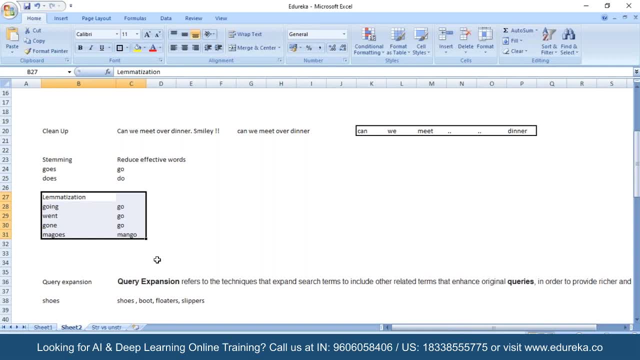 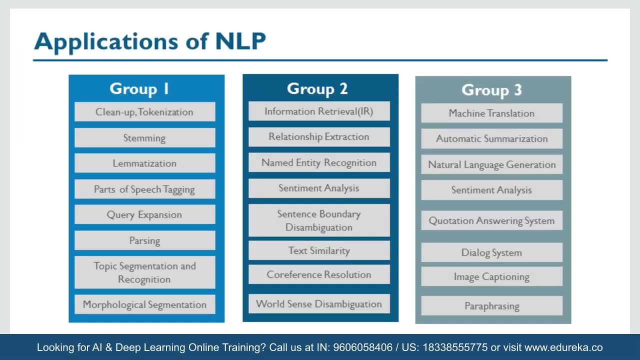 It can also understand the part of speech like it is a verb or adjective or pronoun or adverb. So lot of things it can do, So we will come To the details here. Again, overall things if I talk about a lot of different techniques. 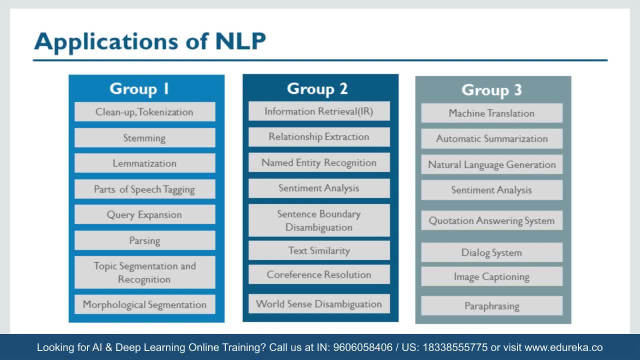 which has been mentioned here, to part of a speech tagging. So what does part of speech tagging does? is suppose you have tokenized your sentence into small words. Now it can identify each word, whether it is a noun or adjective or pro verb or a verb. 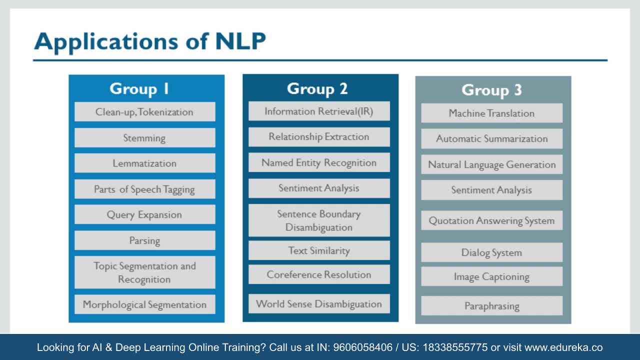 Now, what is query and expansion? now, query, expansion is something which is used in Google search. Let me give you an example. So, basically, suppose you write a word shoes, S-H-O-E-S shoes- on Google search, So it does not only search a word shoes. 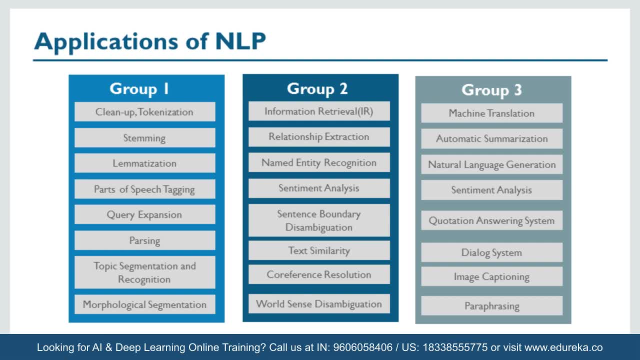 but it also searches some similar words to shoes. For example, it will also search shoes, boots, sleepers, floaters, so that it can give you all good results or all good web pages which are related to shoes somehow. So that is query expansion. Now 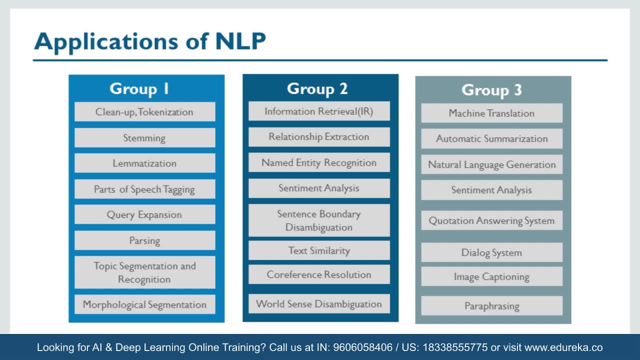 for example. let me give you the example. This is topic segmentation and recognition. Now, what is topic segmentation and recognition? So suppose you have basically thousand PDF data, So data in form of thousand PDF format file, PDF files, and all those thousand PDF files basically contains a story of a novel. 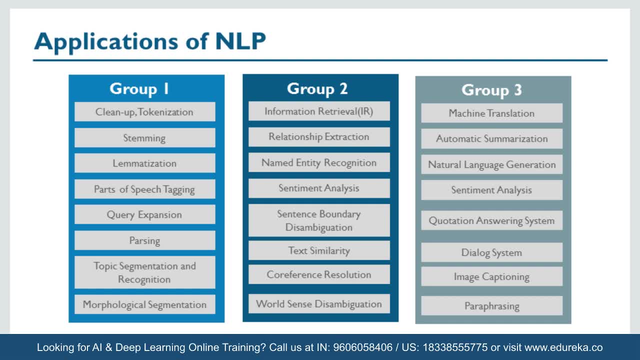 Now if you want to classify or cluster all those novels into some categories- for example, drama, romance, sci-fi, science fiction- So what you can do is you can pass the data in a PDF file of all those hundred novels and it will categorize them into maybe three or four clusters. first will 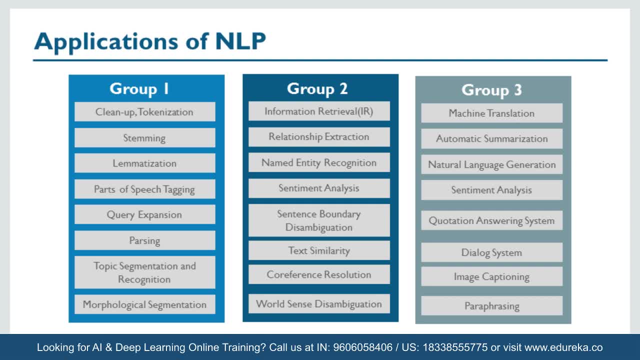 be sci-fi. second will be drama. Heart will be romance. fourth will be some other thing, action. So that is called topic segmentation And then recognizing whether which particular cluster represents which particular topic. is it drama, is it sci-fi? So there are a lot of things, guys, which has been mentioned here. 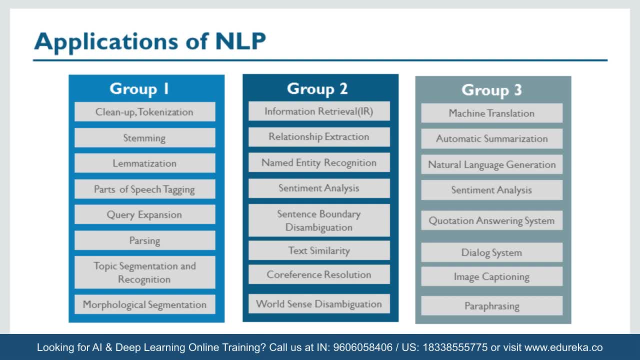 So what is sentiment analysis? as I talked about the Twitter example, like elections are close, Everybody's is putting their tweets, their sentiments, in a form of a tweet, So what I can do is pick the tweets data and I can analyze whether the sentiment is with the public, sentiment is with BJP or is it. is it anti BJP? 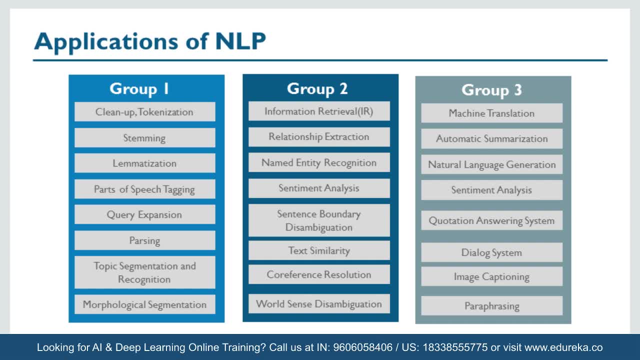 or maybe is it with the Congress or anti-congress, or maybe it is it with Mr KG well or against Mr KG one. So that is called the sentiment analysis. If I again take some another example: image captioning. So what in the image captioning? 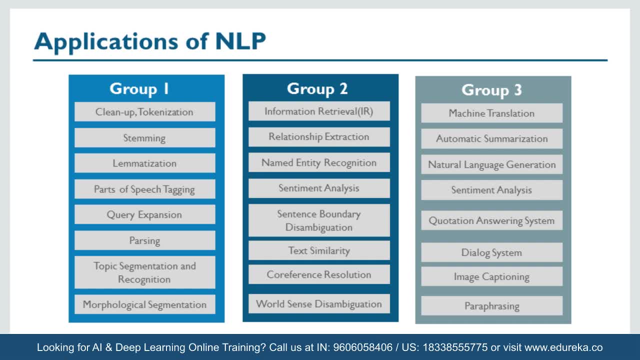 So have you seen the Netflix where, if you switch on the image captioning thing, what happens is if you are watching a movie, so whatever is is the scene, you can see a textual explanation of that scene. I'm not talking about talking about the subtitles. subtitles is a different thing. 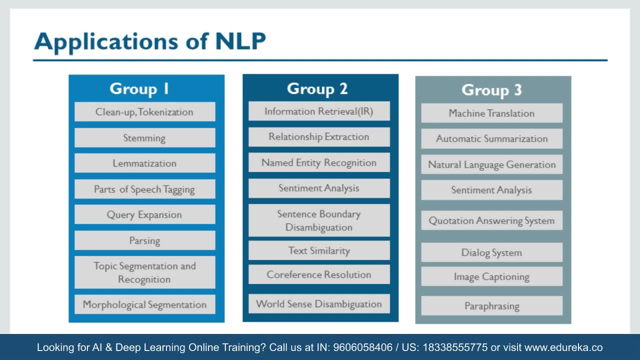 but it gives you a explanation of what is being played in the video. For example, the Thor picks up the hammer, The Thor hits Mr America, Captain America, with the hammer, Mr America, Captain America, falls down. So this kind of video explanation or image explanation where you can explain. 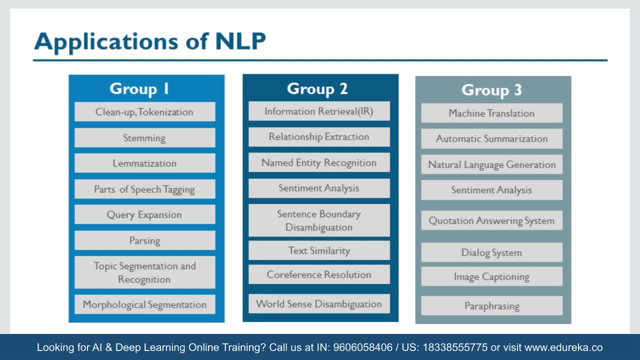 an image or a video with some written text. that is called image captioning dialogue system. Now, what is the dialogue system? That is a chatterbox. you write some query and there is nobody sitting on the other side and a computer system is answering your question. naturally, again, machine translation. 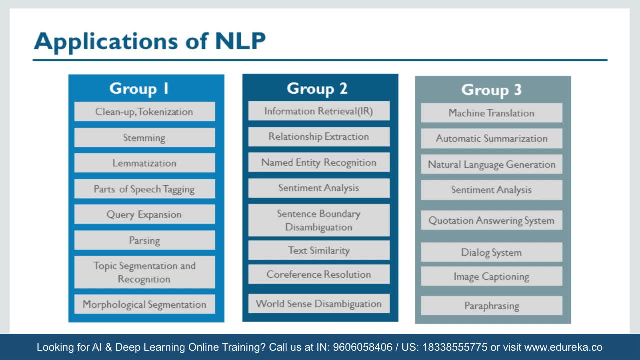 So what is machine translation? Have you seen that Google Translator? Now, what is Google Translator? So suppose you have to write French, but you don't know how to write French. Now you can go to Google Translator, You can write your. 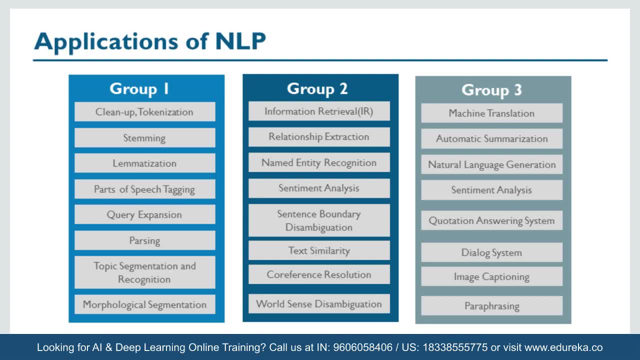 English words and automatically, whatever you write your sentence, that will be converted to French language. that is machine translation, language translation. Now, lot of different things are there, guys, So I can talk about the applications of natural language processing the whole day. As I said, lot of data, lot of information. 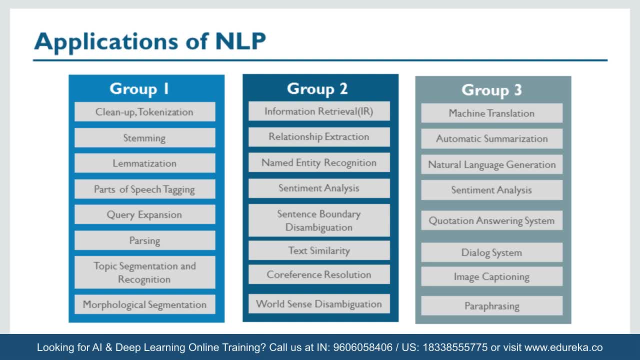 but very less research has been done. very less algorithms are present. So there is a huge scope of doing some research. There is huge scope of we inventing something. that is huge scope of we more improving some given algorithms. and there are huge scope of we developing lot of different application. 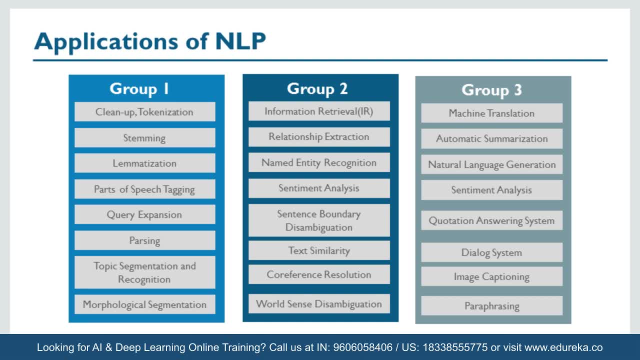 which can give us and which can improve the human life in better terms. This is all about the main applications of NLP. Now, guys, let me give you another example. here is lot of credit card frauds are happening on credit cards and with the help of NLP, 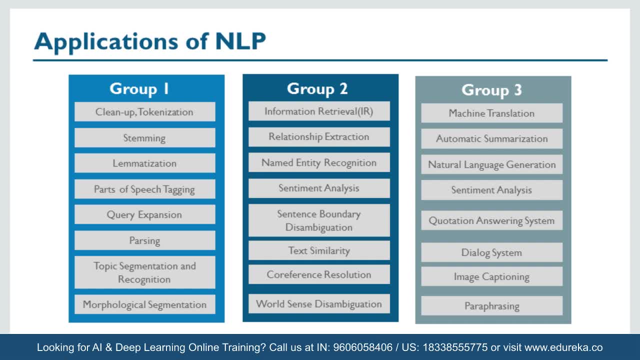 We can also identify whether this transaction and we can prevent the credit card frauds, For example. let me give you my experience, a project which I have worked on. So basically what happened is there is a very big loophole, which sometimes people do is basically suppose. 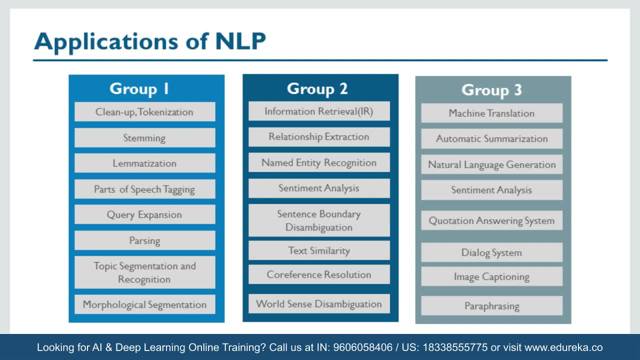 I am owner of McDonald's outlet right, I have a point of sale. So I have that swiping machine of American Express And what I do is I ask my wife to take American Express credit card, and I am The owner of the shop. my wife has American Express credit card. 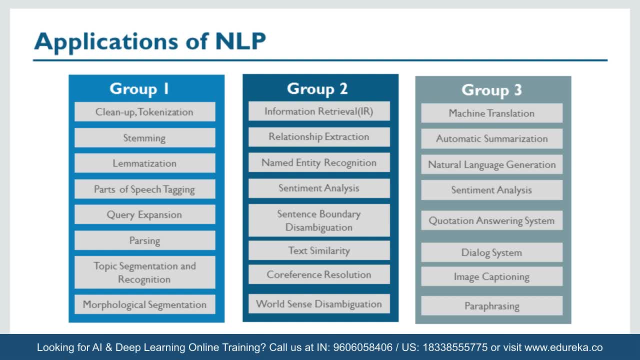 and she starts doing swipe and swipe- $20, $30, $40 and lot of swipes It does. now What is the benefit which I am getting here? So benefit is I'm getting free money for some couple of days. Why? because my wife need to pay the money. 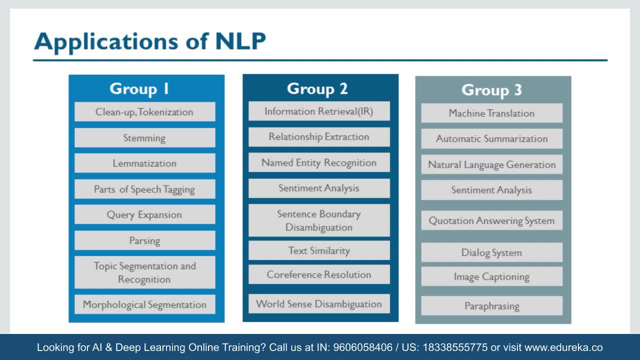 She has swiped after 30 days when the credit card transaction, when the credit card statement comes. but I will get that money after seven days. So basically I will get that money free for 23 days. How American Express can analyze and stop this fraud. 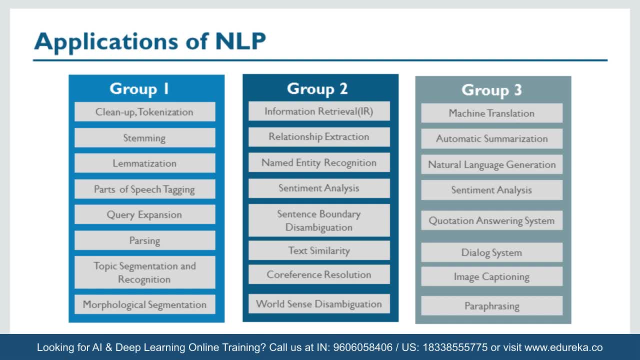 So basically what they do is they take the address of the merchant and then address of the card member. They match it. the pin code, They match it. the phone number, They match it. the email of the seller and the email of the customer, They match it. and if there is a certain amount of match, generally 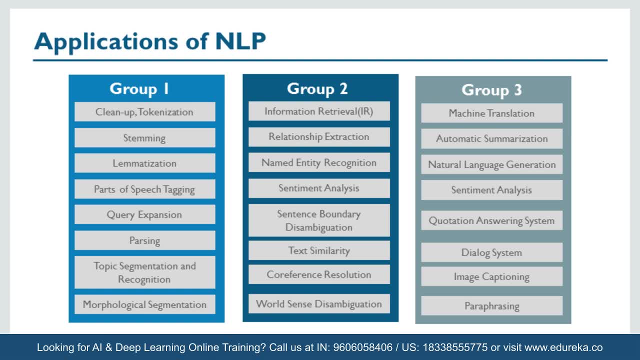 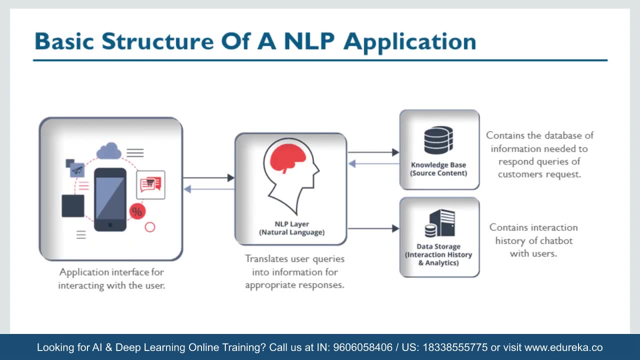 then they understand that, okay, this is some kind of fraud being Happened. So, guys, again lot of examples, lot of places where NLP is being used to either earn money or to save money. So let's move to the next part. So, as I mentioned, guys, the overall process of a natural language processing NLP application is like: 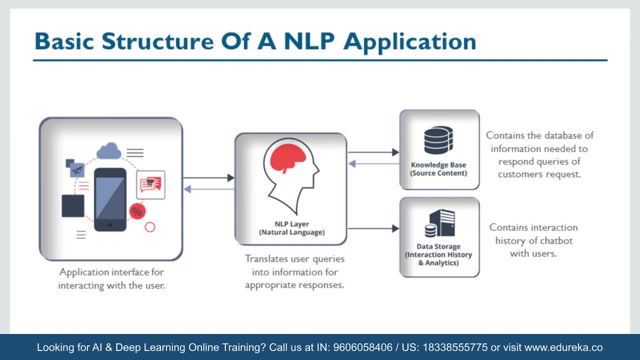 that. So, for example, there is a mobile or there is a maybe a laptop or maybe a desktop, So most of the times it is a mobile on mobile application, Then user or we basically interacted with maybe a chat, chat or maybe a message, or maybe Facebook or maybe Twitter. 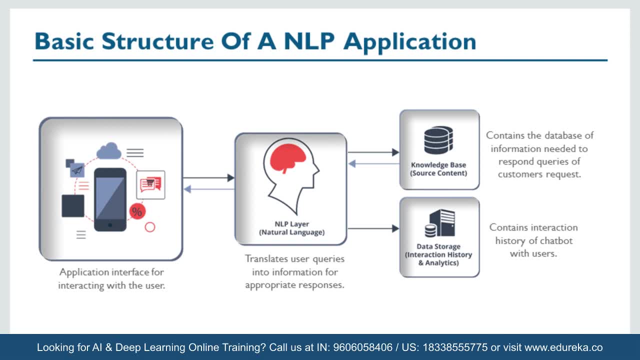 or maybe WhatsApp, and then what happens is the data which you write is sent to the NLP layer, which is basically a program written with artificial intelligence logic which translates your user queries into appropriate rest of responses, and then it sends you back and also, if it needs to contact. 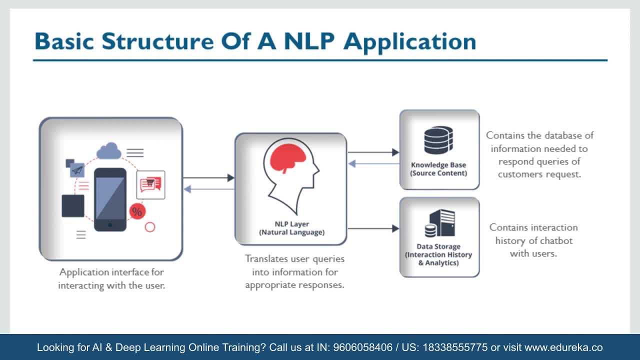 answer your question. if it needs to contact any knowledge base or a database where a lot of information is shared, So it will contact that also. for example, suppose this NLP layer is Alexa, So when you ask Alexa to do something, what it does is it may contact any database. 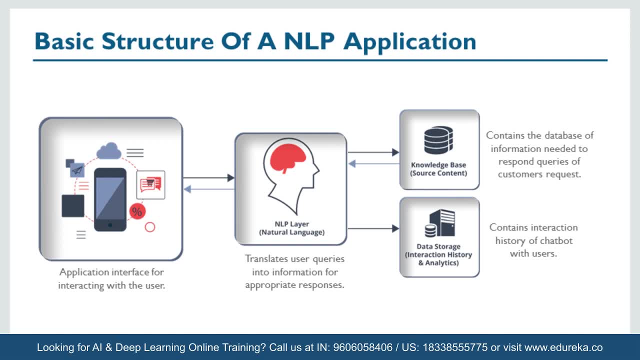 or it may contact any Google repository, or it may contact any website and to fit some information to provide you. on other hand, whatever you interact with Alexa, whatever interact with NLP layer or whatever you interact with this NLP application, It can be stored, as well as your interaction history. 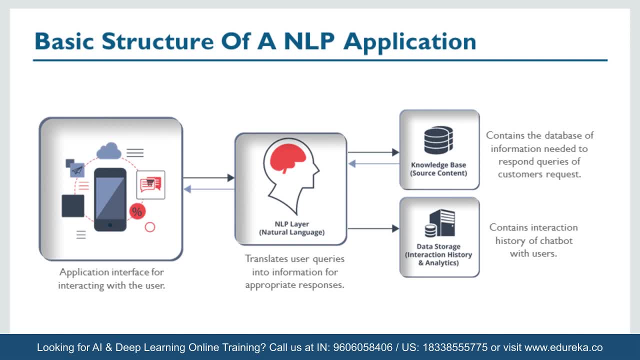 And why do you store it? because when you store this data, you can use it for analytics purpose, for maybe some prediction, maybe some analysis, maybe drawing some good insights from the radar, maybe understanding the user history, For example with the chat you have done with Alexa. 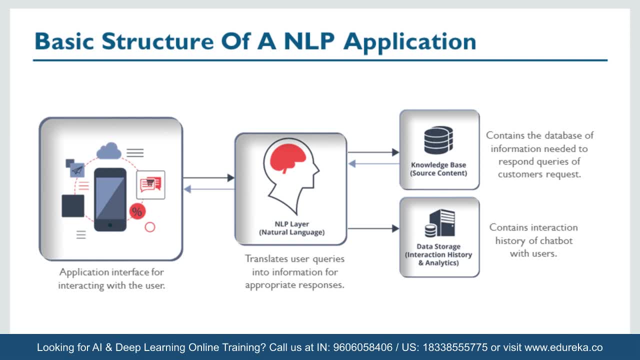 I will be able to understand That you like pizza very much. Why? because each Friday you are ordering a pizza. Maybe I can understand that you are very short-tempered guy, because when you chat with your friend, or after two or three minutes, 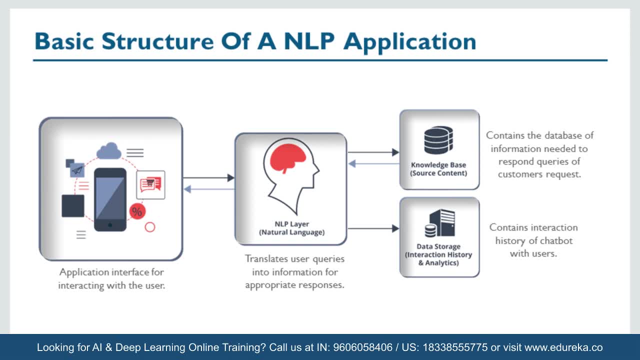 if he is not responding, you start writing hard words. Maybe I can understand that you are a diabetic person. Why? because you ask Alexa to look for some diabetic remedies. Maybe I can understand that your salary account is with Citibank. Maybe I can understand that you work at Google. 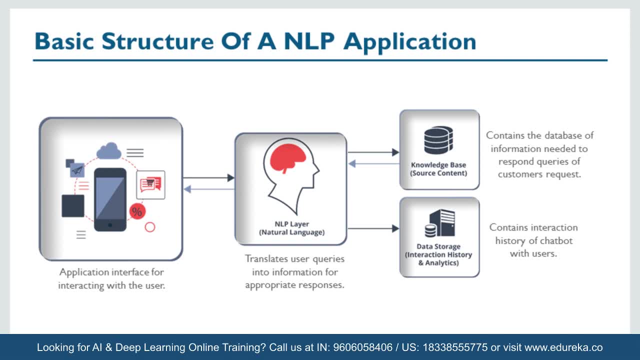 Maybe I can understand that you like drama movies. Maybe I can understand that you write you like a Ramon as a music director. Maybe I can understand that you are unmarried. Maybe I can understand that you, you don't have any child. So, guys, this is lot of things which is being happened in real world. 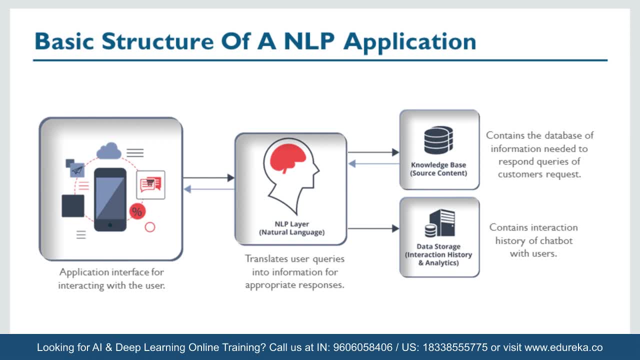 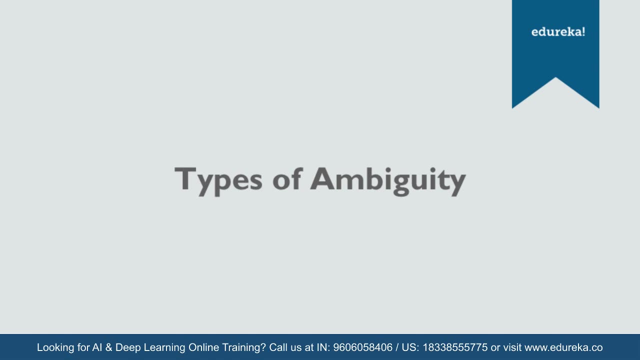 Lot of things which you can do, a lot of things which is being done and lot of use of huge amount of data And a lot of research have been done. This is how an overall NLP thing works. So, guys, one of the biggest problem in NLP is the ambiguity. 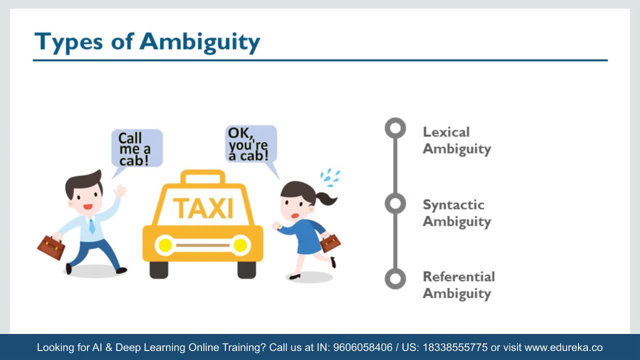 Now, what is ambiguity? Ambiguity is basically where a word or a sentence or a context is basically pointing to two different meanings. For example, suppose there is a person who calls call me a cab. Now he is trying to book a cab. 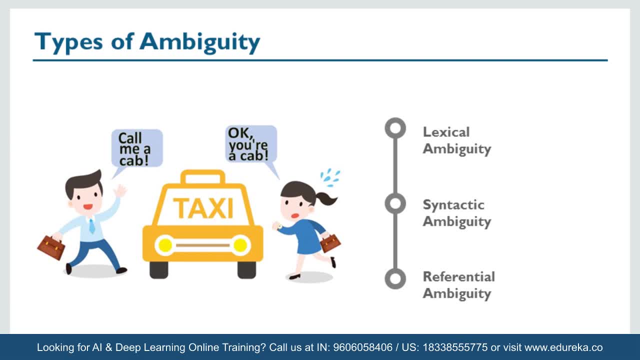 But the person in in front of him understand that his name is a cap. So this is a kind of ambiguity which happens in natural language and sometimes programming languages like packages, machine learning, deep learning algorithms or computers are not able to understand whether. what is the context? is it the first meaning or is it the second? 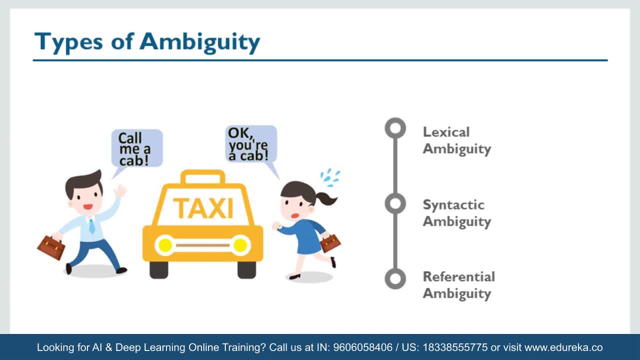 meaning. so that kind of ambiguity is very much there in natural languages. That is one of the challenges Which we need to solve, and ambiguity is basically of three types. So first is the lexical ambiguity, The second is the synthetic and ambiguity, and the third is the referential ambiguity. 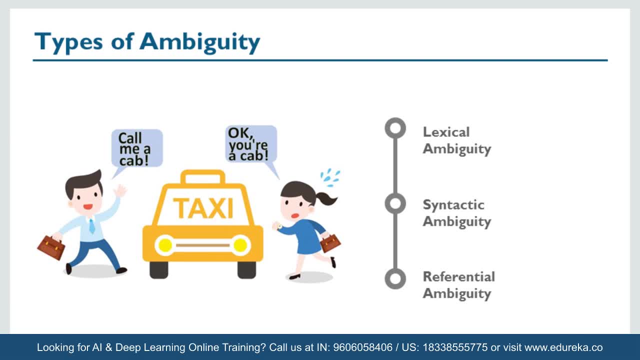 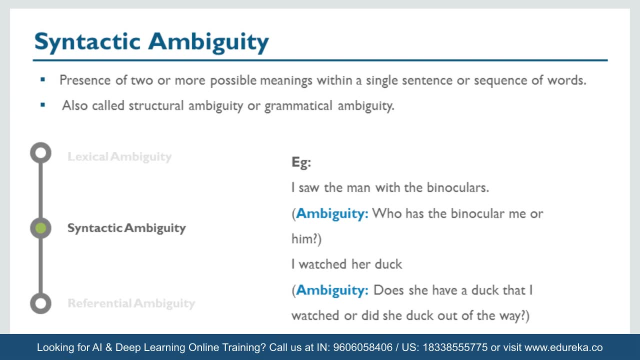 So let me take an example of the first ambiguity, which is lexical ambiguity. So lexical ambiguity is the ambiguity which happens due to a particular word. For example, see the first sentence- He is looking for a match. Now, the meaning which I understand is: she is looking. 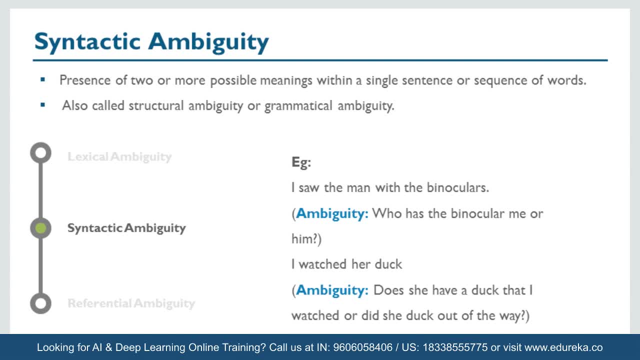 For a life partner. But suppose there are four lines or four sentences before this sentence and the girl went to a mall where she wants. She has basically bought a dress and she want to match her shoes with the dress. So she want a match. but the literal meaning, or the most popular meaning, goes. 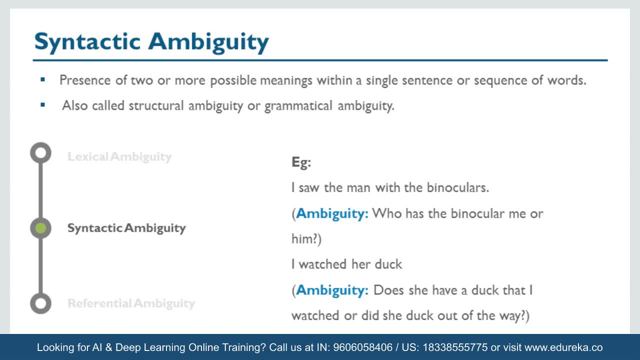 that she wants a life partner. right again, the same way if you go through the second sentence. The fisherman went to the bank. Now what is the bank? Is it the financial organization Bank of America, or is it the bank of the river? 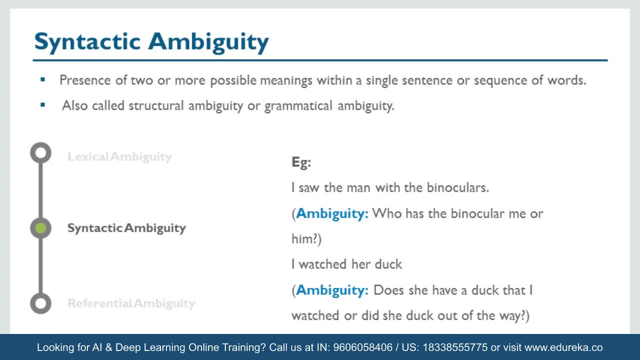 So this is the kind of ambiguity which is happening due to a meaning of the word, when a word has more than one meaning. So this is very much common into natural language processing and this is a challenge for artificial intelligence and the computers to solve it. 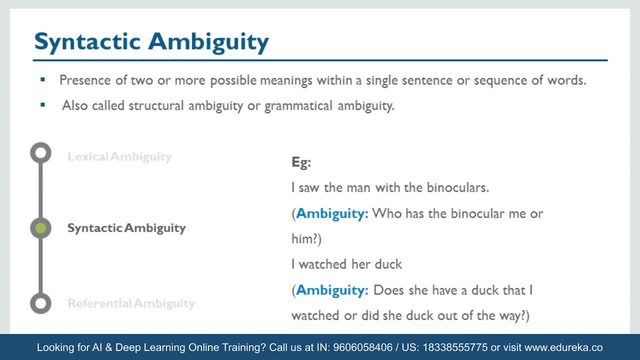 Then again syntactic, and the ambiguity is Basically the ambiguity which happens not only due to a word, but a group of words, maybe a sentence, For example. if you take the first sentence, I saw the man with the binoculars. Now, when you write, I saw the man with binoculars. basically, what does it mean? 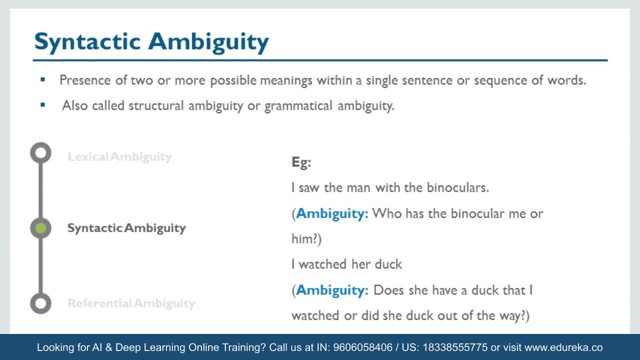 does the man whom you saw the binoculars, or you saw him with the help of a binocular. next, next, again, the next example you have. I was not Now. did you watch the animal the world does which the girl was possessing, or He talked you, she talked you out of the way? 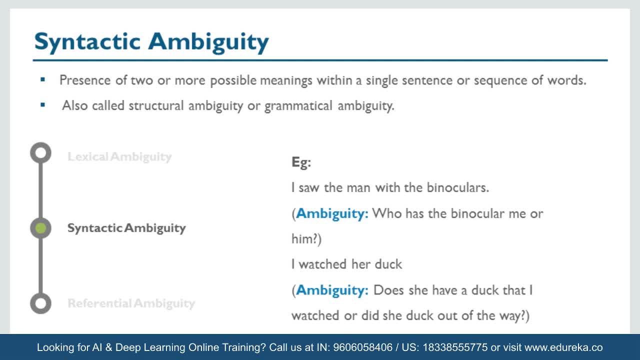 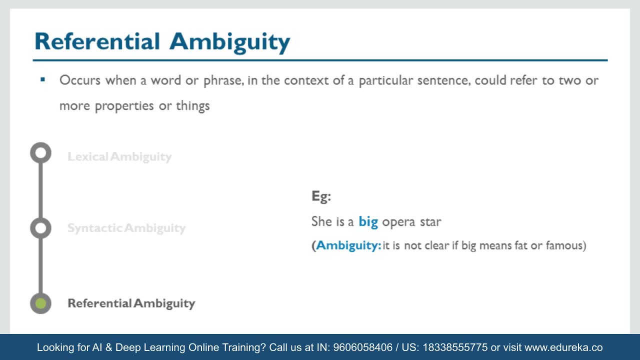 So basically this kind of ambiguity is called syntactic ambiguity, which is due to a particular sentence. Now again, referential ambiguity is the ambiguity which happens due to some reference, due to some context. which is the example is: he is a big over a star. 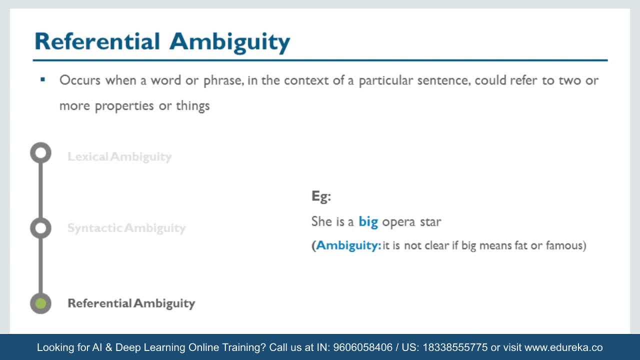 Now, Who is big? is the over a big, or is the star is big? So this kind of reference ambiguity is also there. So, guys, these three kinds of ambiguity is generally present in natural language, and that is the reason the machine learning or deep learning algorithm has to be so. 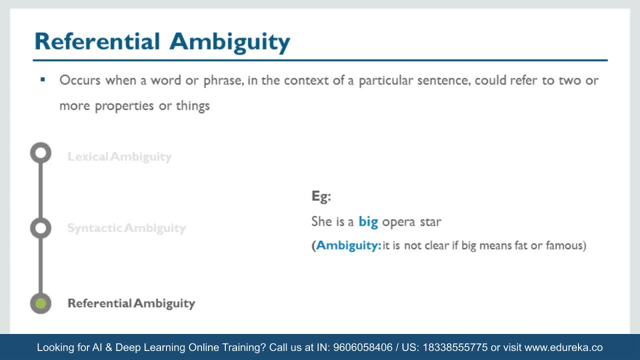 smart that when you take your text data, when you process it, when you bring to the machine learning or deep learning algorithm, it should be able To understand the ambiguity, It should be able to understand the context which you are talking about and it should should be able to read the right meaning of the word and the 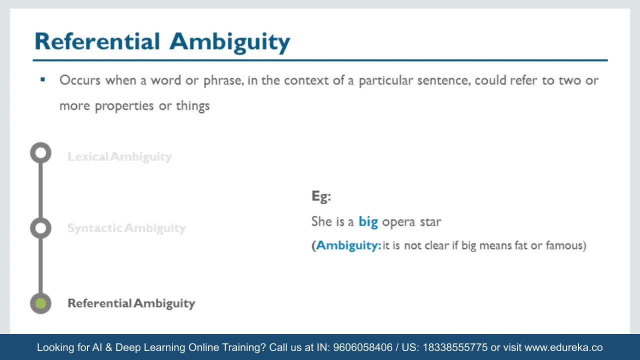 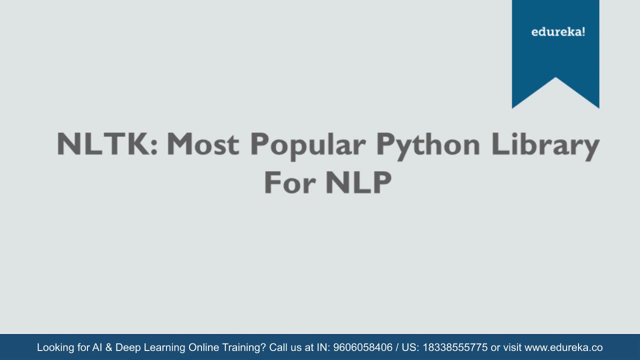 sentence and the context. So that is one of the challenges of the natural language processing thing. Now, what is the most important package? What is the python package which is used for a natural language processing? the two important packages for natural language processing is: first is NLTK and 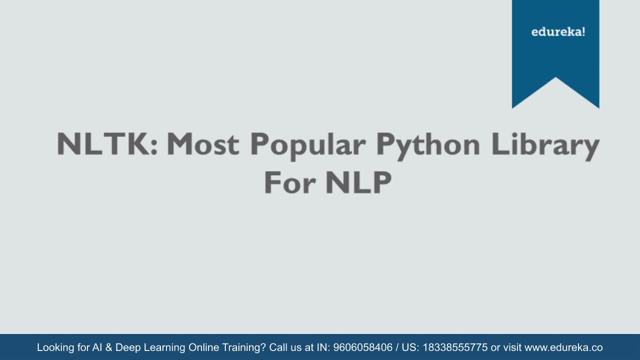 second is specie, SPACY, specie. However, I would recommend you NLTK. why? because NLTK is easy to learn and especially for beginners, who does not know NLP before, NLTK is the best thing to study. NLTK is mostly used in learning and development purpose, while specie is 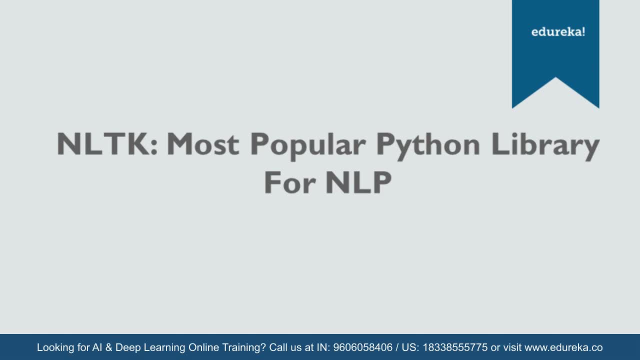 used by most of the organizations in real-time production and if you know the NLP concepts and if you know NLTK, it won't be very hard for you to switch to a specie. So you should. recommended package for you is NLTK. 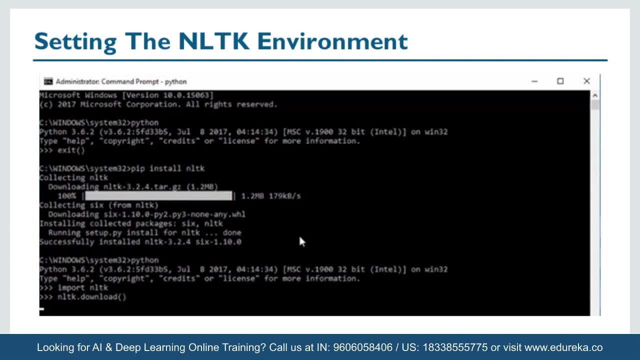 Now, if you want to install NLTK, this is very simple, guys. As you can see in python, This is a python package which can be just installed by writing: pip: install NLTK, pip. pip- install NLTK and, guys, this will be installed. 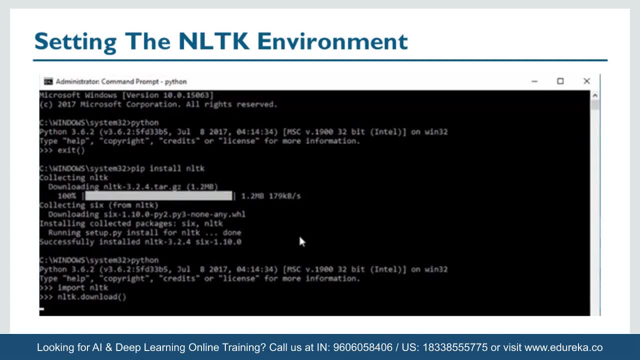 This is as simple as that. also, after You have done with installing, you need to download some of the packages, some of the example text, some of the different facilities, utilities which are presented to NLTK on. for that, You just need to write NLTK download. when you write NLTK download on your python. 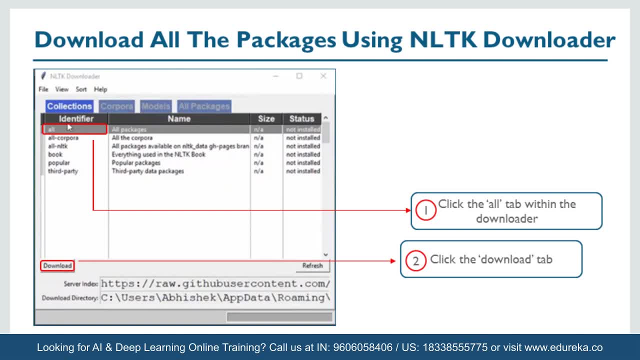 console window like this will open, where it will be like a list: all corpora, all NLTK book, popular third party. So what are these components all corpora basically contains? there are a lot of different corpus documents available in NLTK package which you can avail and you can use them for. 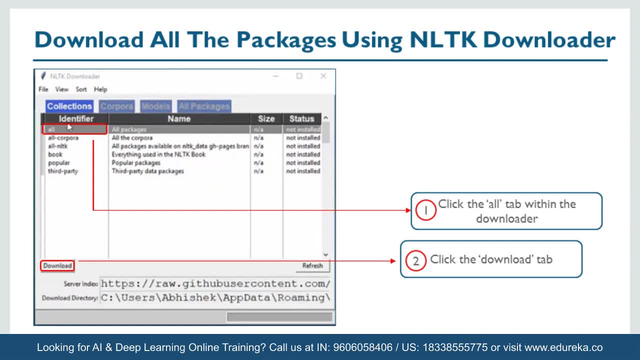 learning purpose. For example, the speech with Mr George W Piss Bush, the president of us, made in all four years of his presidency, is available on NLTK package as a text data. So if you want to analyze, you can just take that data and you can use it. 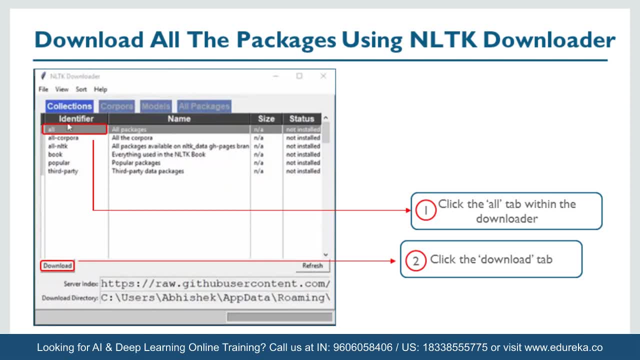 There are a lot of books, ebooks which are available so that also you can download, and a fetch from NLTK package and you can use it. There are third-party packages as well, So better option is click on all where it is written, all so that you can it can download. 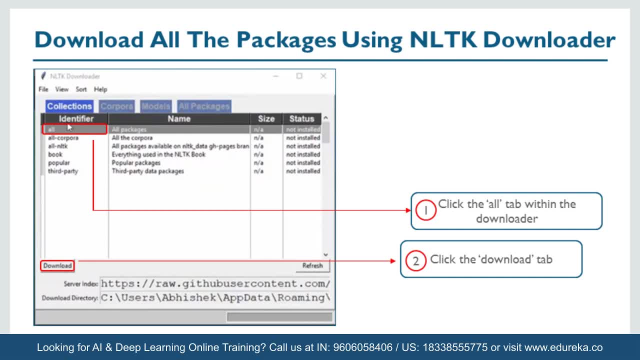 all the things which has been written here, and just click on download and it will download all the books, all the corpora, all the examples, all the third-party packages, so that you have the complete NLTK things with you Whenever you need to use it. 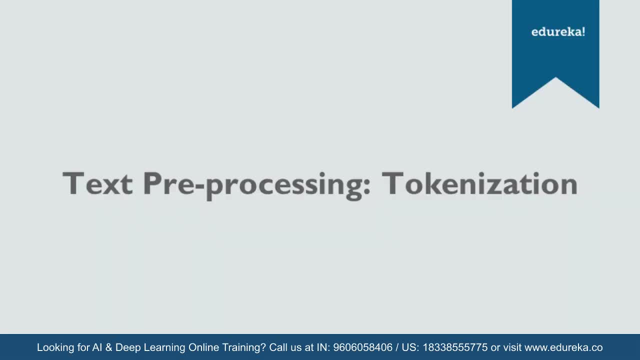 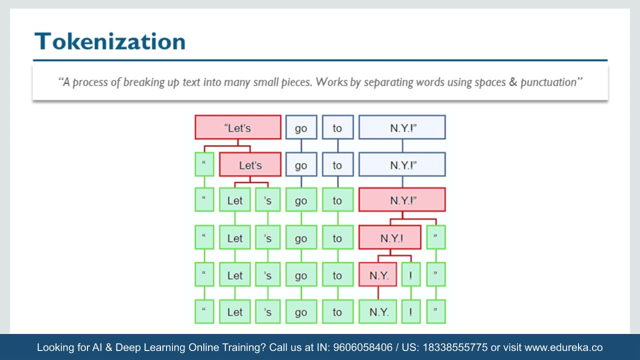 What are the steps we do for NLP thing? So the first step is the tokenization thing. Now, what is the tokenization? tokenization, guys, is nothing but taking a sentence, or maybe taking a document where you have a lot of sentences, and breaking it into simple, simplest. 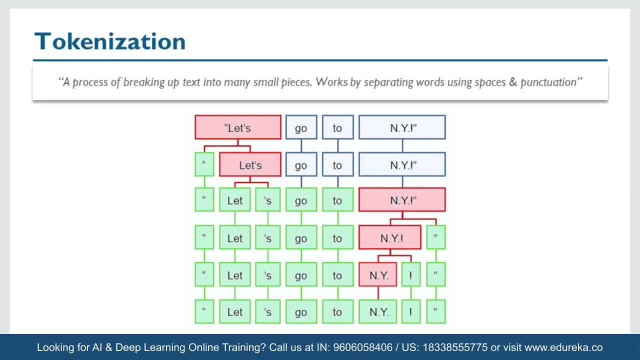 unit. that is what. so, for example, if you see the sentence is let's go to new off, and when you tokenize it It becomes Let's go to New York. and then in the next step it become let then s go to New York, and 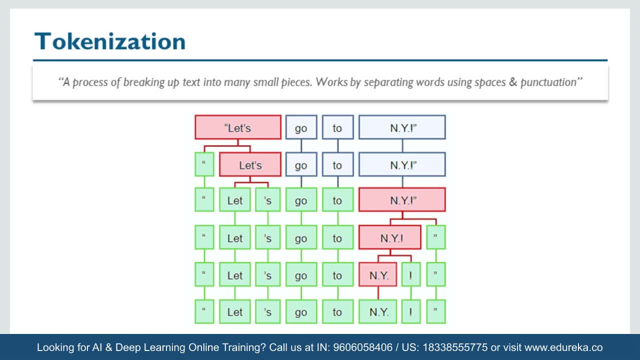 this way, guys. basically you can tokenize your document or your words or your sentence to basic words and then each words. you can analyze that. what particular words were used? What are the positive words which were used? What are the negative words which were used? What are the frequency of good words? 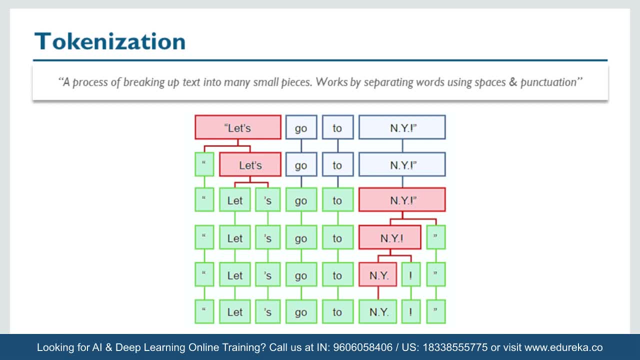 What are the frequency of bad words so that you can do, and after that you can see whether the sentiment of the person who has written this, this statement, is positive or negative. Is it good to society? is bad to society? What mood he has is in in depression, is in a good mood. 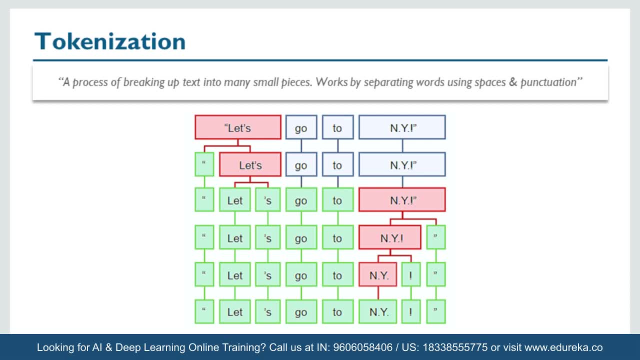 What does he want to convey? or maybe, if you have thousand lines of sentences, what is the extract of those sentences? everything, guys, you can do, but the only thing is that you have to start with tokenization. Now, what is the tokenization? as I mentioned, it basically breaks. 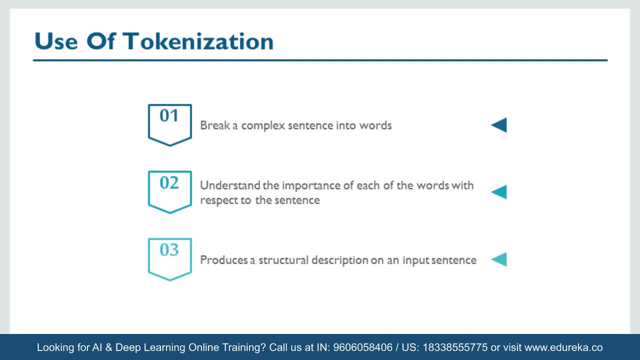 The complex sentences into words so that you can understand the importance of each word and then you can structurally represent them into better information. Don't just think that we generally break our sentences one single pieces. Sometimes we also make a couple of words or maybe couple of tokens, and those or maybe 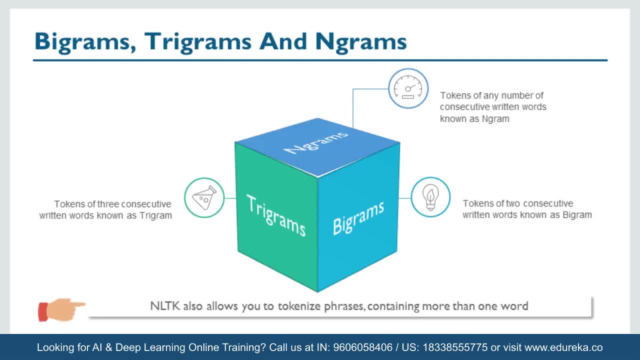 three words together, or maybe four words together, and that is called by gram, or try gram or engram. So if you are breaking the sentence in such a way that each token contains two words, that will be called by gram. if you are breaking the sentence in such a way that there are 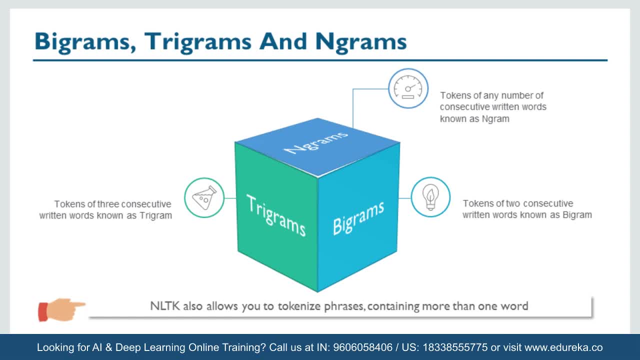 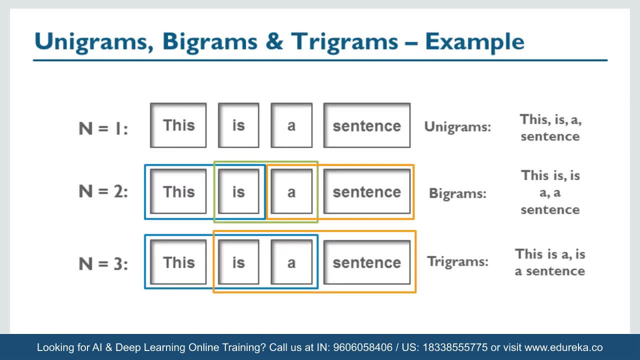 three words. that is called try grams. So now, how does this diagram looks and why do we create this by gram and diagram? Let's see. So suppose this was your sentence where you have written: this is a sentence. now, if you create uni grams, 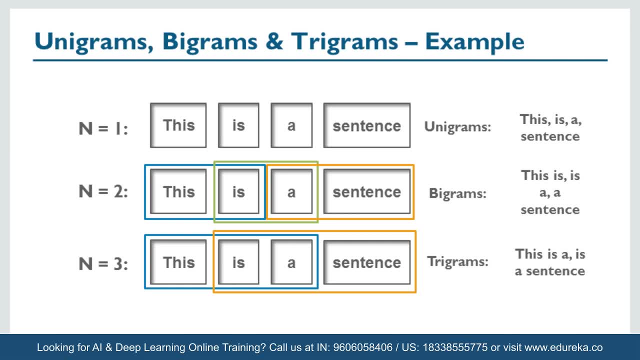 So uni grams basically, will break it into single words. This is a sentence. Now, if you create a biogram, there n is equal to 2, the tokens will be: this is the second token. is is of. the third token is a sentence. Now, again, if you take n equal to 3, that means you want to create a try gram from the sentence. 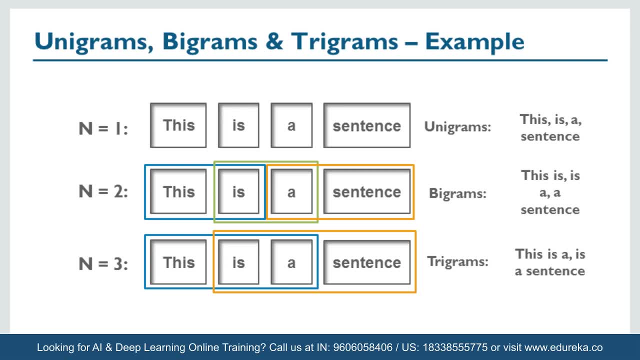 This will be the token will contain three words. This is of is a sentence. now, guys, Why do we create it? How do we create it? We know it. Now, why do we create it? Let me show you an example that why do we create it. 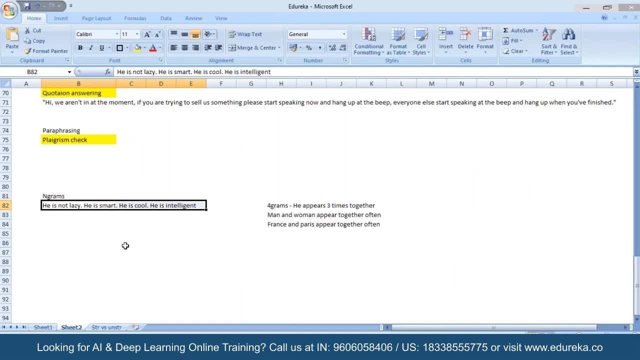 So, for example, let's see this sentence. This sentence says: he is not lazy, He is a smart, He is cool, He is intelligent. Now, if I create four grams, I mean the four grams where I tokenize them into four, four words. 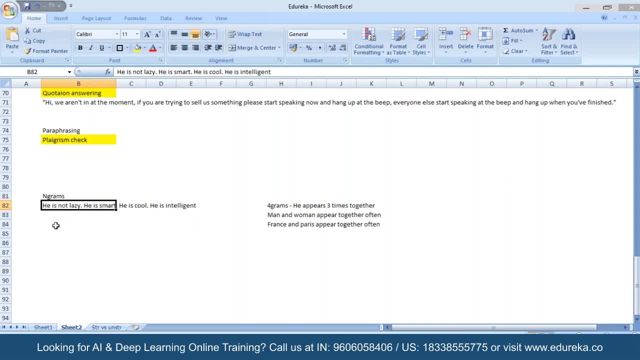 So can you see that if I create four grams, He words repeat four times. So see, here he is not lazy. So in this he word is again coming with he four times, he with he, then he with he. so basically, why do our? we are doing it. this type of analysis basically will tell you that generally in 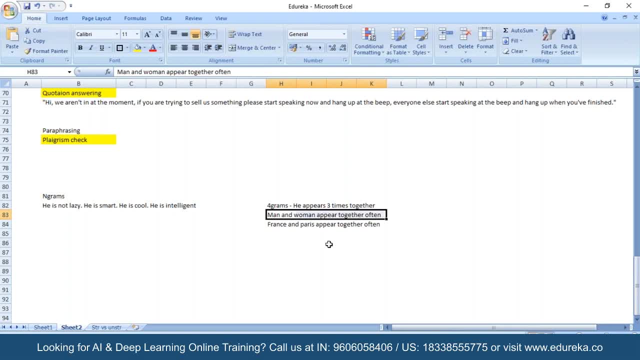 natural language. man and woman appear together often. also, France and Paris appear often together. India and maybe Pakistan Generally happen together. Maybe New Delhi and India Gates happen together. So basically, this tells you the probability of a world occurring with a particular word. India with Pakistan has a great probability of occurring if you are talking about any. 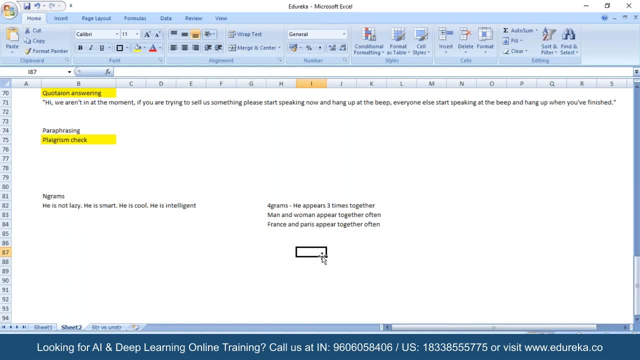 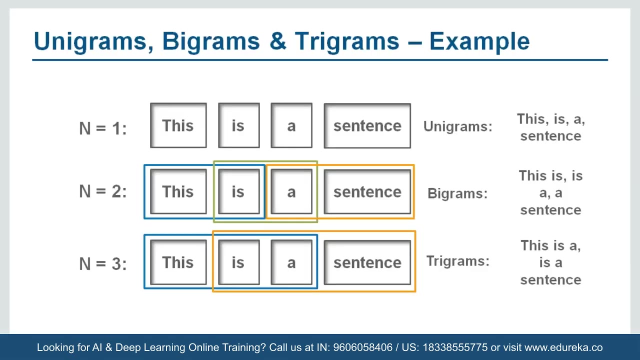 news, or if you are talking about any international conflict, but India with Bangladesh or India with Bhutan or Myanmar as a lesser problem. So this kind of analysis where you want to understand that which particular word happens with or maybe occur with which particular world. 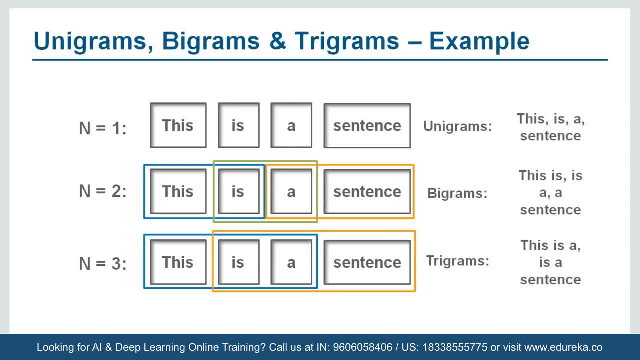 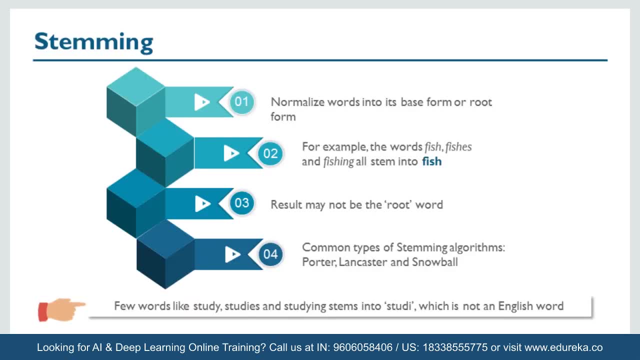 So in those cases, unigrams by grams and try grams of the whole data is very useful. Now, what is stemming? So, as I said, there are different words and and words are in two different formats. For example, the word fish- it may appear like fishes, fishing- and a lot of different formats. 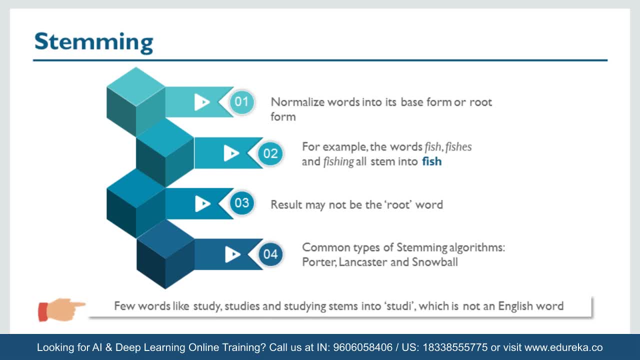 It may appear in your Document, on your text data, but the original word to the all those words is fish. and suppose, if you do not make it this data to your original data? Suppose, if I have a word called fish, I have word called fishing. 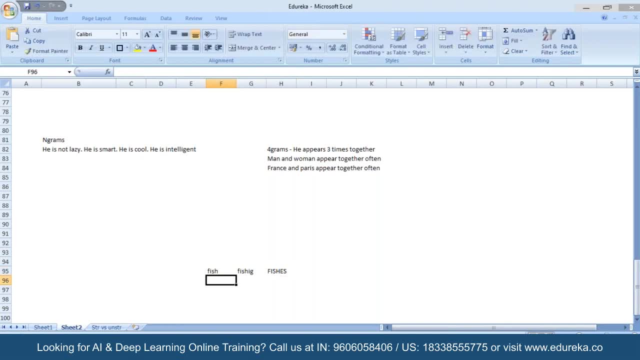 Right, and if I have word called fishes? Now, if you do not make it to the original data, what will happen is, when you try to analyze it, it will be treated as three different Words. Right, but the reality is that all the three words relate to fish. 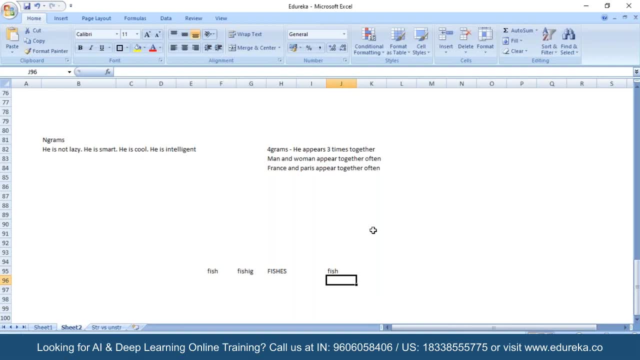 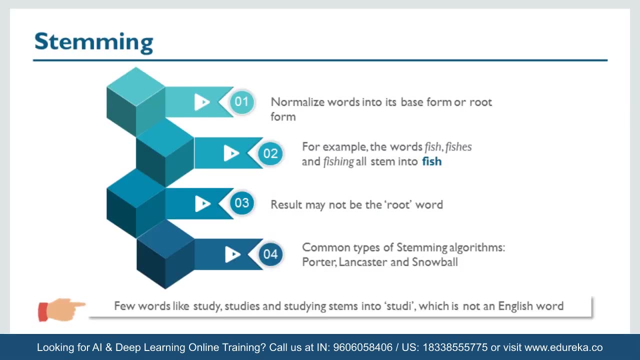 So that is the reason, guys, stemming, or lemmatization, is important to understand and to reduce the dimensionality of your data. So all these three words represent fish, So you need to convert it into fish when you are analyzing your text data and and that can be done. 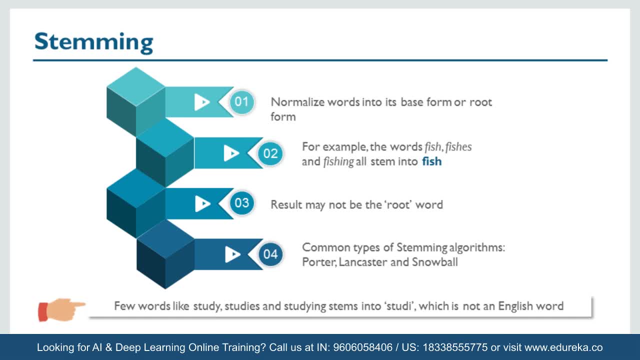 with the help of stemming. So, as I said, stemming- basically what it does is try to remove some suffix or prefix and then it try to create the original word. but this is not a very good technique and sometimes it fails, like if you have words like study, studies and studying, and if you want to apply the stemming algorithm, it will. 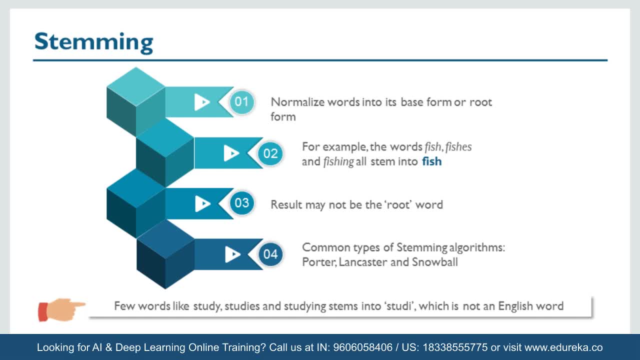 the word which you will get is STUDI, study, which is not an English word. So sometime it fails And you need to use some different algorithm, So let me give you an example here. So what we have done here is: from NLTK, dot stem, import Porter stemmer. 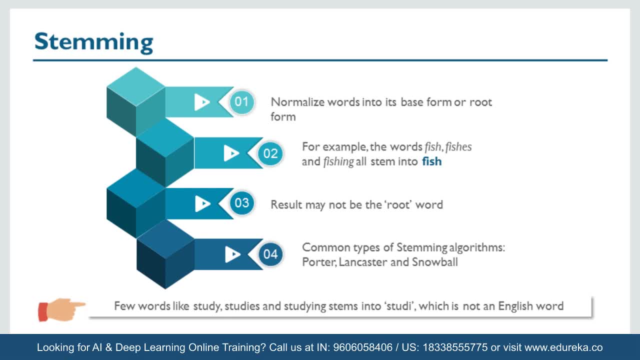 So basically, Porter stemmer is an algorithm which is used to stem the words and PST equal to Porter stemmer. Basically, you are creating an object of this Porter stemmer process so that you can use it Now if you see PST dot stem. 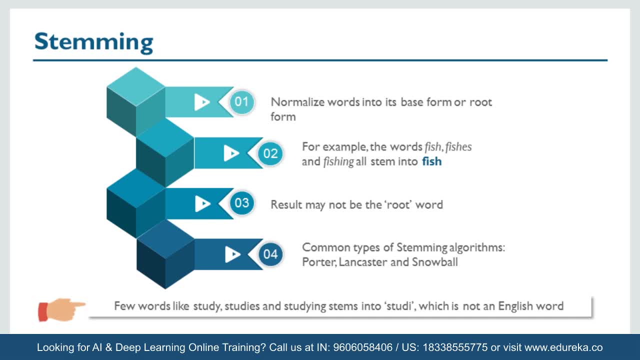 Now stem, Now PST, dot, dot, stem. and the word you wanted to stem was having. so you can see the output which you got is half. So it worked right: having word got converted to have. now Let us try this on some different words. 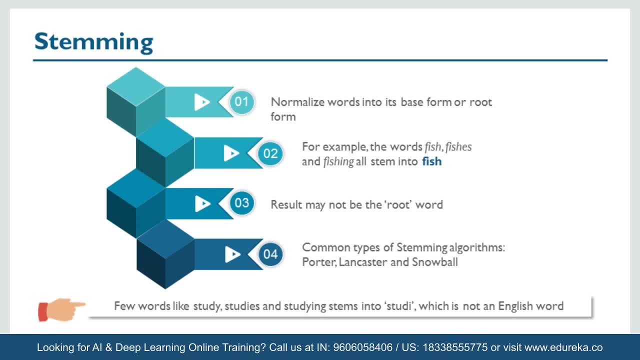 Now I have a list of words like give, giving, given and give. now if I apply the stemming algorithm on all these words, can you see the output? the first word: give- converted to give, that is fine. Giving converted to give, that is also fine. but given and give, they were not being converted to the. 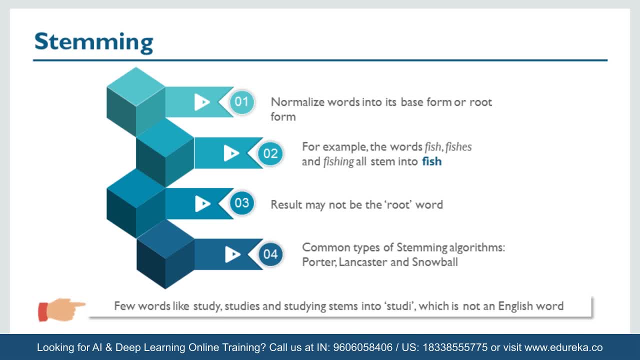 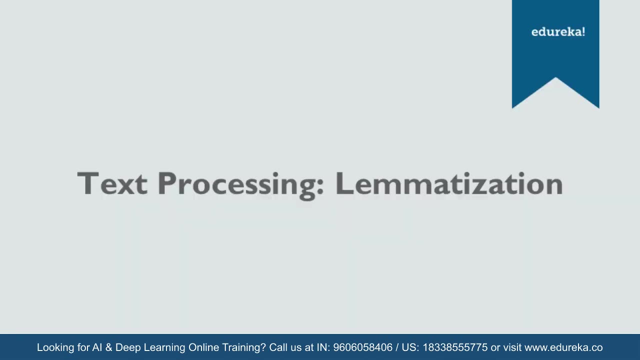 original word give. so that is the problem, guys: Sometimes the stemmer is able to convert and sometimes the stemmer is not able to convert it to the original word. Okay, That is the reason we have another algorithm, which is called lemmatization. now, lemmatization is similar. 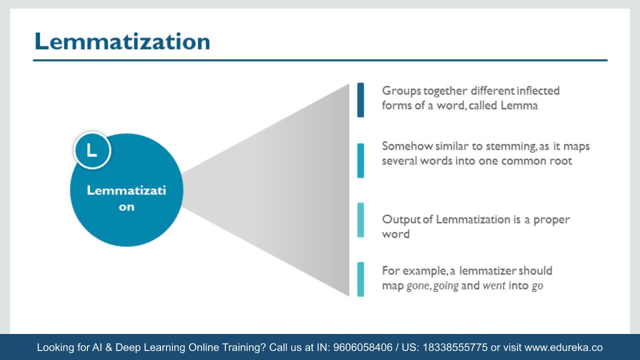 to stemming. It also tries to convert the word into the original word, but it can do it in a very efficient manner and the performance of lemmatization also is better than stemming. So I will show you with some examples here. Also, please notice that output of lemmatization is also always a proper word, not like the stemming. 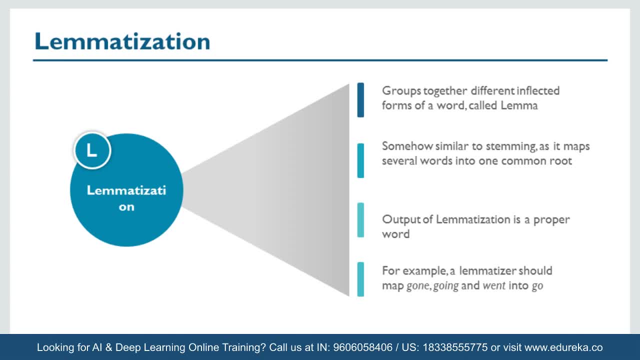 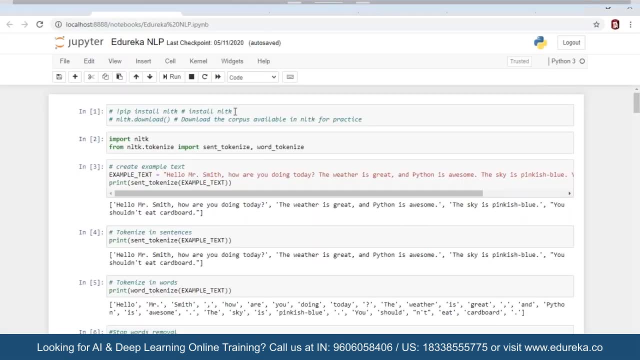 thing, So better guys. Let me show you a python example here so that it will be More clear to you. So this is how we installed NLTK: like pip, install NLTK. and then this is how you do the NLTK download. I have commented it here because that was not required and I have already done that. 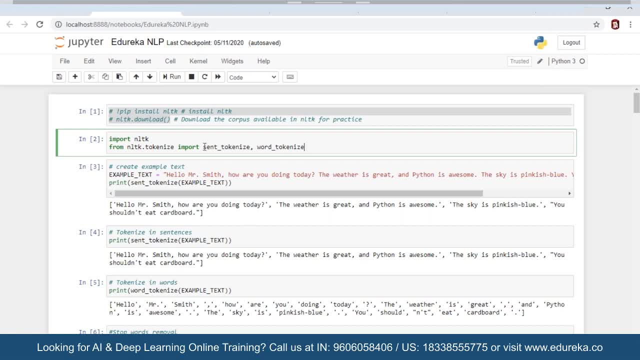 So here I have imported all the packages which were required. Now, if you can see, here I have example text. now, example text is nothing, but a text has been written. Hello, Mr Smith, How are you doing? This is like a chat, guys. 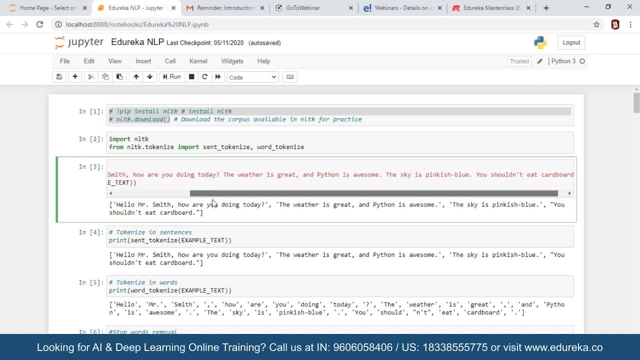 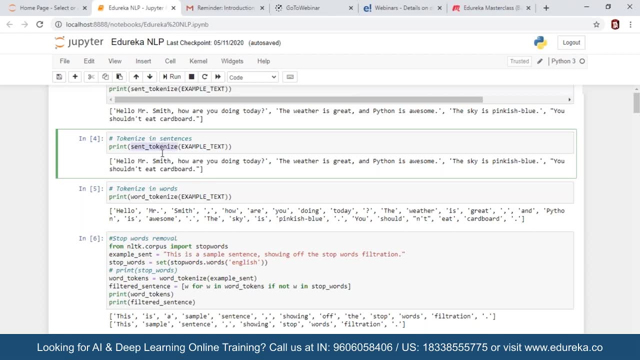 The weather is great, The python is awesome, The sky is pink, is blue, You should not be at the cardboard, and all when I want to tokenize it into sentence. I have a function called sent underscore tokenize and if I apply the sent underscore tokenize, 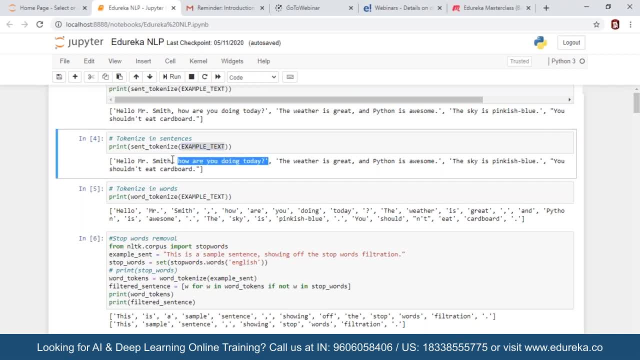 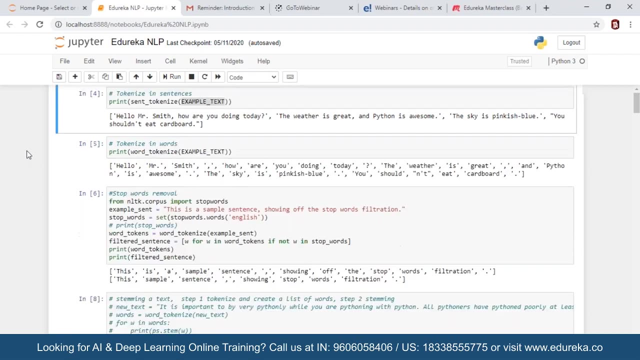 thing. can you see that the output is basically: each sentence is now a element of this list, So it break the complete text into sentences. Now the next element is again a sentence, and so on. rather, if I want to convert and change, I can tokenize them into word. 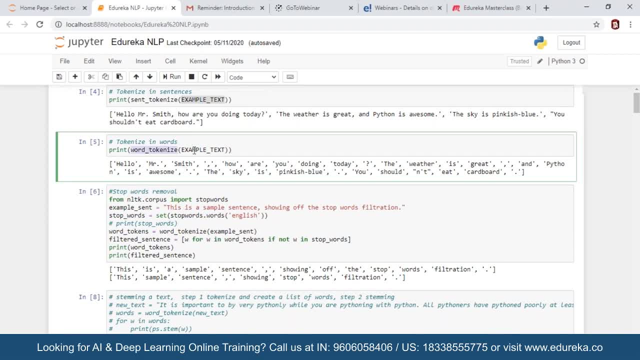 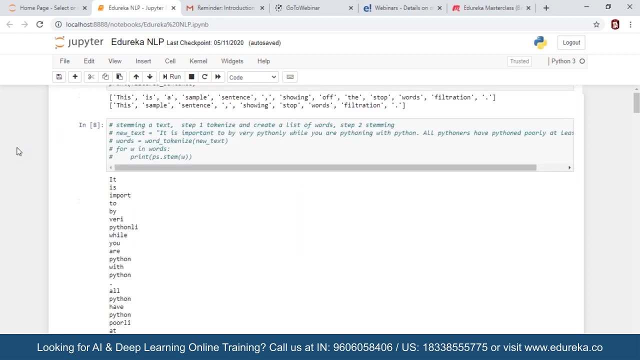 I have a function called world underscore, tokenize and I give the text. So if I write work underscore, tokenize- example text, can you see that it broke the sentence into individual words. So, guys, this is how we do the tokenize things, and let me show you how to do the lemmatization. 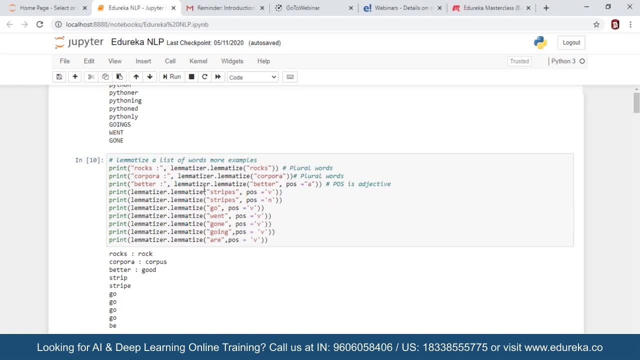 thing, and how lemmatization is better than stemming. So can you see this, guys, that I have used the function Lemmatizer, dot lemmatize, and the word I have used is rocks. So when I use this thing, the word which God has an output is rock, and that is absolutely. 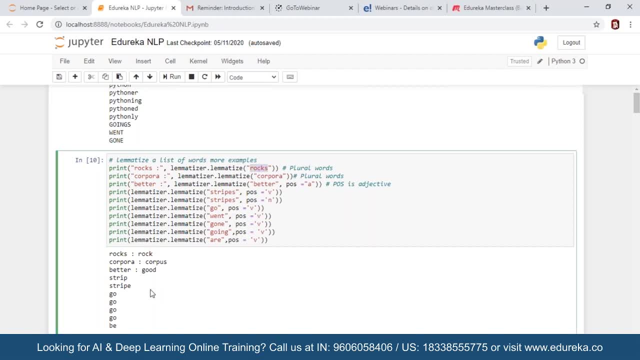 fine, Why? because I use the plural plural word and I got the singular format of that. Same way, I used corpora word and I got the singular format: corpus. Now, if you can see, here, guys, I use four different words: go, went, gone, going, right, and I just 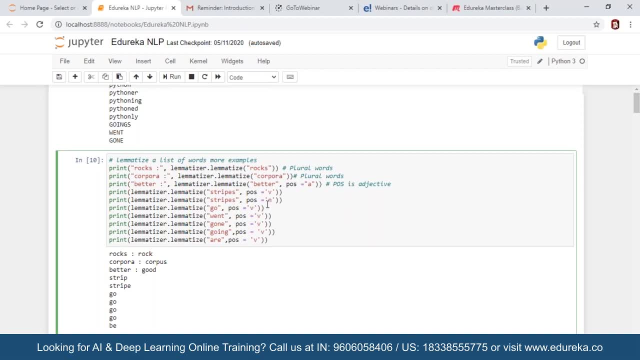 mentioned POS. Now, what is POS? POS is part of speech. V means work. So I just told the lemmatizer that this is a type of work And when I did this, the lemmatizer understood that, okay, the vent is the verb and I need 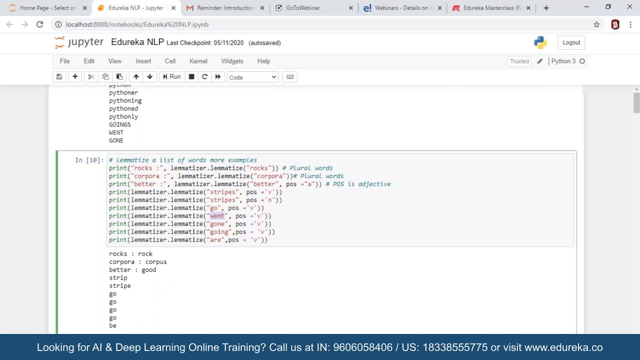 to go to the root word, and the root word for vent is go. if can see here that go, went, gone. all the words got converted to the original word goes. So, guys, This is the benefit of lemmatizer, that you can go to the original word in a better manner. 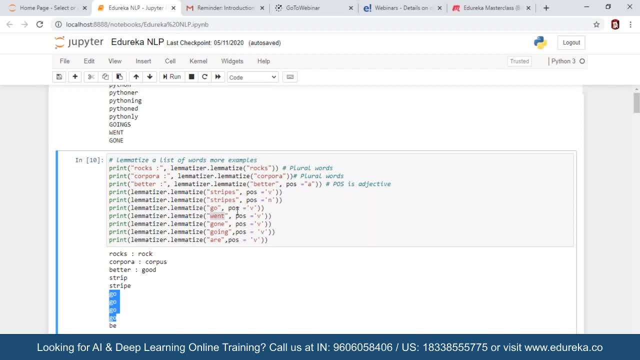 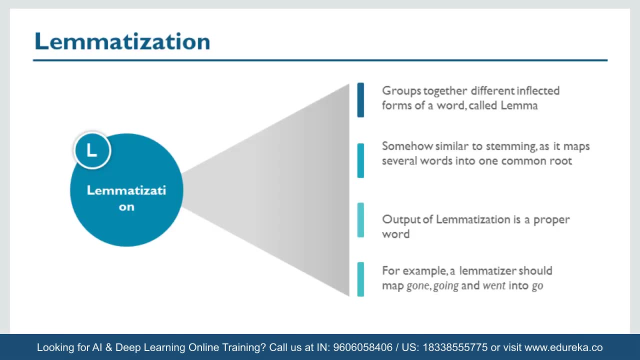 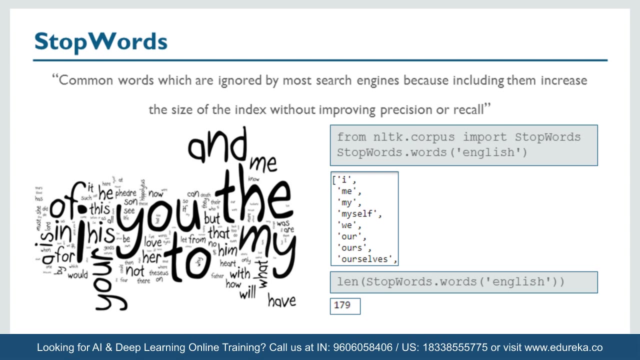 which stemming cannot do, and this is very easy to do: You just have to use the function lemmatizer dot lemmatize. This was another technique which we generally you use, and this is better than stemming. There is another thing which is very important to do, and that is called stop words. 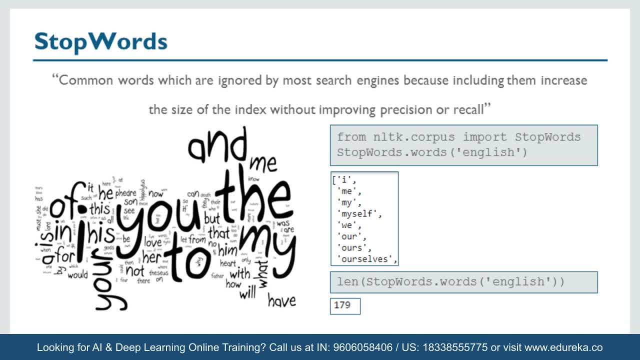 Now, what are stop words? So, guys, if you write and if you see, and if you study the text, data, or maybe a story or maybe a speech, you would see that the most frequent words are like I, me, my myself, be our, our, ourselves is our. 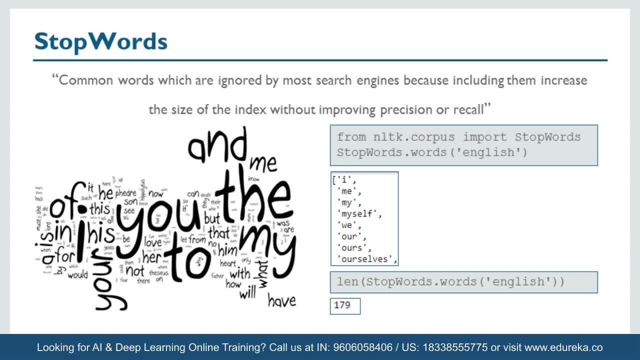 and all those. so these type of words are very frequent, but these does not add any value to your data. This does not mean anything. the words which mean are different. for example, if I am doing the sentiment analysis for BJP, So the words which will be meaningful for me is: disaster is awesome. 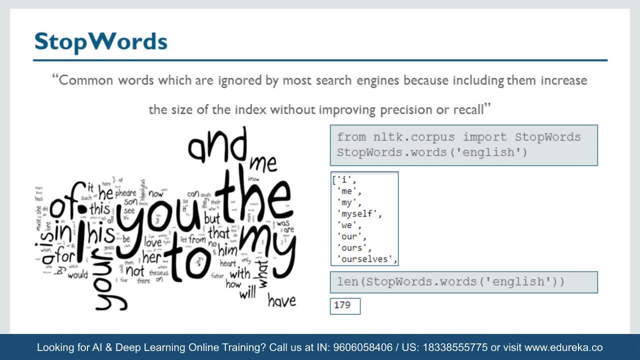 Is basically good work, right? So this kind of work would be there, or maybe economic reformation, rather than I, me myself. So what happens is any analysis which you do on text data. There is a good practice that you should remove these stop words. 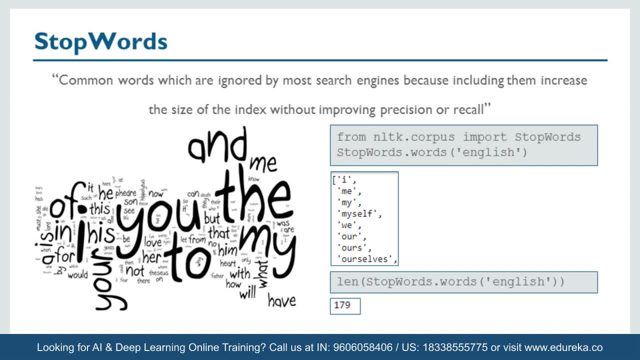 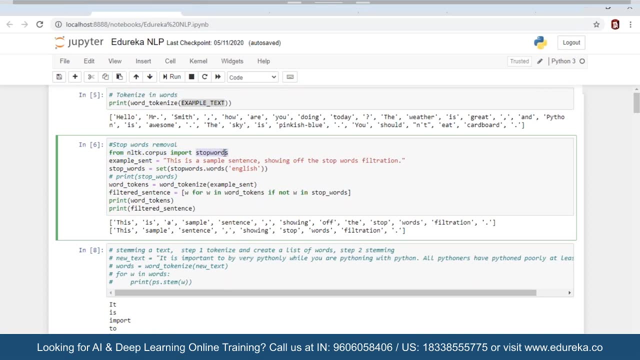 and removing the stop words using NLTK guys is very, very easy. You can do it in just Two, three lines. Let me again show you the code for that. If you see here I imported the stop words here From NLTK dot corpus. 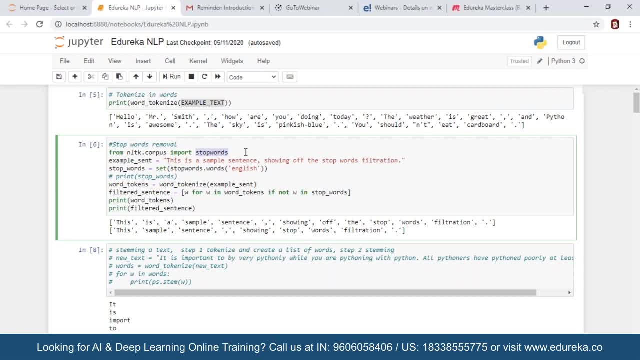 Now, what is stop words? Top words basically contains all the list of stop words into itself, like I, me myself, everything. Now, if you see here, I first created an example sentence here. The example sentence is: This is a sample showing off the stop word filtration. 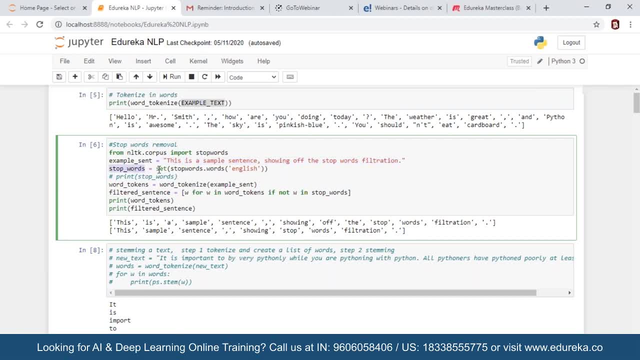 Now what I did is, guys, I created an object- stop words- where I took English stop words. now, stop words is an object which contains lot of different languages stop words if you write French, so it will basically show you or use the stop words used in French language. 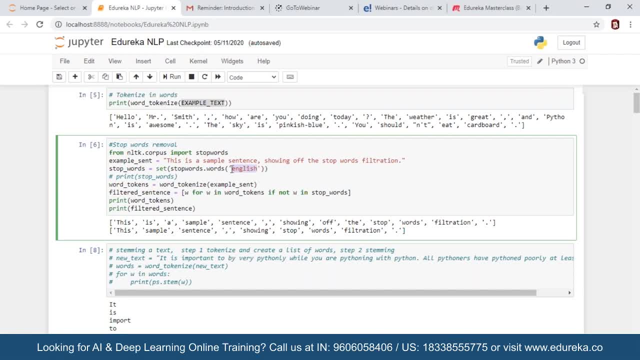 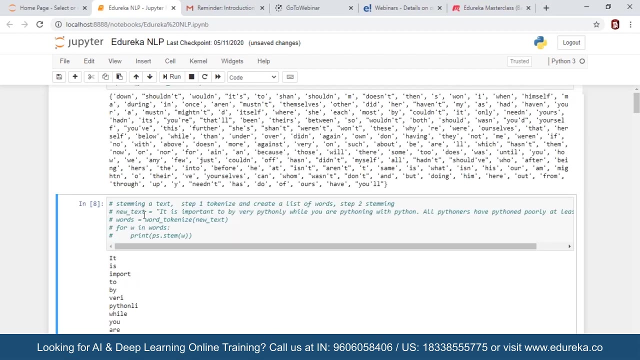 but because the text was English, so I called the English stop words here and let me show You, if you want to see whether, what are the? how does the stopwatch works? So I'll show you. how does this stop what look like? Okay, so, guys, can you see this? 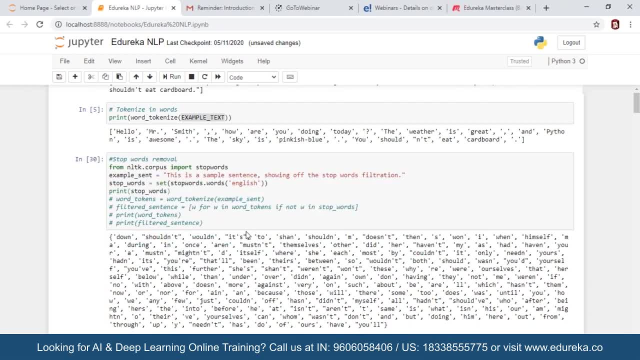 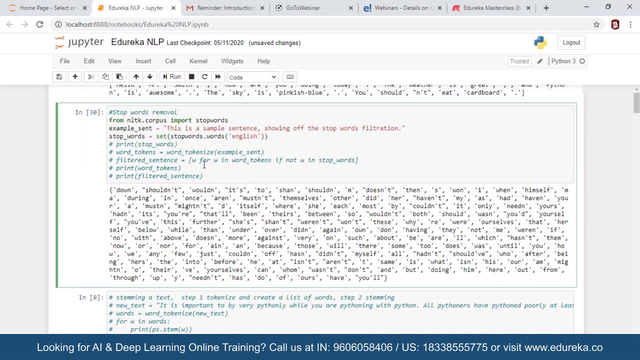 These are the list of stop words down. shouldn't, wouldn't, it's to Shan, shouldn't between theirs. So these are the list of a stop what work, guys, which is available in NLTK for English language. So what it will do, guys, is it will search for. 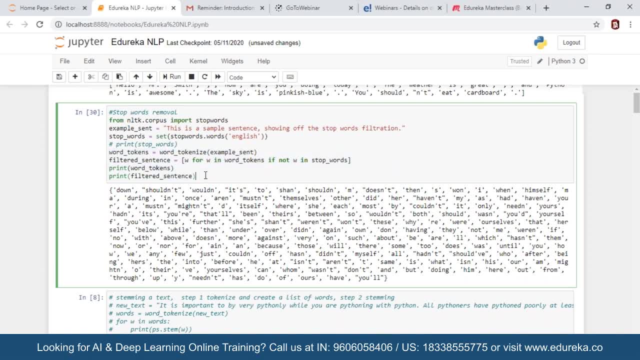 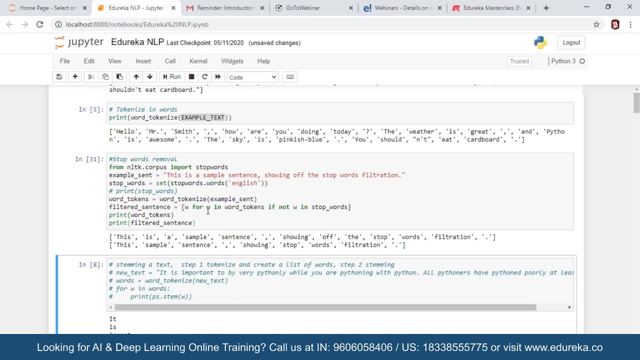 These words in your text data and wherever it is present, it will remove it. So if you see here what I did is I filter those words W for W in words, if not in the stop words. So what I did is I find, for all the words which are not present in the stop words, 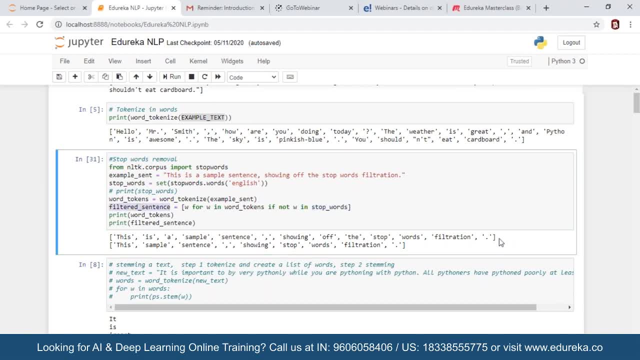 and I stored them into a python is. so see here, guys. This was your original word. It contained some stop words like is a, of, and all those words now here below. This is the list which does not contain the stop words. The stop words has been removed now. 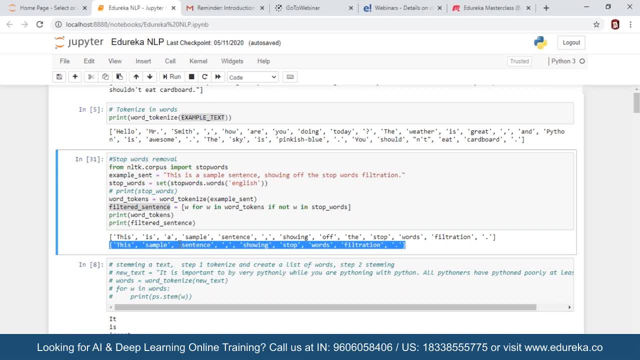 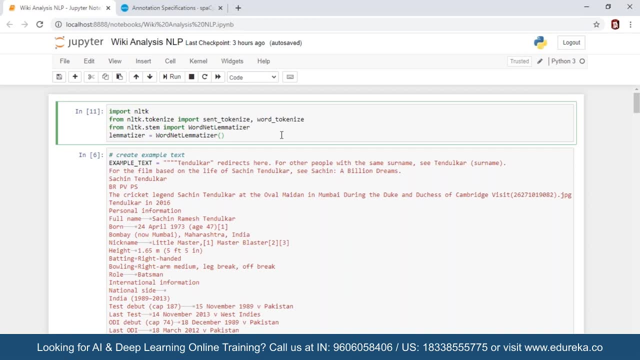 This list is a better source which you can take for your analysis. So, guys, this is like a lot of techniques which I wanted to work with you now. Also, there is something which I wanted to show you end-to-end, because you will. you will think that okay. 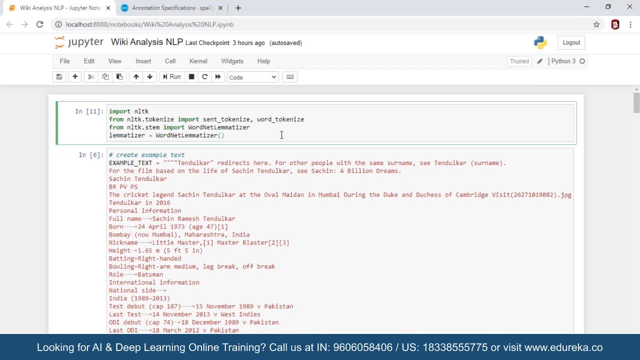 why we are doing tokenizing, Why we are doing, Why we are doing stop words, Why we are doing sentence tokenizer. What is the aim, What is the last thing which you want to do? So for that reason, I have taken a very small end-to-end thing. 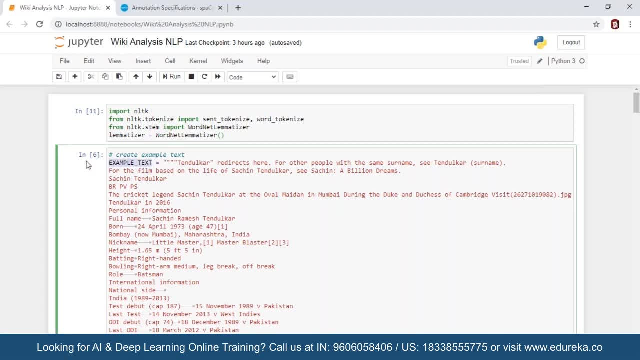 So here what I did, guys: I created an example text and within the text, I took the data which has been written for Sachin Tendulkar Wikipedia. So, if you can see, this is the Sachin Tendulkar Wikipedia content and I mentioned it into double quotes. 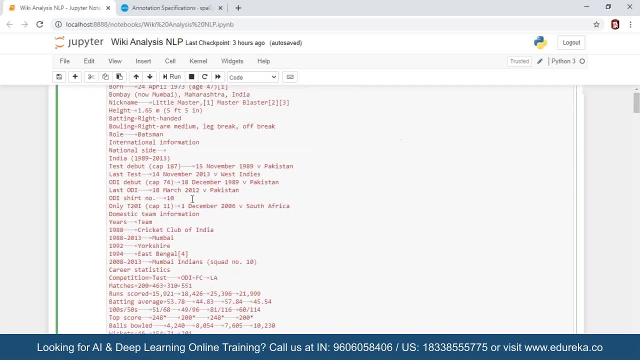 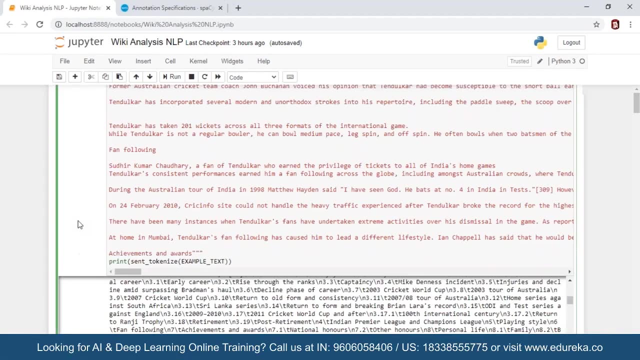 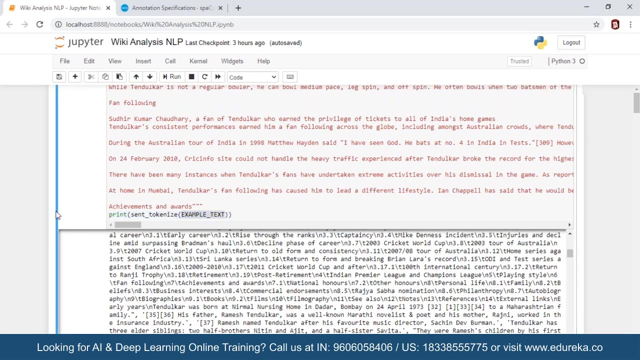 So, basically, this is the data I am going to analyze. so this is a very long data, guys. I have taken intentionally just to show you that, what we can do with NLTK, and after that I basically printed this text data. always remember that the data which I have taken is called example text. now, 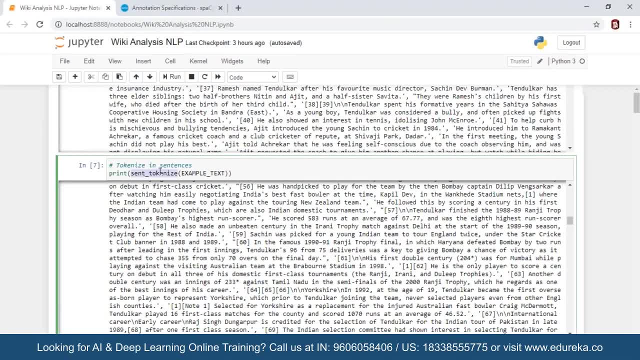 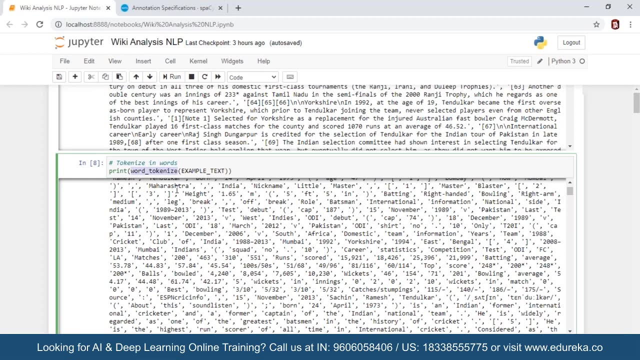 in the next step. guys, What I did is I use sentence tokenizer to sentence tokenizer. What it will do: it will break all the data on the text into sentences. Next, what I did: I use the word tokenizer. So what it will do: It will tokenize all the data into words. 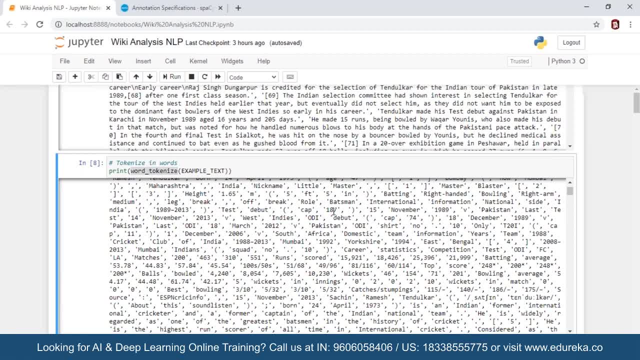 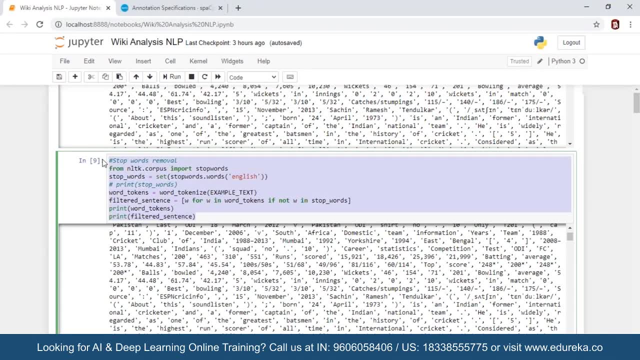 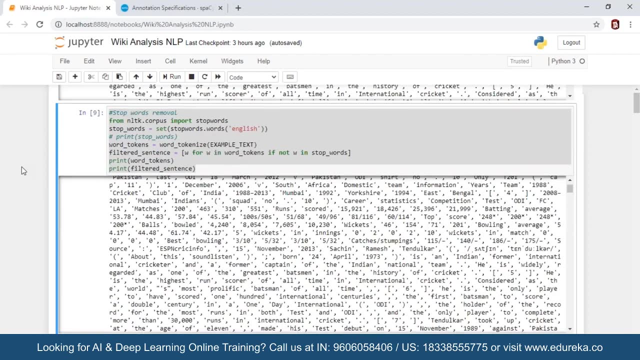 So can you see here each word? we have all the words here. Now, guys, what it did is, as I showed you, that we need to remove the stop words. So I remove the stop words because stop words are not an necessary for my analysis. So after removing the stop words, guys, 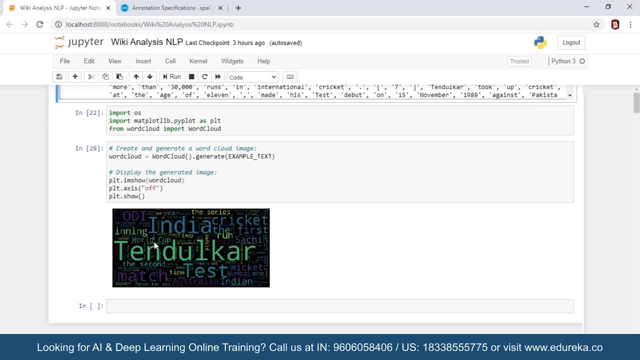 I created a word cloud. So what is a word cloud? word cloud is a representation of world. All the words in your data will be represented and the word which is getting the higher font. Can you see? the Tendulkar award, the India world, the ODI world. 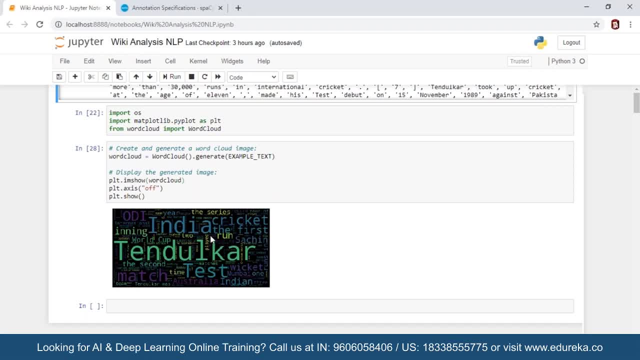 is having the bigger font rather than the cup run player, and all the time. why? because Tendulkar has is more frequent in the text. the frequency of the word Tendulkar is more in the data and the frequency of the word India is more in the data. 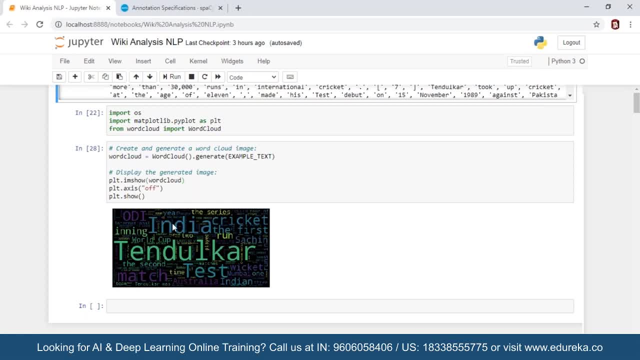 The frequency of the word ODI is more in the retires compared to the series here, And this is obvious. guys, if such in Tendulkar Wikipedia page, if you go and study, if you want go through it, then look at what will be used more of it. 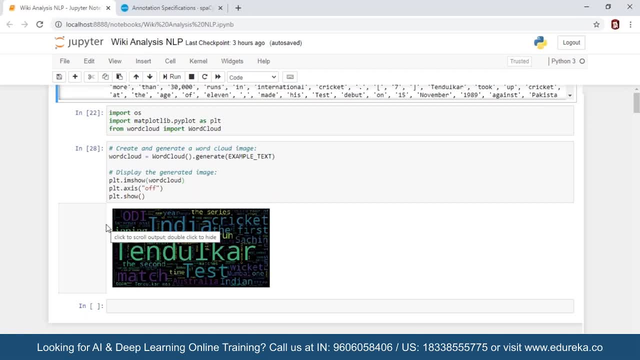 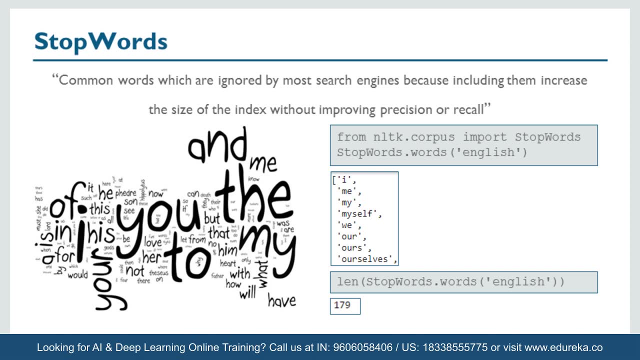 So, guys, this is the example which I wanted to show you that what we can do. What is the word cloud? word clouds is basically nothing but a cloud of words where the most frequent words will get higher font size, So all the present words in your text data main words will come there. 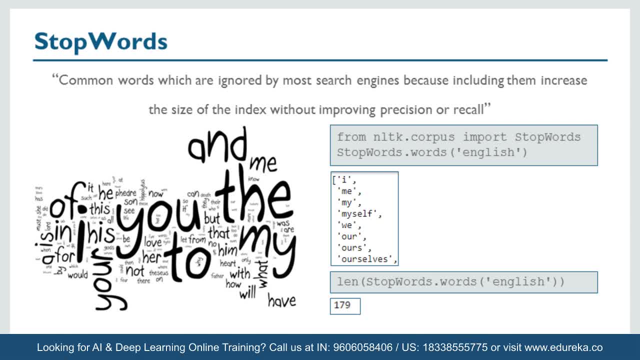 and the most frequent word, We'll get a higher font and the lesser frequent word will get a lower font. Does an LP data scientists need to know language to work on it? No, this is not required that you need to know the language, but generally we need to work on English. 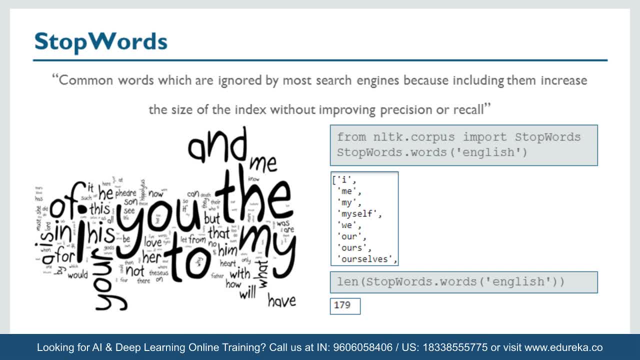 But if you know, if you are familiar with the language, that is fine, That will be an advantage. advantage. But even if you don't know the language, you can do the basic NLP principles and you can come up with a good analysis. What are the differences between deep learning and LP? 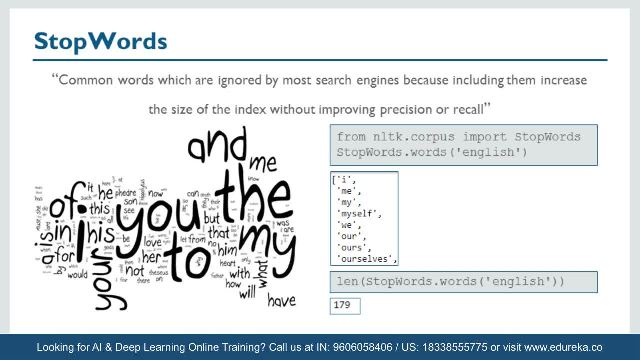 So deep learning is a different domain, NLP is a different domain and LP is the particular domain where you take the text, data, You process it. deep learning It's something which is related to neural network. You can use neural network and deep learning to solve NLP problems. 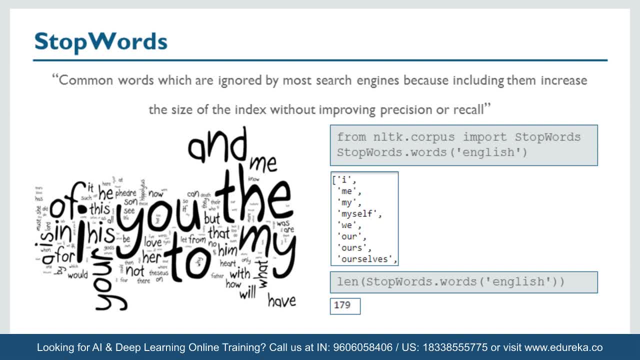 These both are different, but these both are helpful. These two are different things which you can learn and with a combination of these two things, you can solve a lot of the problems. So how does a chatbot understand the sense of word? So, guys, chatbot basically reads questions. 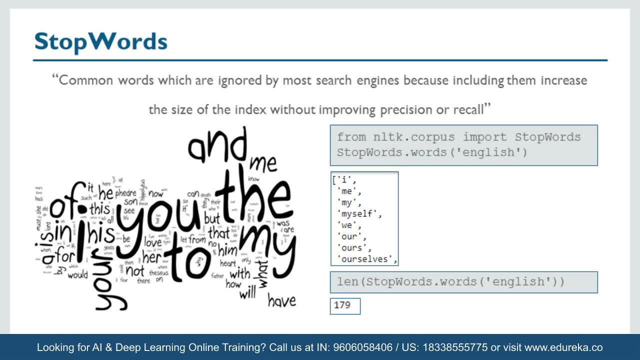 So you train a chatbot on on question and answer. So maybe if I give him a 1 million question and answer like chats of the two friends, but one friend will write questions and one will and will answer it. So we train it on question and answer and we train it.